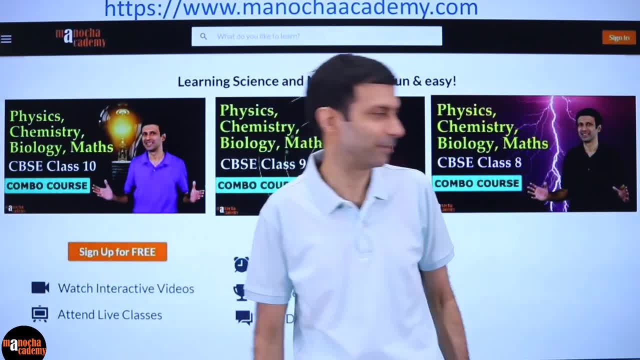 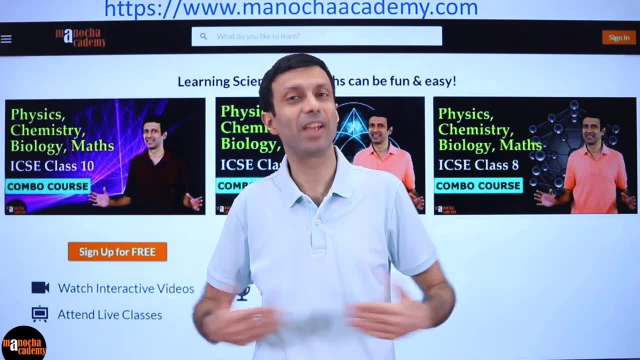 taken the other courses. do take them and do share it with your friends. for the ICSE students, we have physics, chemistry, biology and maths courses. for classes 8, 9 and 10, once again, do share out our courses with your friends. you and if you want to learn coding, we have Python programming, we have Java coding. 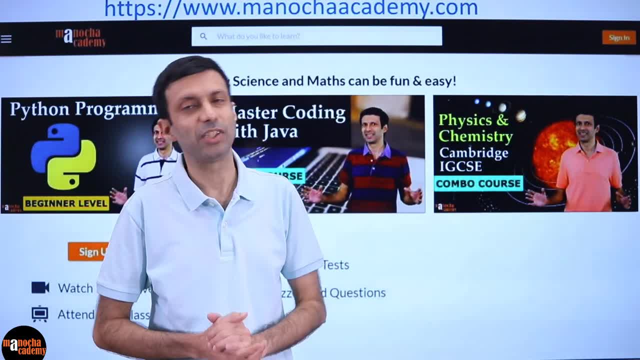 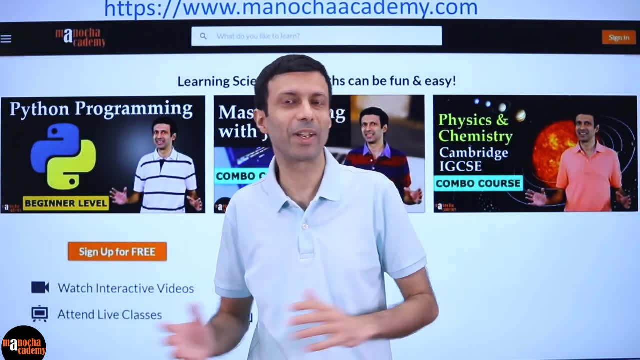 and we have physics and chemistry for the Cambridge IGCSE, which is the International Board. so please do share our courses with your friends. make sure you have subscribed to our YouTube channel. you can also follow us on Facebook and Instagram, so stay connected with Manocha Academy and keep learning. 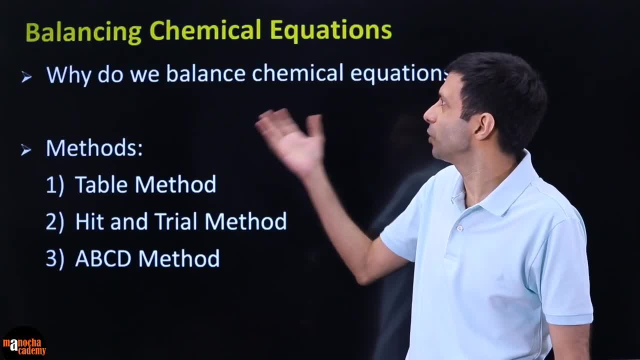 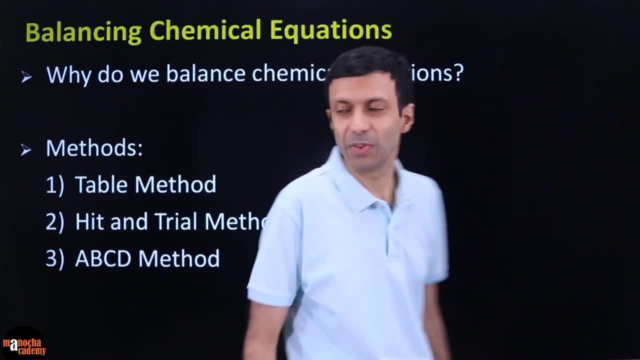 so when we are talking about balancing equations, the first question is: why do we balance chemical equations? so we are going to look at that and then the goal for this class is: we are going to see the different methods. we're going to be learning the table method, the hit and 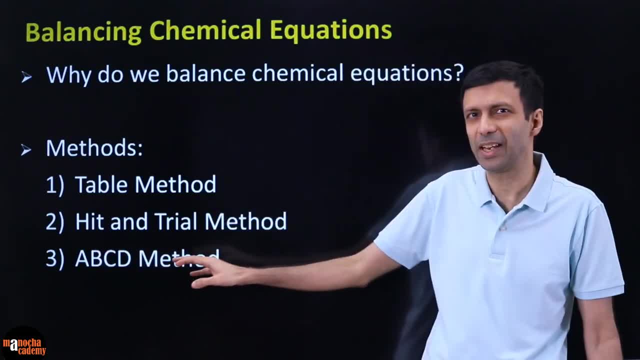 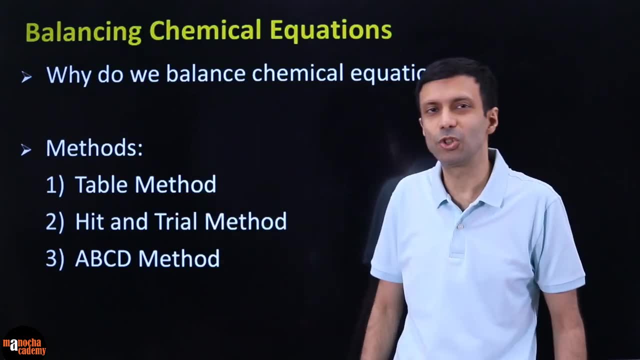 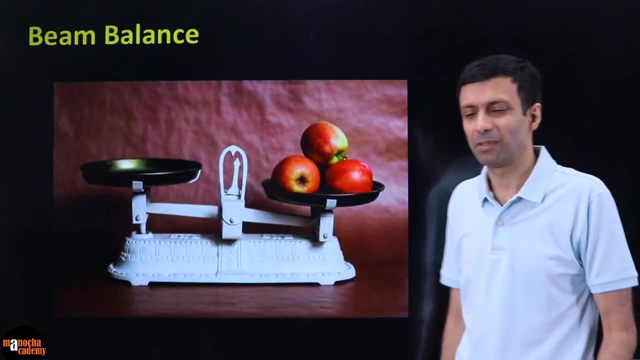 trial method and this wonderful ABCD method, which can help us solve even difficult equations that we are not able to balance. so I'm going to try to cover all these methods in today's class and make it really easy for you. so let's get started. so I'm sure all of you have seen this beam balance like if you go for 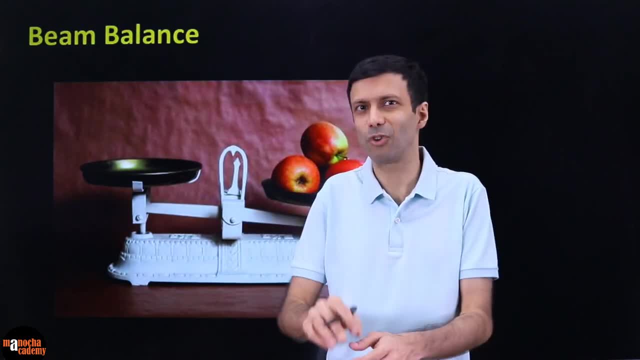 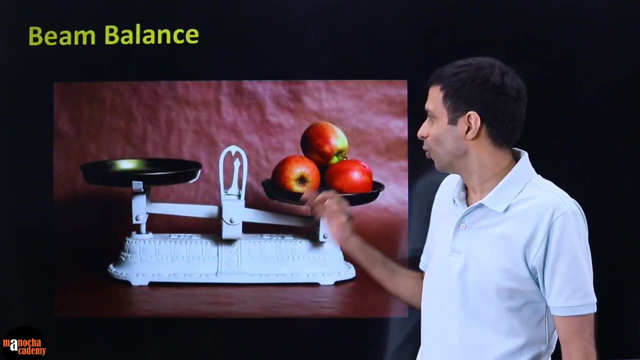 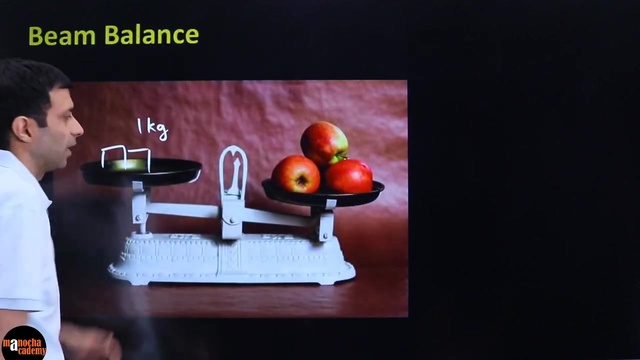 vegetable shopping. of course, nowadays, you know, they're replaced with this electronic balance where they just gives us the weight. but this is that traditional beam balance, or we call it as Tarazo in Hindi. so where, if you place the you know apples over here, and let's say we play some masses over here, and let's say 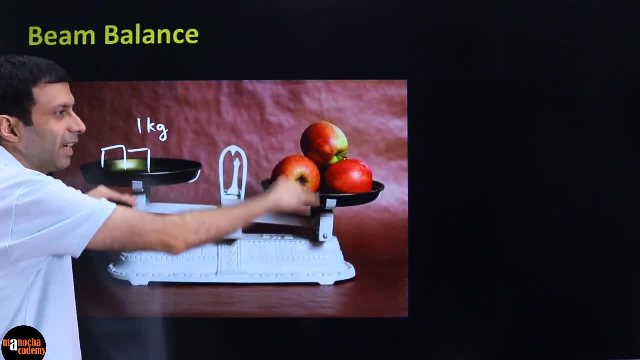 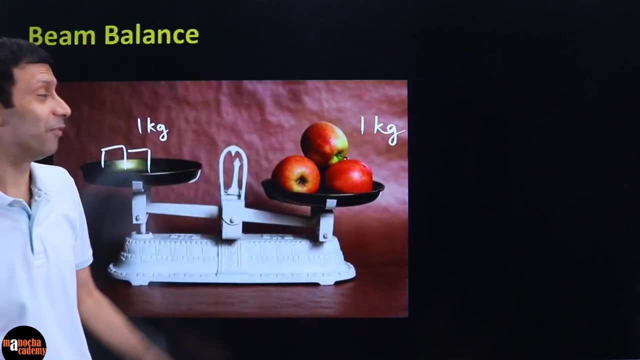 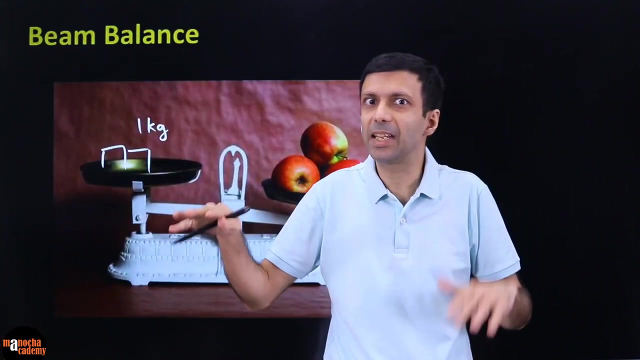 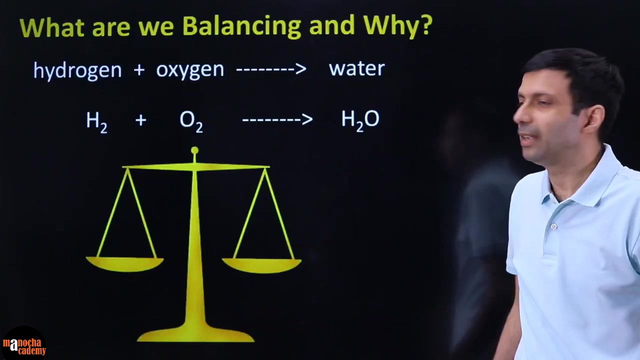 when we put these 1 kg weights or masses, we see that it gets balanced. so then, what is the weight of these apples? or, correctly speaking physics, the mass of these apples is 1 kg, because it is now balanced. similarly, we are going to be balancing what is in chemical equations or the number of atoms. so, for example, let's: 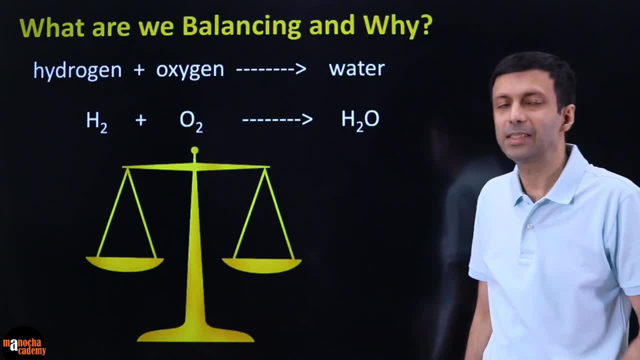 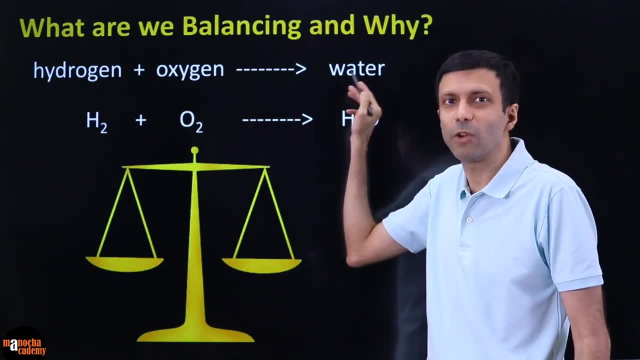 discuss this balancing. let's really understand what are we trying to balance and why so. this is the famous equation all of you have seen: hydrogen plus oxygen is water, and this we call the world equation because we have written it in simple words, but really we are chemistry guys, so we want to translate. 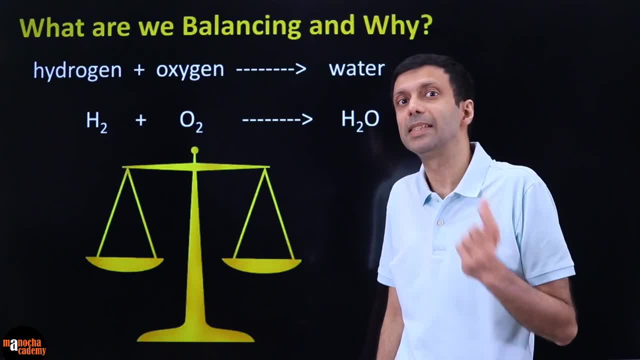 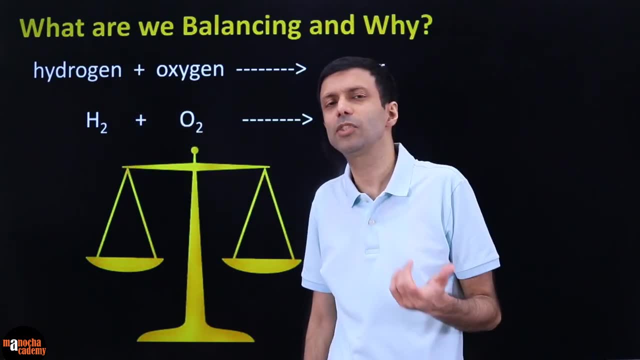 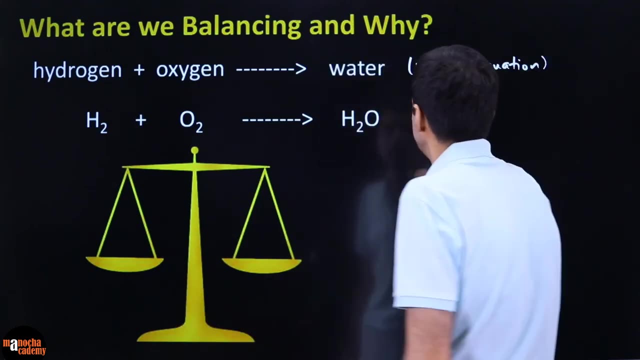 it into a chemical equation by changing all the words into symbols. now, how do we do that? Hydrogen, Why have I written H2?? Why have I not just written H? Because, remember, this thing is a world equation And we are changing it into a chemical equation here. 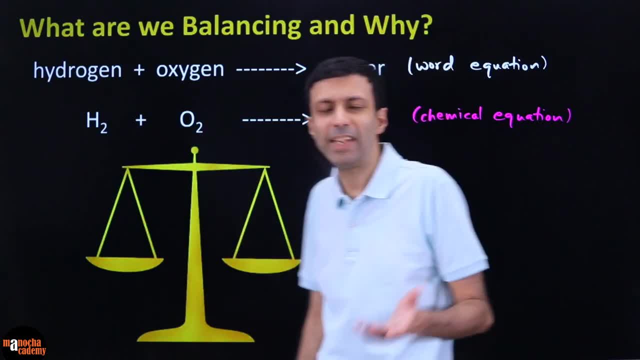 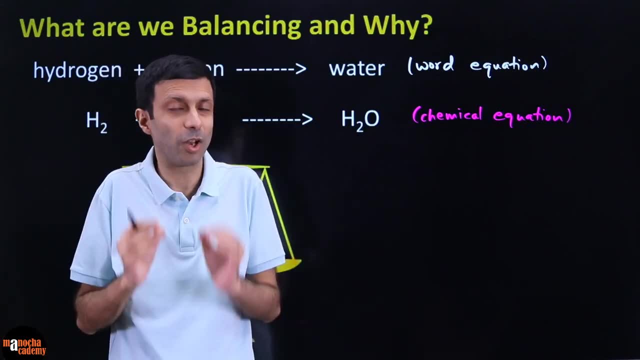 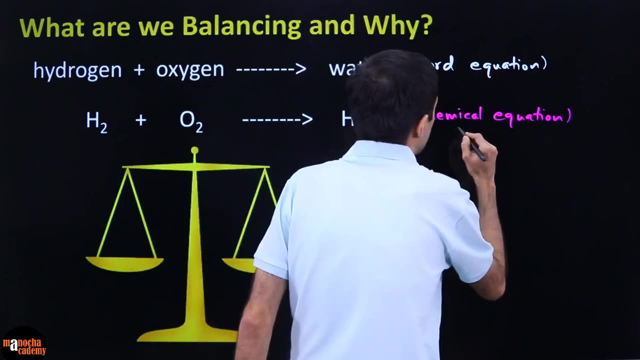 But why do we see this? H2, O2?? Why not just simple H and O? Because, remember, the world exists in terms of molecules, or substances exist in terms of molecules. Because molecules can exist independently, right, They are stable. So that is why, remember, chemical equations are written in terms of molecules. 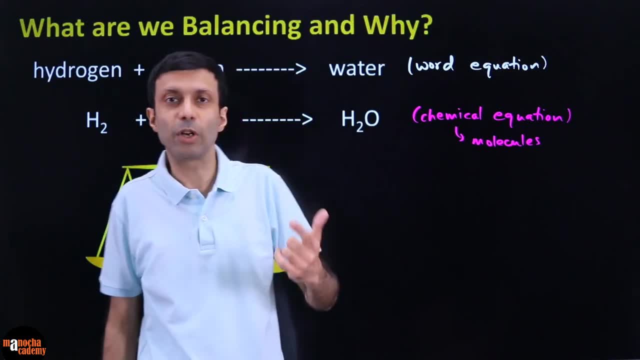 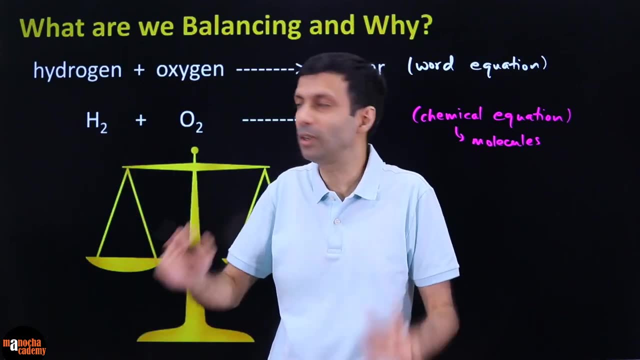 So what is one? molecule of hydrogen- H2, because hydrogen is diatomic gas. If you are just writing the atom of oxygen you would have, of hydrogen, you would have written H, But molecule is H2.. Similarly, molecule of oxygen- O2, containing two atoms of oxygen. 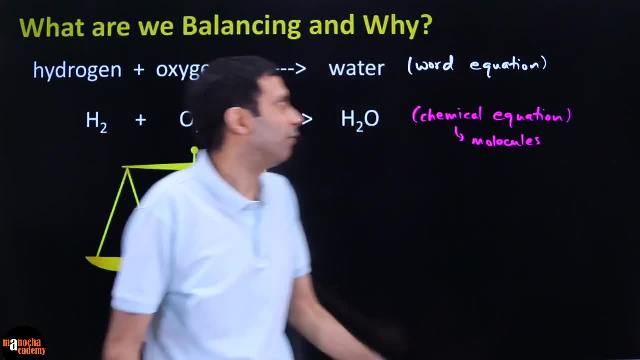 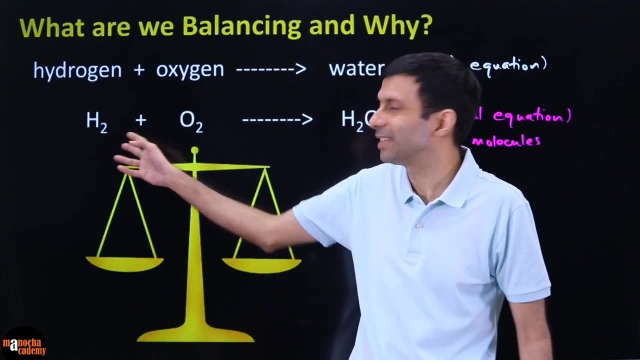 And when they two, when these two react together, they form the compound water: H2O, H2O. So for elements, remember, we use atomicity. These guys are diatomic, These are elements. For molecules, we have to use balancing right. That is why H2O here. 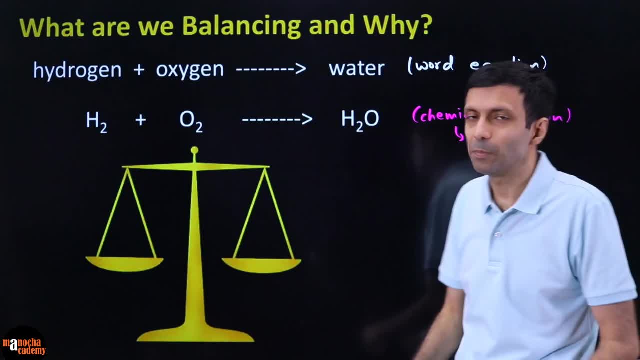 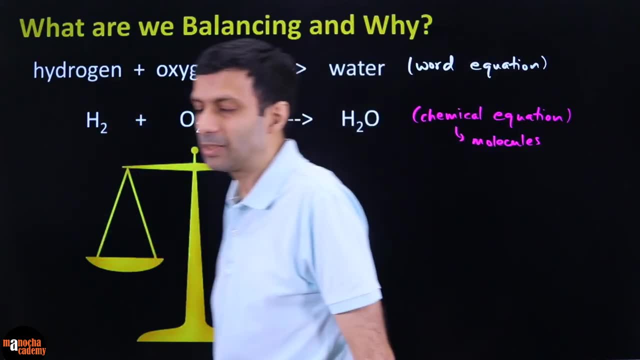 So this is our chemical equation. Now, if we take a look, what does this mean? according to our beam balance? So, if you want to put these, what do we call the guys on the left? as in the chemical equation, These are called as our reactants. 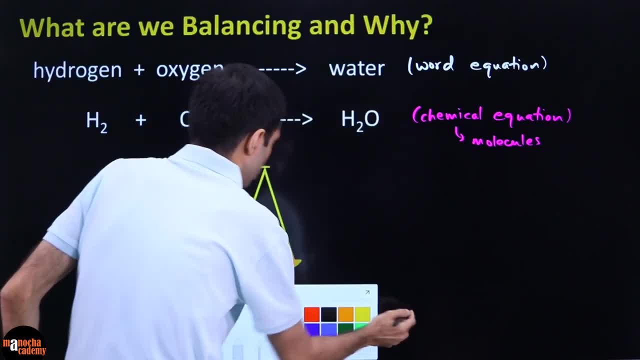 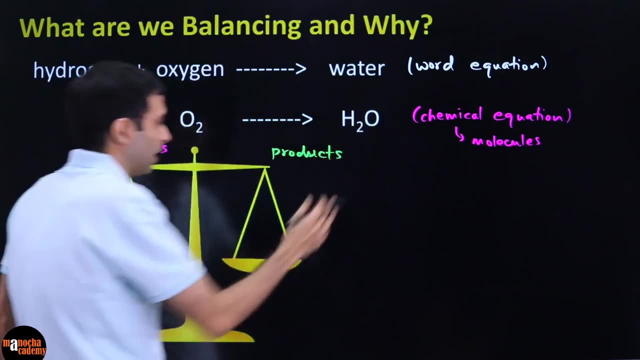 And this side is called the products. So let us see, So, let us see, So let us take these reactants here and put it on the left side of the beam balance, And the products, we will put it on the right side. 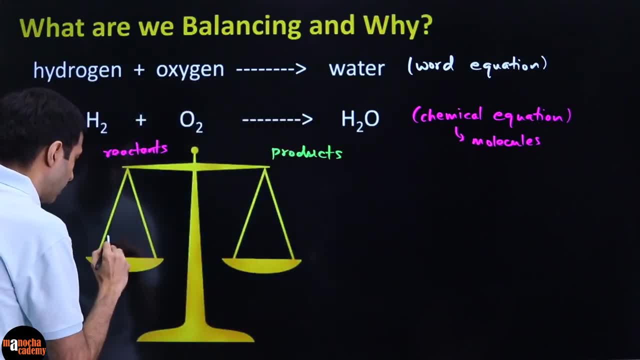 So, for example, if you have got H2 and O2 here And here we have H2O. So, since we have put it on a beam, balance means we are going to try to see if their masses are balancing or not. 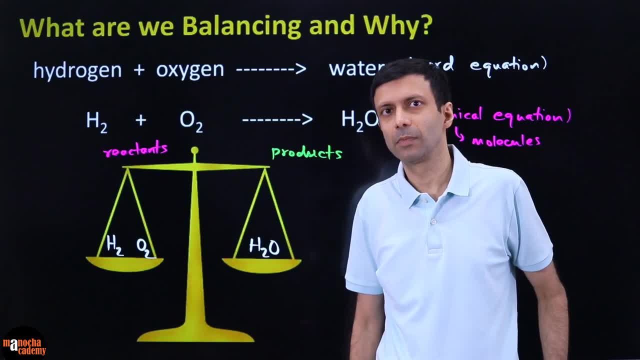 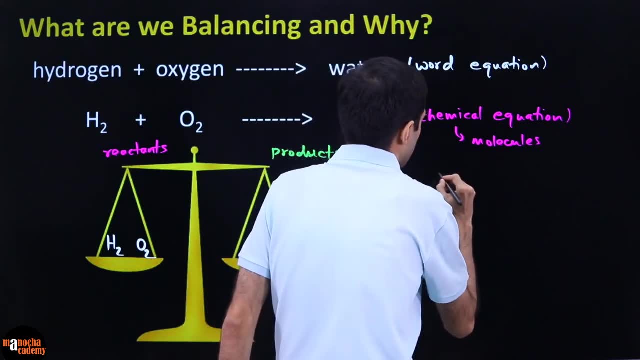 So can you guys tell me what is the mass of H2?? Or let us start with what is the mass of one hydrogen atom? You guys know that Mass of hydrogen atom is 1 amu or 1 u, whichever way you guys write it, right. 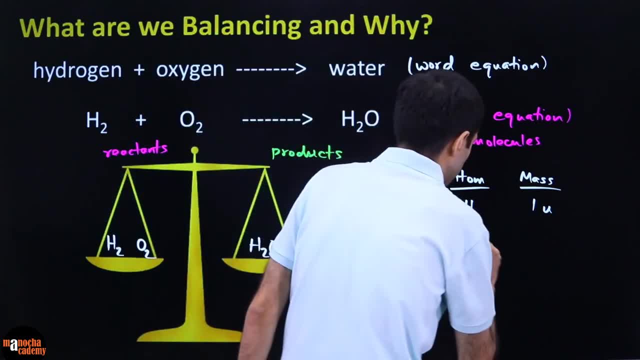 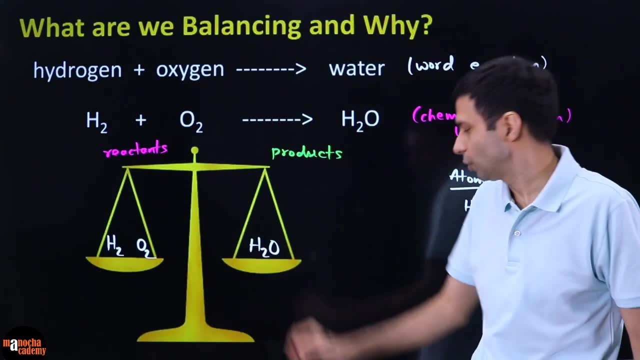 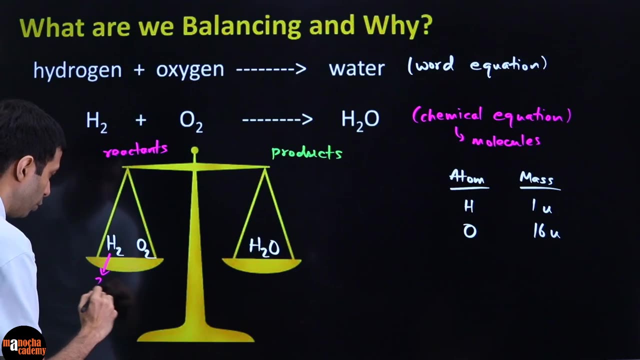 It is the lightest atom. Oxygen is 16 u. So if you work out the numbers, what is the mass of hydrogen over here? Hydrogen is basically 2 times 1.. So this is going to be 2 u plus we have 16 u times 2.. 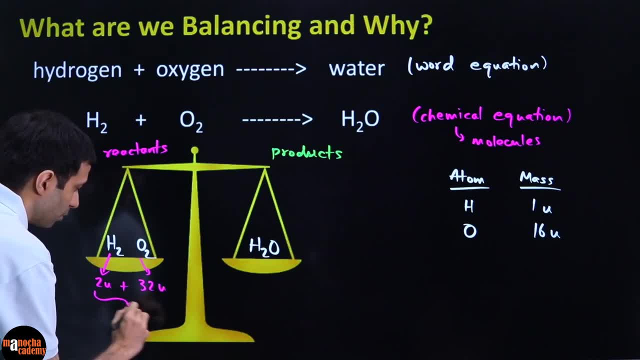 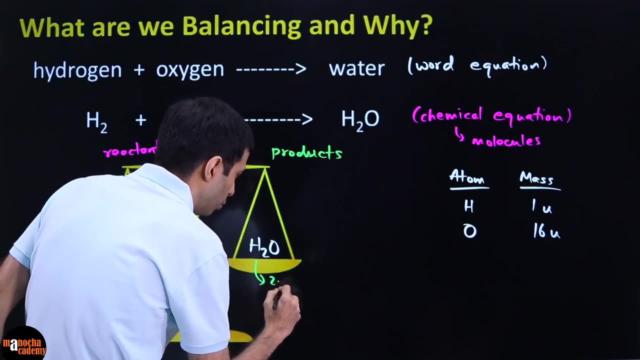 So 32 u. So what is the total here? Total is basically 34 u or 34 amu. You guys agree. What do we have on the product side? Water, Water. what will be the mass? This is going to be 2 u plus 16 u. 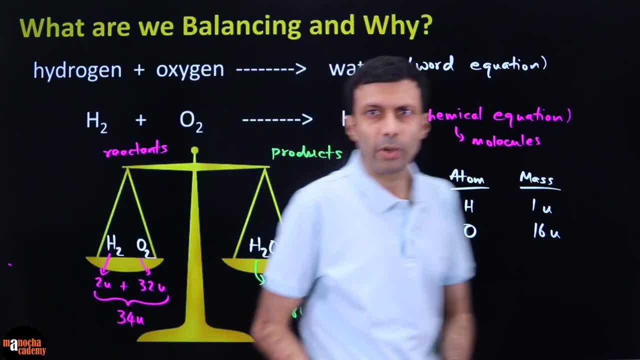 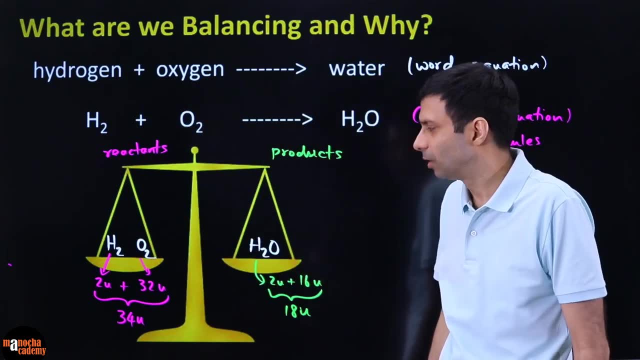 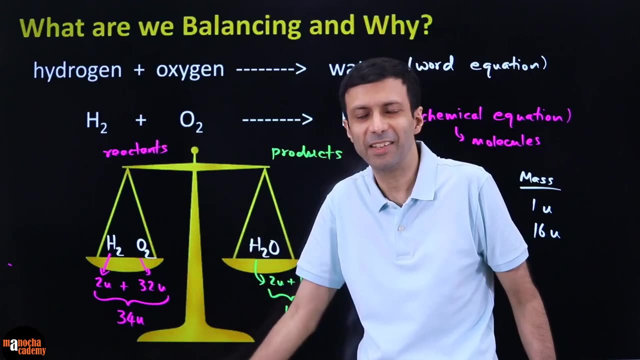 That gives me 18 u. So if we take our The chemical equation, if you wrote And we just put it on our beam balance, Will it balance? You have 34 u here and 18 u here, So definitely it is going to tilt towards the left hand side. 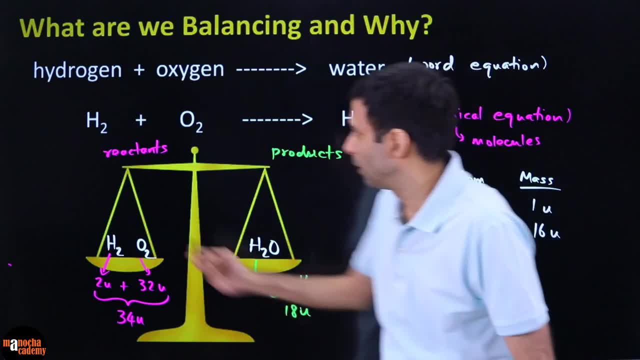 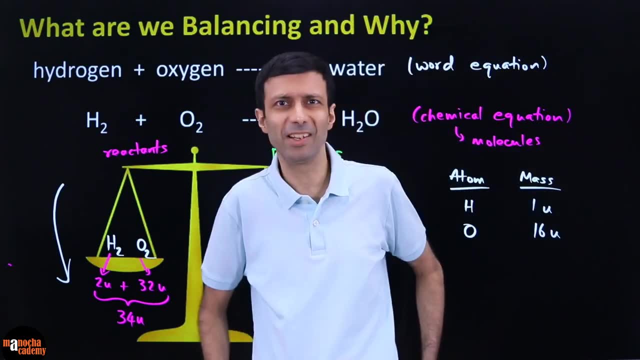 Do you guys agree? So our beam balance is definitely going to swing this way. It is not a balanced equation And in life everybody wants balance. right? You keep hearing this term. lead a balanced life. Everything we want, perfect balance. 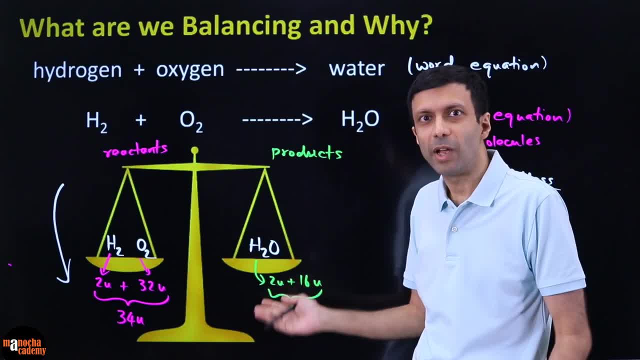 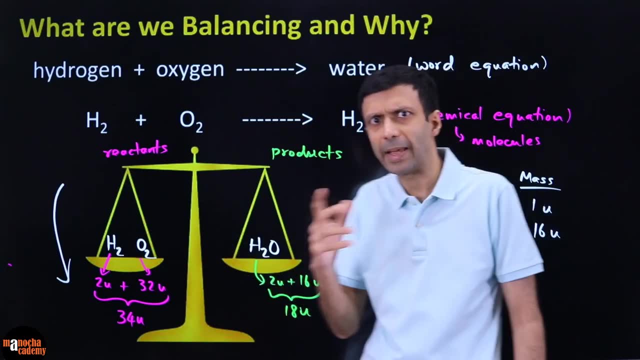 Same here. This is not good. And what is not good here? How can 34 amu become 18 amu? That means there is a loss in mass. Can a loss in mass happen in a chemical reaction? We know there is law of conservation of mass. 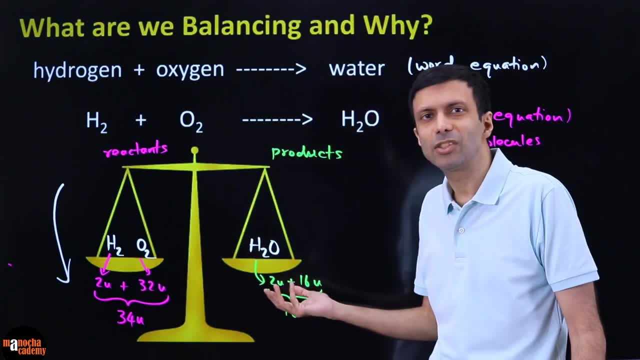 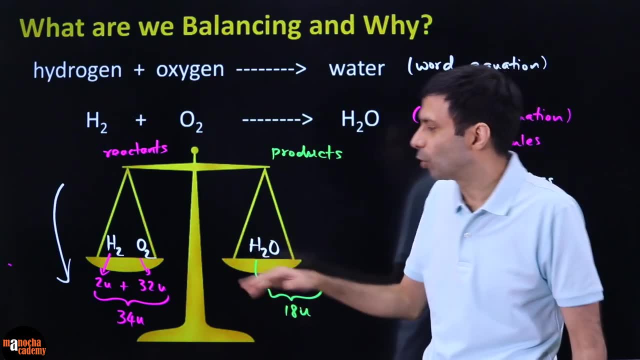 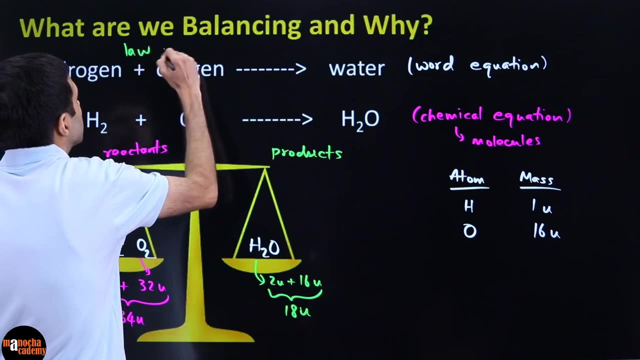 Mass cannot simply appear or disappear. So this is against the law of conservation of mass. So that is what we are trying to satisfy here, That we are trying to balance Because we want to Satisfy The law of conservation of mass. 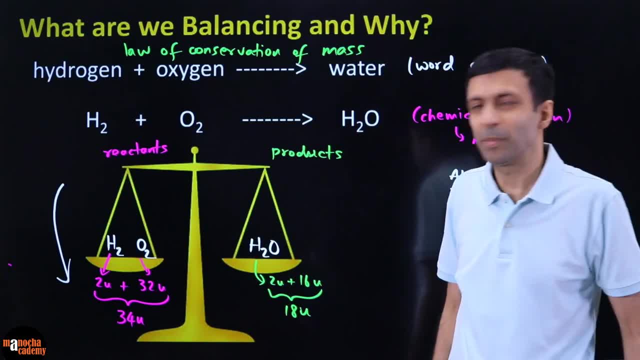 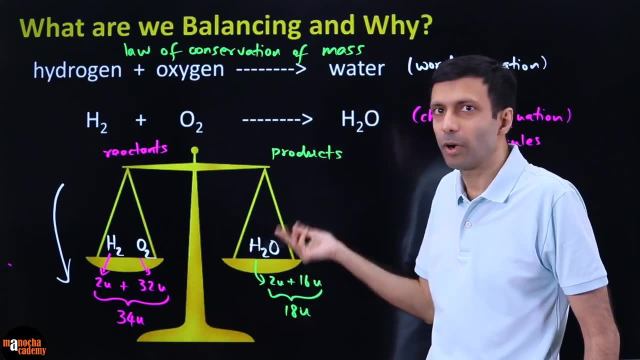 So we will behave like the vegetable guy. We will say, okay, there is more mass there, less here, I am going to put more here. What can I put? I can only put products. I can put hydrogen oxygen here. 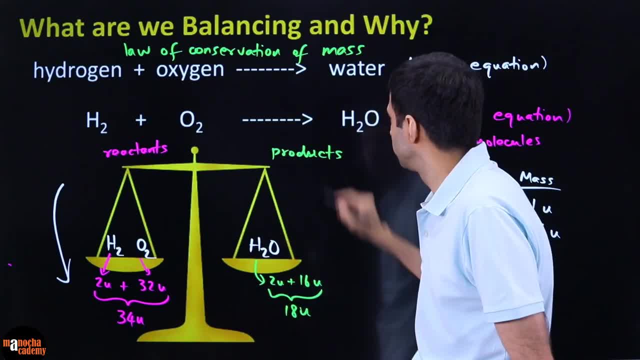 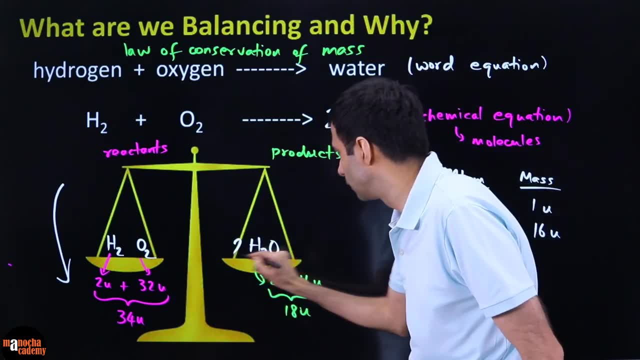 I can only put water. So let us say, if we put 2 water here, So 2 water means it is going to become 2 times 18.. That means if I put 2 water here, This new mass is going to be. 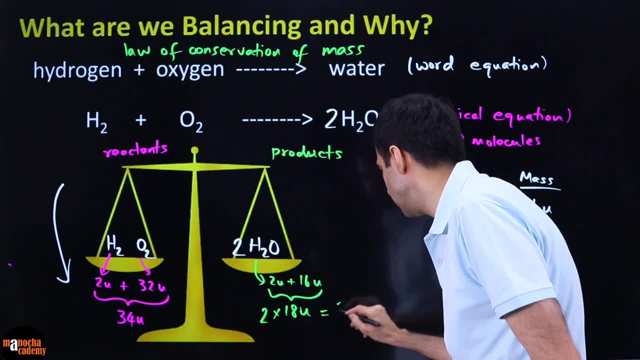 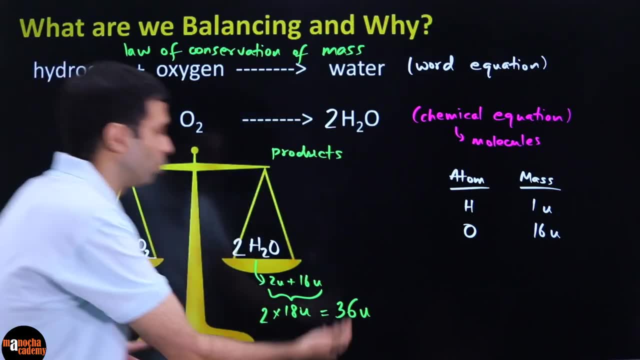 2 times 18.. Which is 36 U. Now we will again be the fruit. The vegetable guy. The fruit guy will say: oh, there is 36 U Too much over here, Only 34 U. So it is still not balanced. 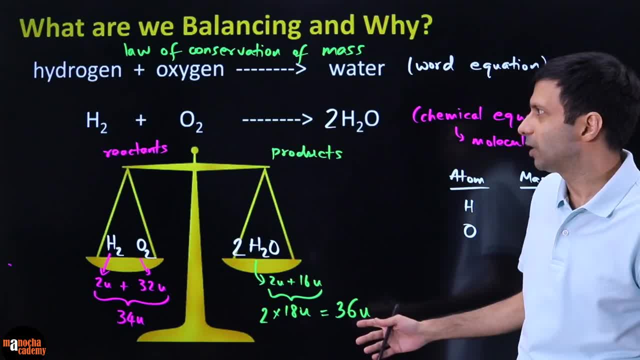 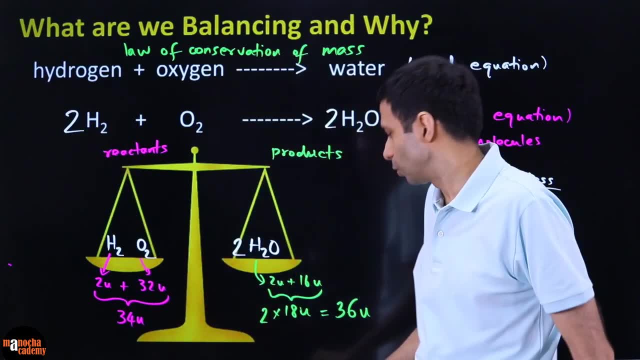 What will we do here? now? It is still not balanced. So we will say: okay, We are a smart vegetable guy, So we will say: to balance it, let us put 2 hydrogen. Because when we put 2 hydrogen, 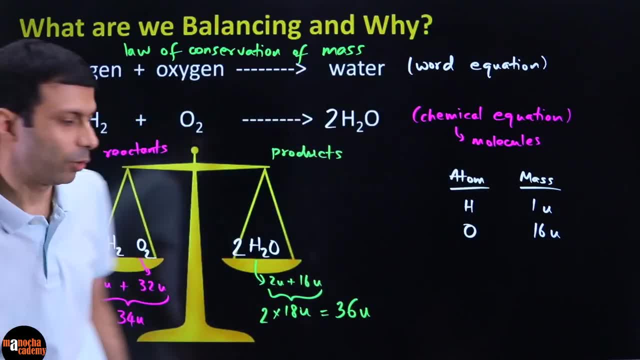 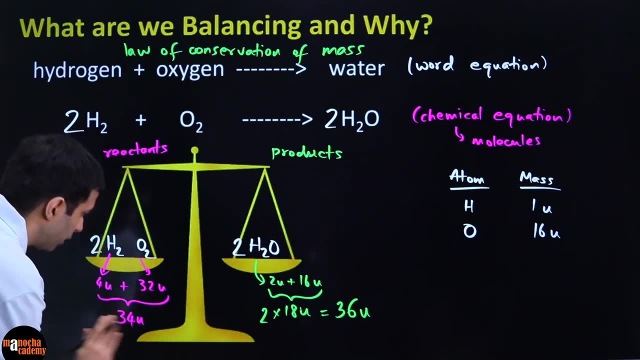 This number is going to change to 4 U, Because 2 times 2 times 1.. So that is 4 U, So 4 U plus 32 U, 36 U. So, like the fruit seller, We are now happy. 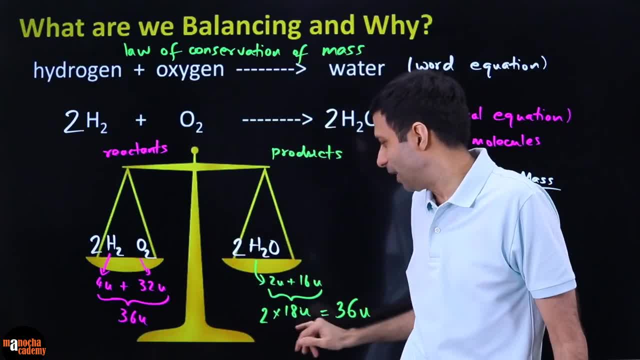 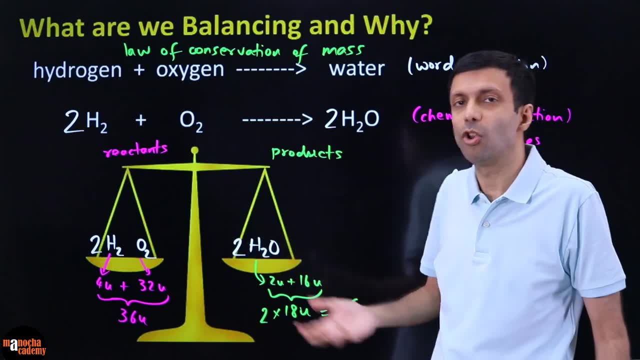 Because our thing is balanced: 36 AMU here, 36 AMU here. So this is the goal Is to balance the mass. The law of conservation of mass must be satisfied. Famous question: Why are we balancing equation To satisfy law of conservation of mass? 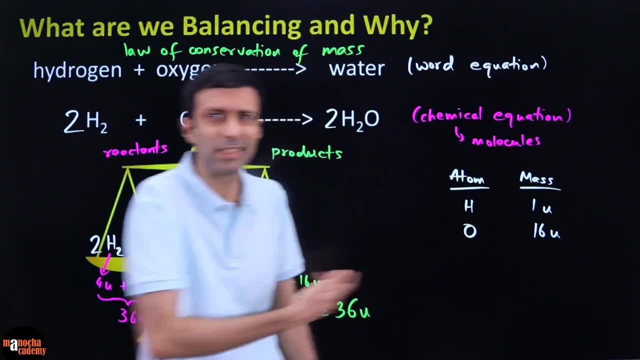 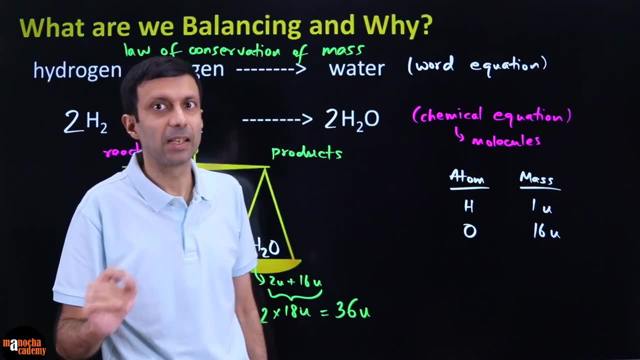 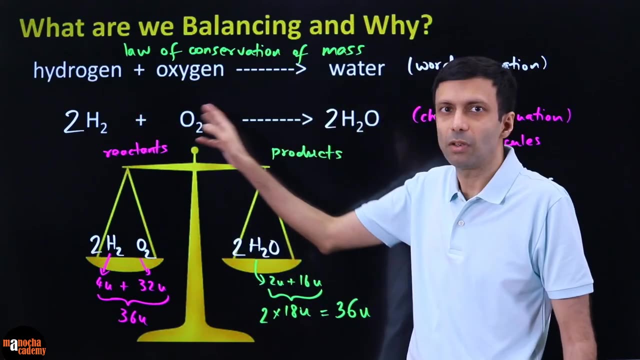 But do we every time need to look at all these masses and do that? The good news is, thankfully, no. So what you really need to balance is the number of atoms of each element, Because, if you carefully notice, Hydrogen is still remaining hydrogen. 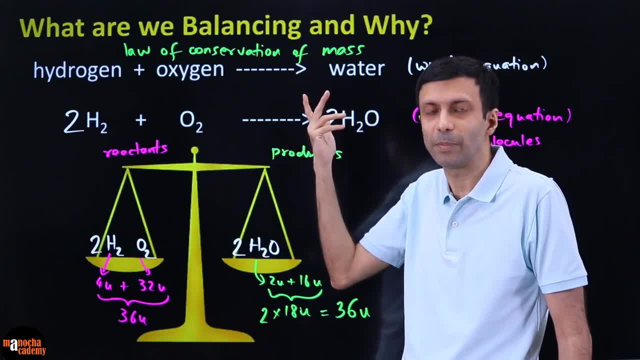 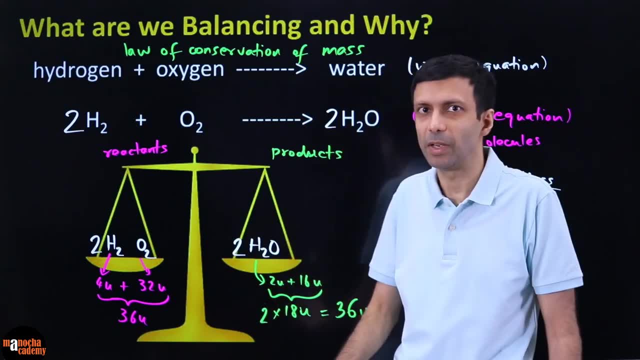 Oxygen is still there in the products. It is not that oxygen has become nitrogen or something else. So instead of balancing masses, We can simply balance the number of atoms of each and every element. So if you look at our final equation here, 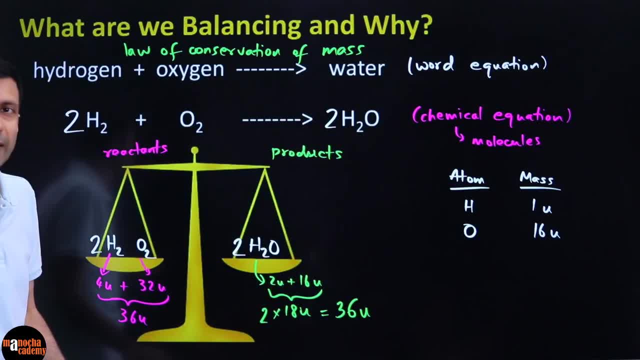 Even though we try to balance mass, What have we ended up doing? How many hydrogen atoms? on the left You can see there is 4 hydrogen atoms here. How many oxygen atoms? 2 oxygen Or 2 O? This is not 20.. 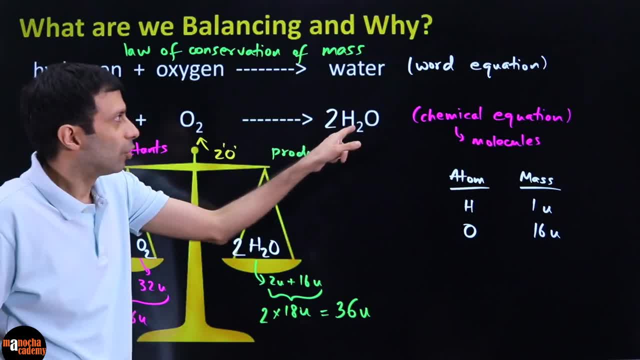 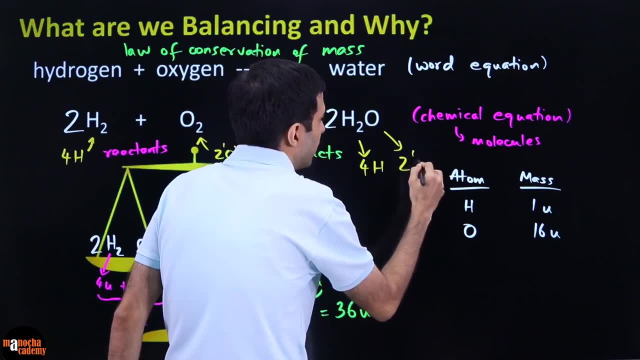 How many do we have in the products? 2 hydrogen atoms in water, But there are 2 molecules of water, So 4 hydrogen atoms, 2 hydrogen here And once again 2 oxygen, because 1 water molecule has 1 oxygen atom multiplied by 2.. 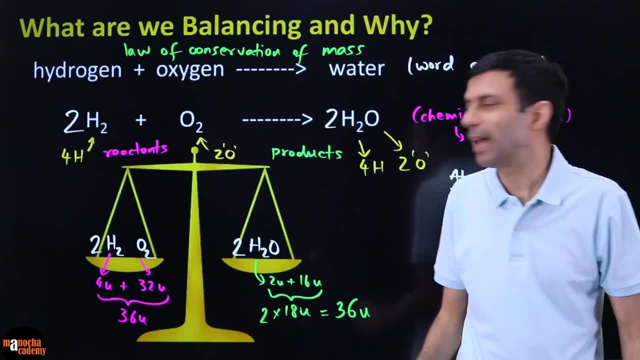 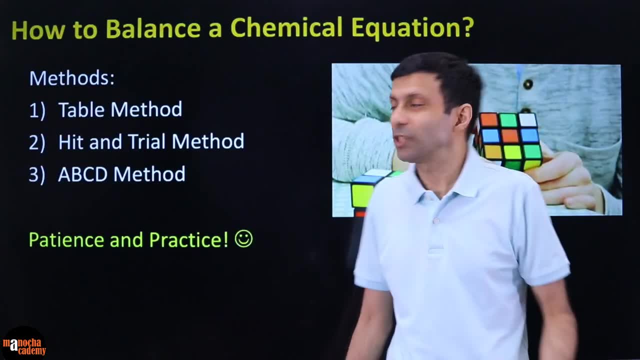 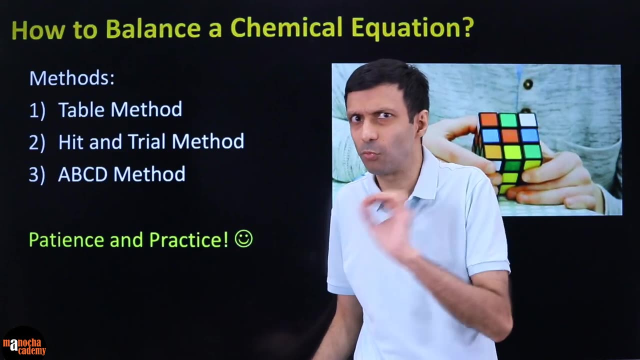 So this is very important, That what we are really balancing Is the number of atoms Of each element. here Now, the important question is: How do we balance a chemical equation Because, as I said, We don't have to do a mass every time. 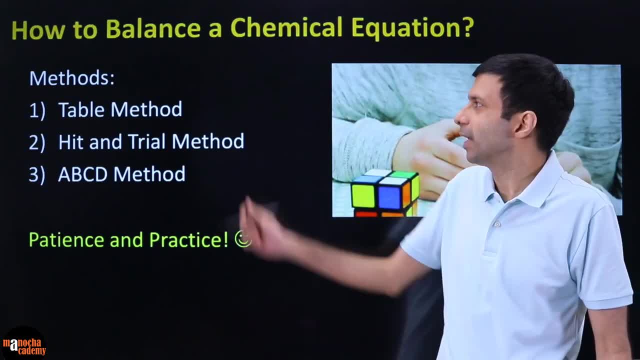 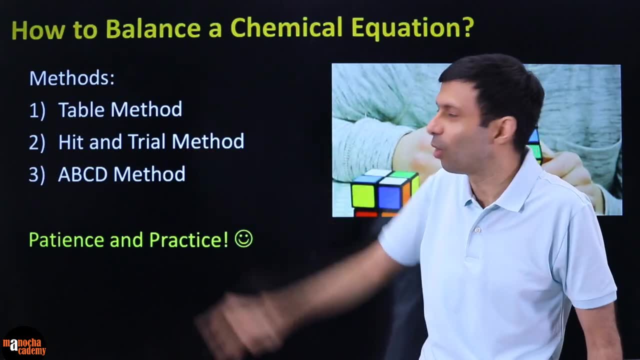 We just have to focus on the number of atoms of each element. So there are many methods. There is basic table method, Then there is hidden trial, Then there is the ABCD- Powerful ABCD- method, And I am going to go through all of these in today's class. 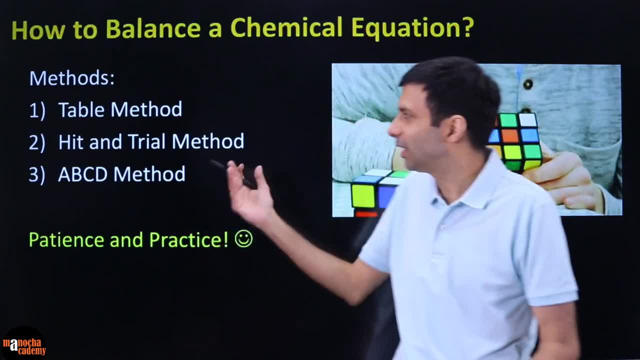 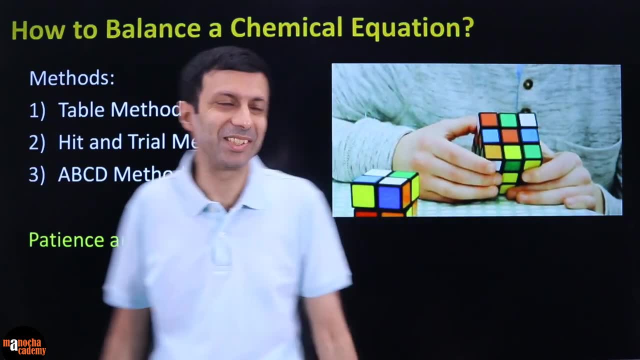 And we will see which one we should use. What is the recommendation here? Of course, yours might be different, But let's see what is the best way we can do, Because we want to solve it quick and accurately. And, of course, balancing chemical equations is like. 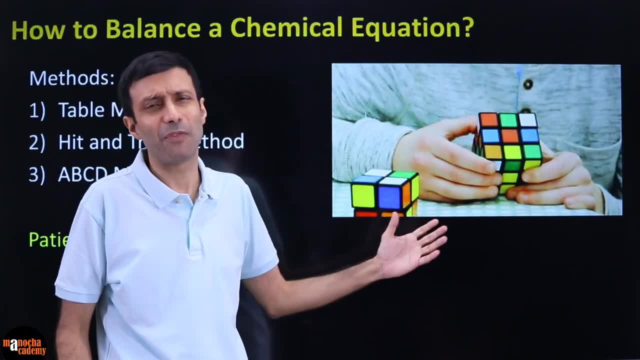 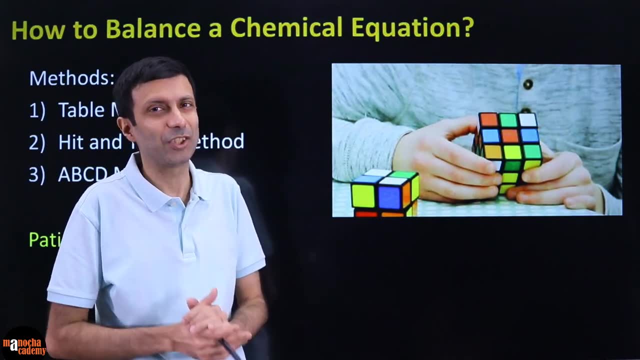 Solving the Rubik's cube. Have you guys played Rubik's cube? It is really fun and interesting, But you know I always forget. the method Really requires lot of patience and practice, But it is very fun to solve Because it is little hard. 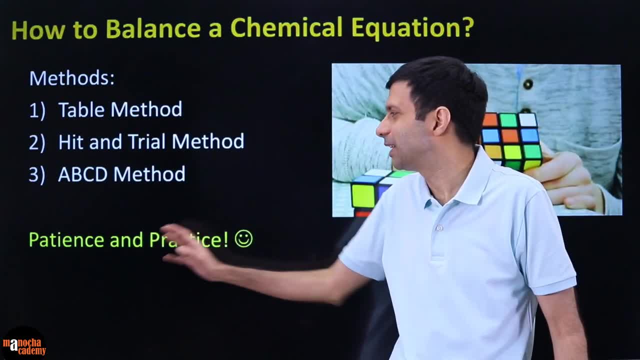 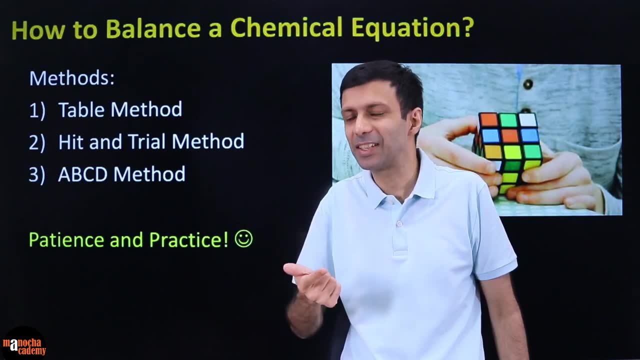 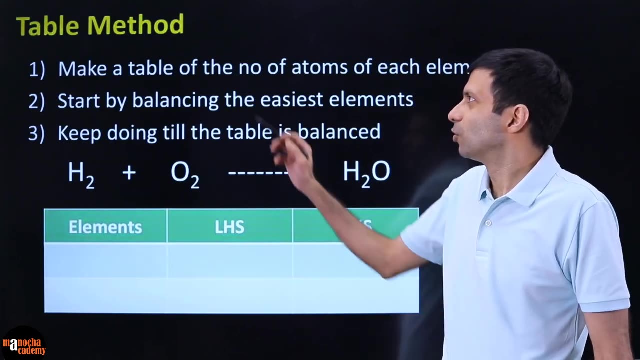 Same with balancing equations: That it requires patience and practice. And trust me, If you do it, Don't memorize the balancing. Keep practicing, You will become an expert at it. So first we will start with the table method. So what does the table method say? 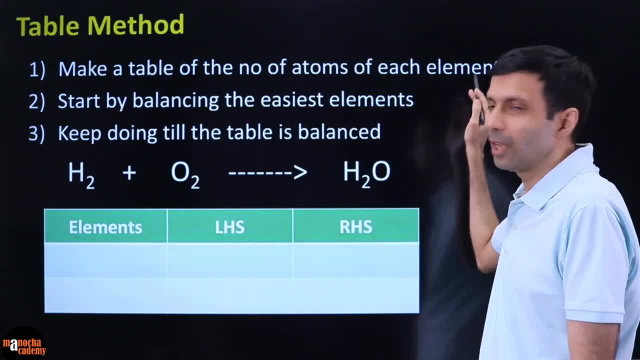 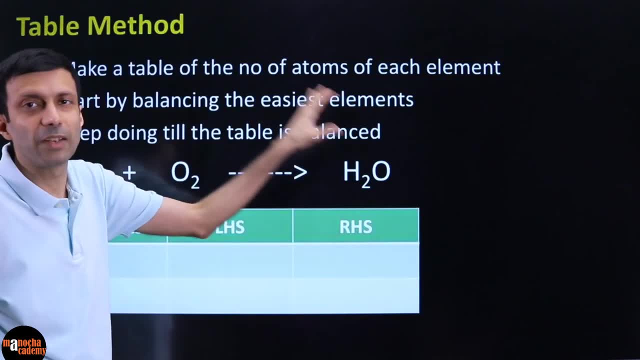 Simply make a table of the number of atoms of each element. So this is like you are doing accounting, Right, You are checking how many atoms of each element And our goal is to balance it. So the table gives you a very nice, easy visualization. 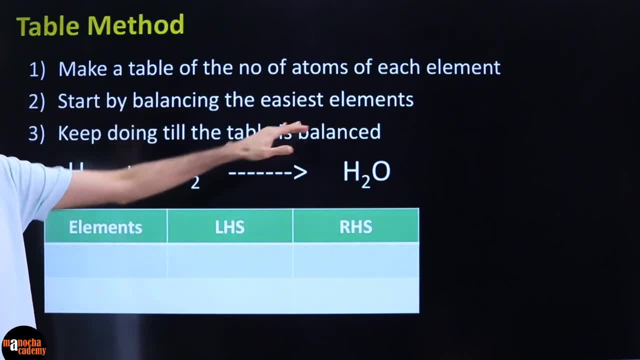 As we will see, Then you start by balancing the easiest elements And keep doing it till the table is balanced. So let's try it out. So, for example, we will again take our simple example: Hydrogen plus oxygen gives us water And everybody, please make this table right now. 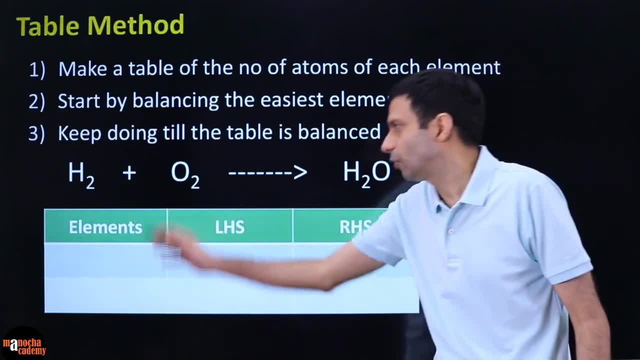 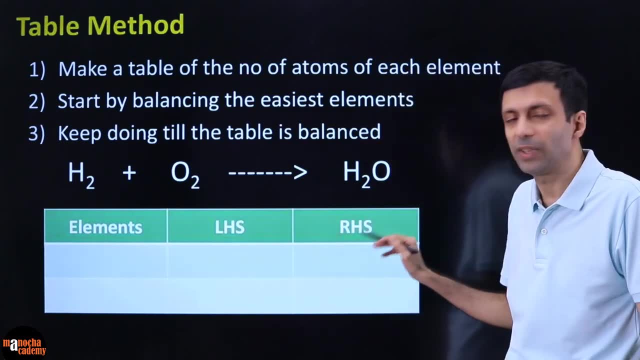 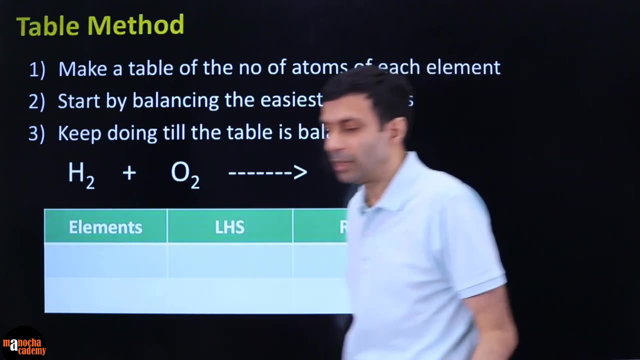 What is your table? There are going to be three columns in it: Elements- Left hand side, Right hand side And the counts of the atoms. So can you guys tell me What are the elements involved in this reaction? What are the elements here? 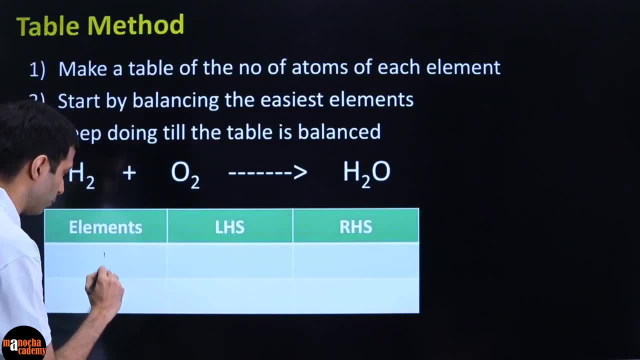 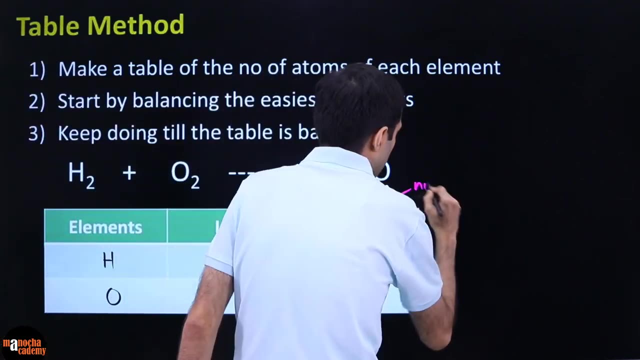 Clearly you can see the elements are Hydrogen and oxygen, So let's put that in the table. Hydrogen and oxygen: You can put whichever one. Since hydrogen comes first, I put hydrogen and then oxygen. LHS, RHS means What we are putting down here is: 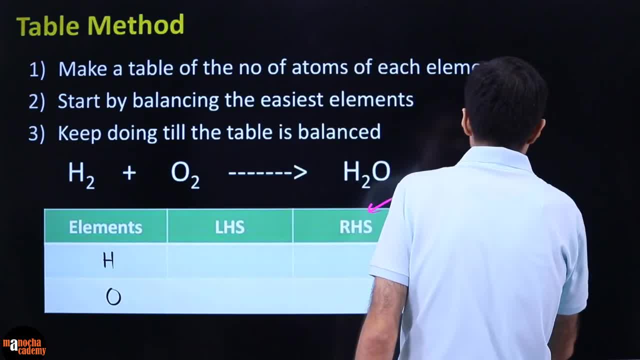 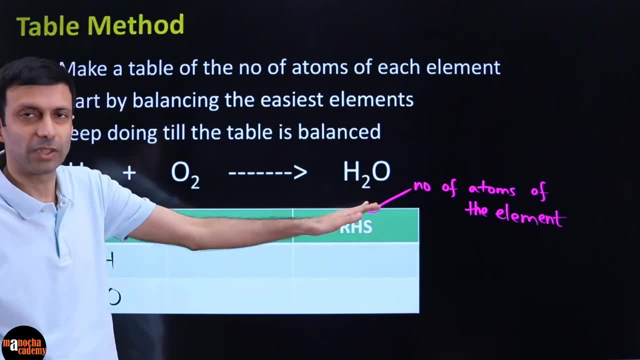 Number of atoms Of the element. So we will be putting down The number of atoms of each element. LHS means left hand side, RHS is right hand side. So on the left hand side, How many hydrogen atoms are you seeing here? 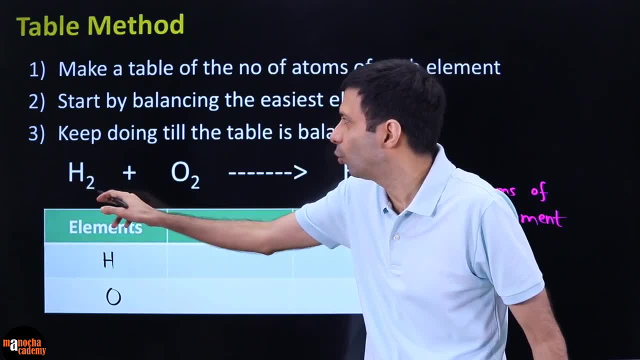 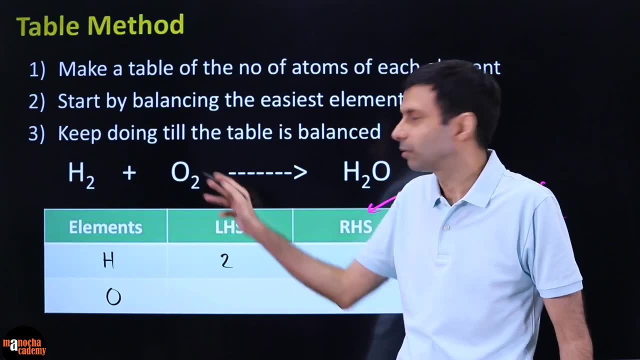 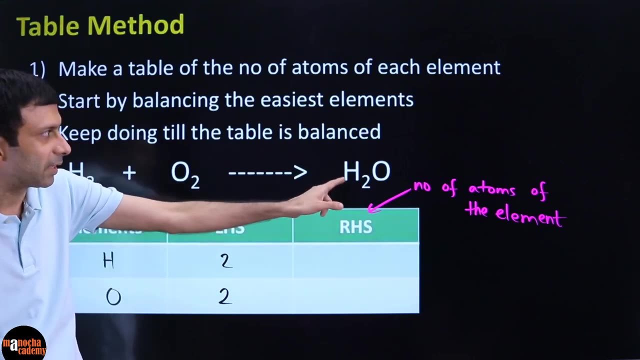 Can you tell me? Very good, the right answer is two, Because there are two atoms of hydrogen, One molecule containing two atoms. So let's put that down. How many oxygen atoms on the left? Again two, Two atoms. H2O is containing two atoms of hydrogen. 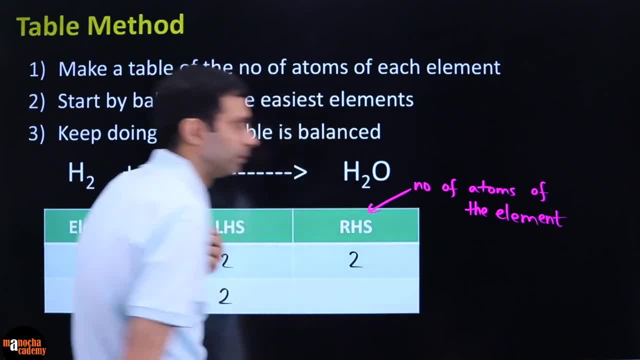 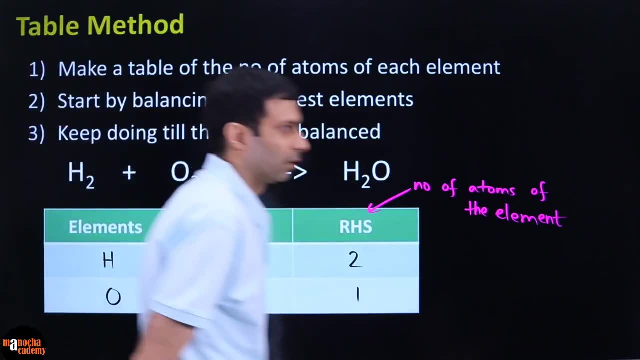 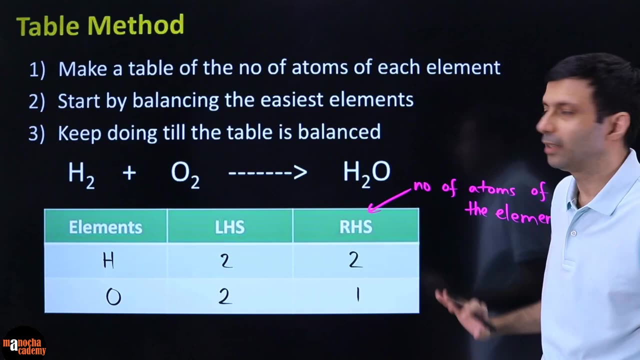 So I am going to put that here. Two: How many oxygen atoms? Water molecule has only one oxygen atom, One, Very good. So everybody please make that table And you can see it is a nice easy visualization. So you have made the table. 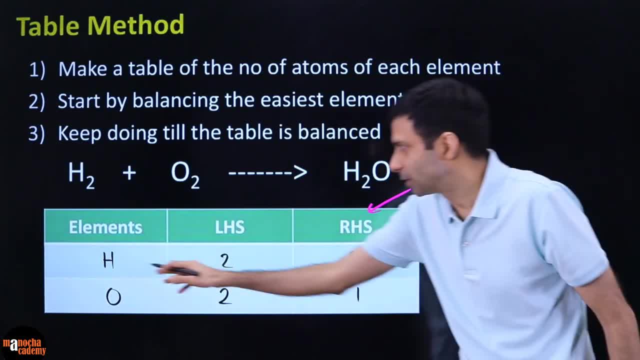 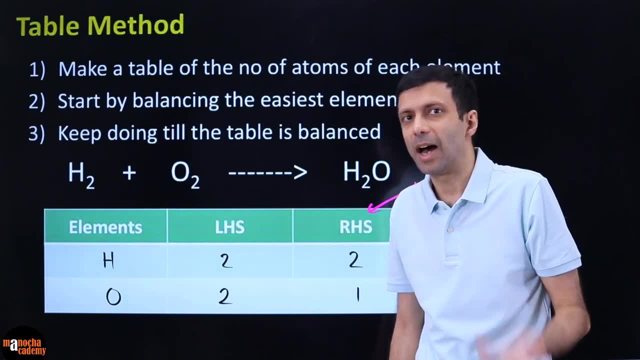 Now the goal is: If something is balanced, Like hydrogen, you can see Two and two. it is already balanced, So we don't have to worry about it. If there are unbalanced elements And if there are multiple of them, Do the easiest one first. 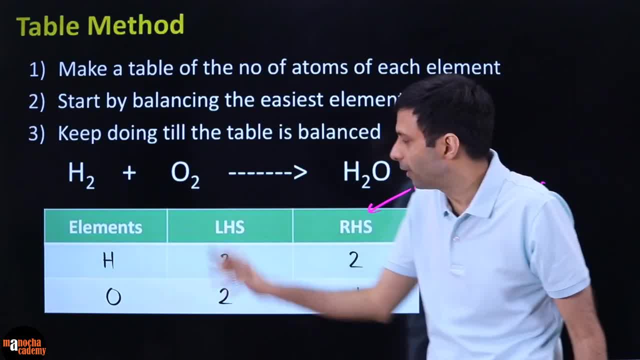 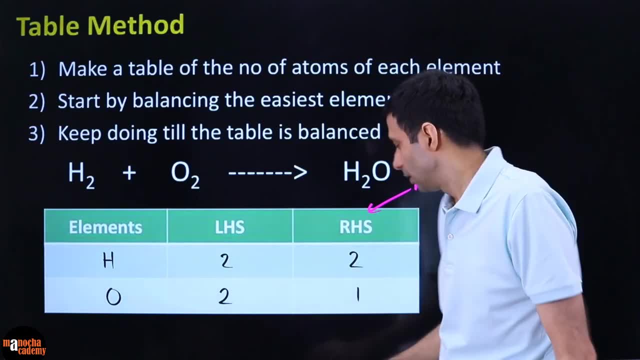 So here there is oxygen, So we have to do that. Oxygen, you can see, is two on the left, One on the right, So obviously we have to increase on the right. Now, how do we increase? Can we simply change this formula? 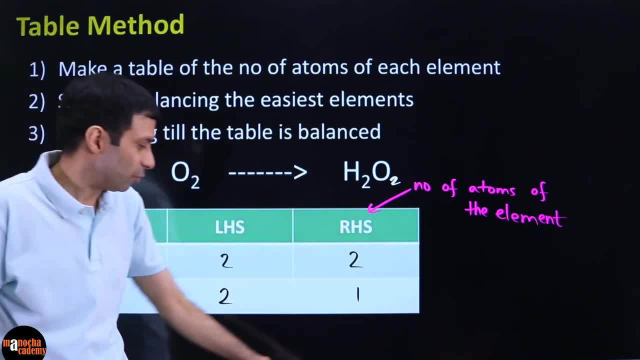 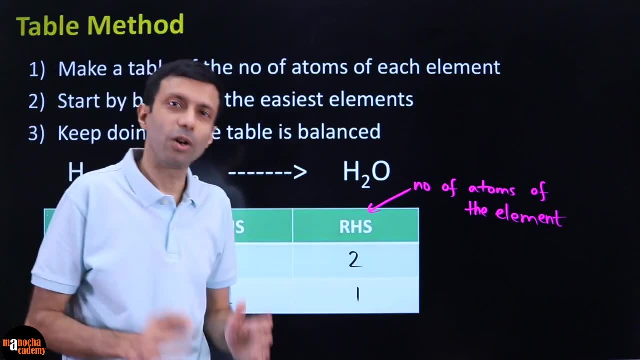 Can we do H2O2?? This is no longer water, This is hydrogen peroxide. So this is a crime. in chemistry. You have committed a crime by changing formulas. Remember: all you are allowed to do Is just do multiplications. 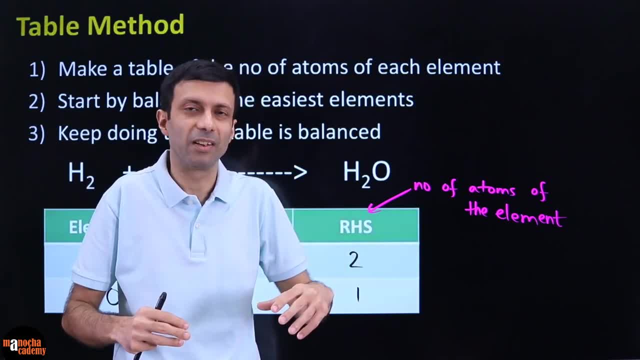 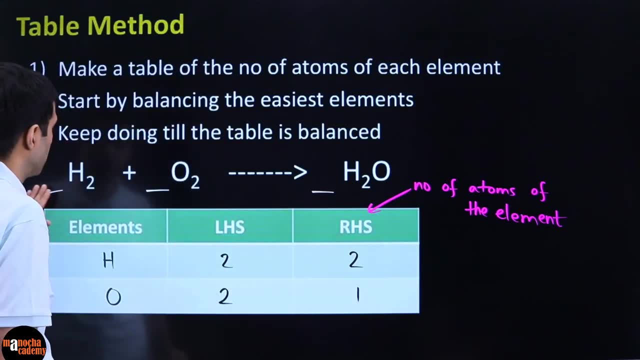 Means, just like a fruit seller adds apples Or adds weights, Same way you can just put multiples, So you can put multipliers In front of these. That's all you can do, So that's all you are allowed to do. So how do I? 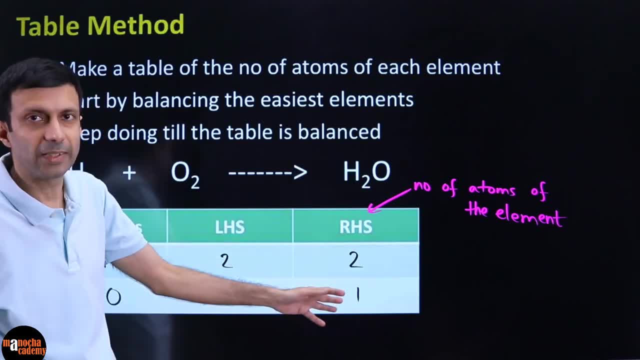 Clearly I want to increase on the right hand side, So left hand side is two, Right hand side. if I want to increase, Let me multiply by two. So some of you might say why didn't I multiply by three, four or five? 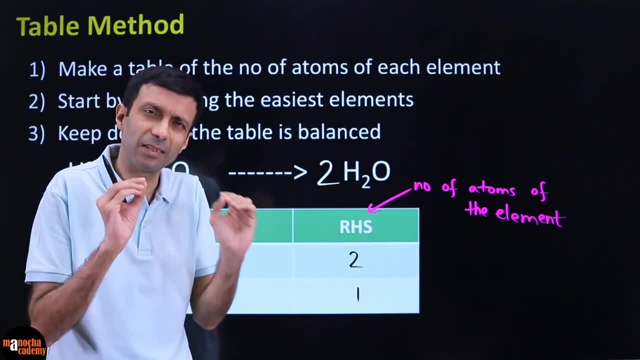 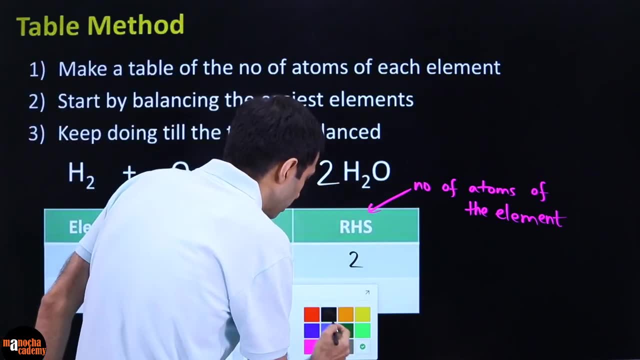 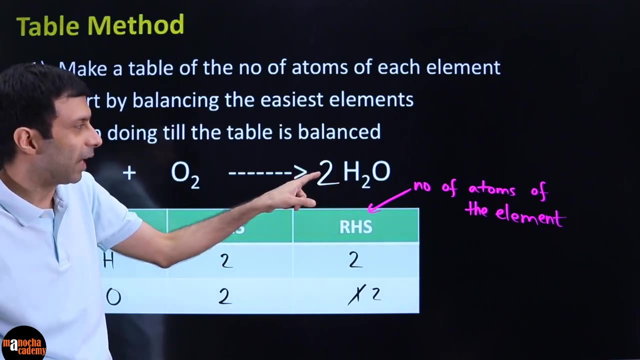 Why do you want to be so generous? Just that much which is needed. So be frugal, Don't be generous. So we have multiplied by two here. So what will happen? Oxygen will become two, But we have affected hydrogen, Because how many hydrogen atoms now? 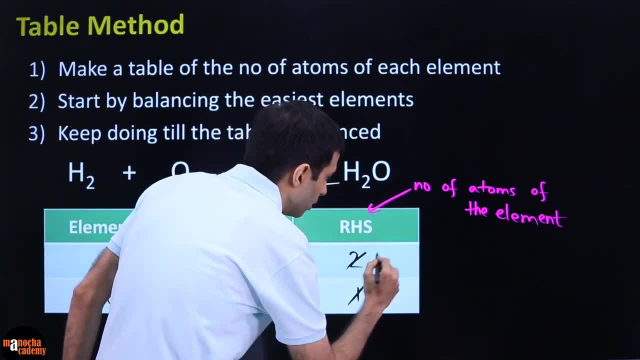 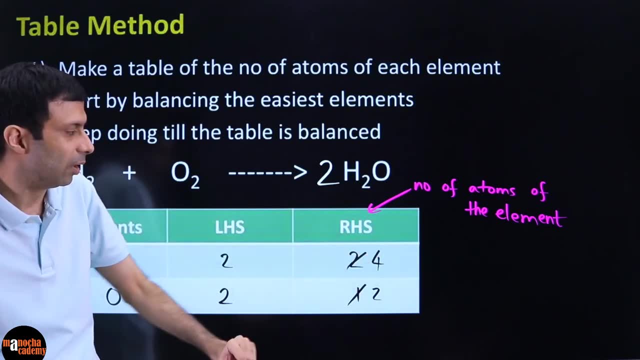 Two times two: Four. So cut it. Cancel it like this. You can use an eraser Or you can simply cut it. This is four. So see, oxygen row is now balanced. That means we don't have to worry about oxygen. 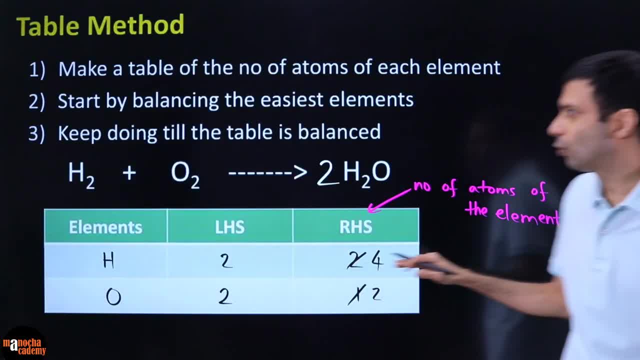 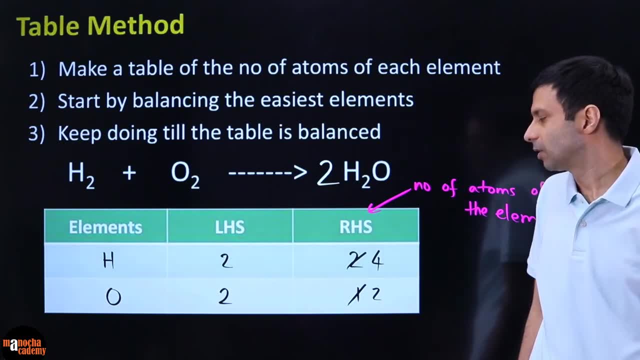 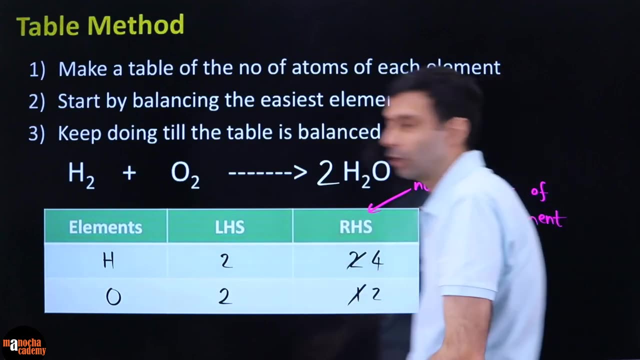 But hydrogen is clearly unbalanced. Hydrogen is clearly unbalanced here, Yes. So what are we going to do? Because hydrogen is unbalanced, We are going to multiply Because it's more on the right, Less on the left, So the multiplier should be on the left. 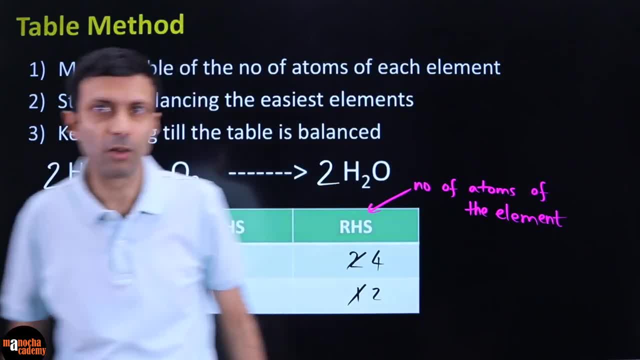 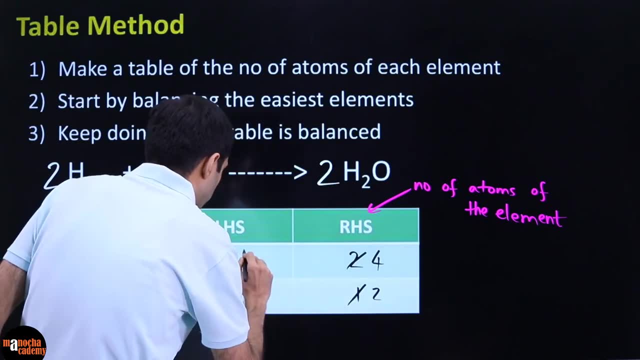 So let's multiply by two here To balance it. Always, your goal should be to balance it. If you multiply by three, it will become six and four. So now you can see, Hydrogen has also become four. So that's what keep doing till the table is balanced. 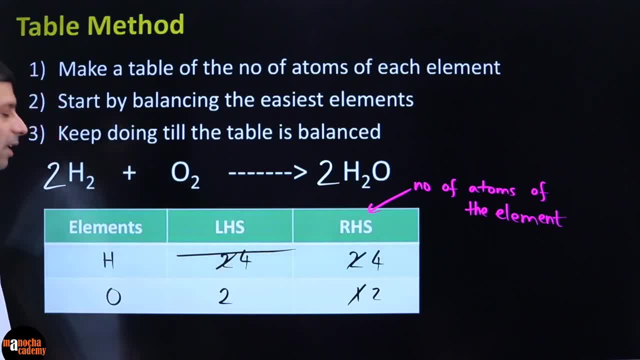 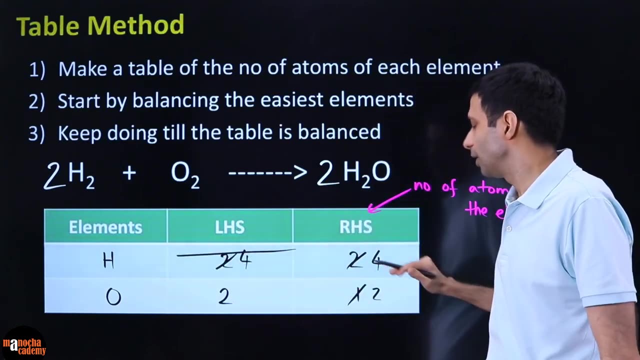 Table. balance means each and every row should be balanced. As you can see, Hydrogen is four- four, Perfectly balanced. Oxygen two: two. It's balanced. Is that clear? So this is how you balance these kind of equations: By making sure that each and every row. 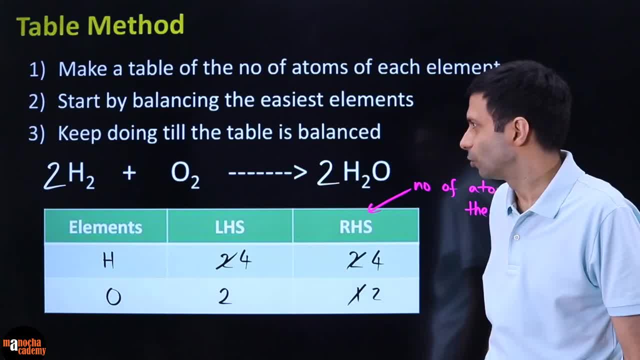 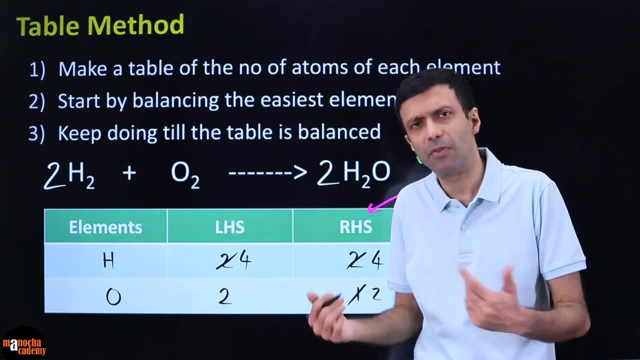 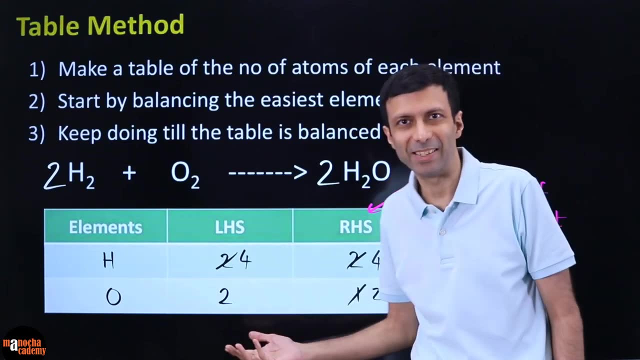 The number is matching. So there you go. Here we can see Our equation is balanced. So this is called the table method. It's a very simple method: Make this table, Keep cutting, making sure each and every row gets balanced, And then you get it. 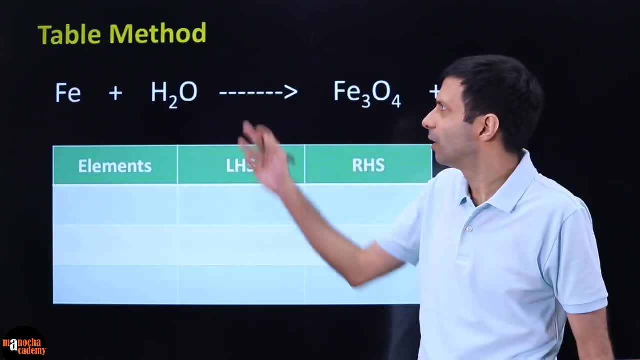 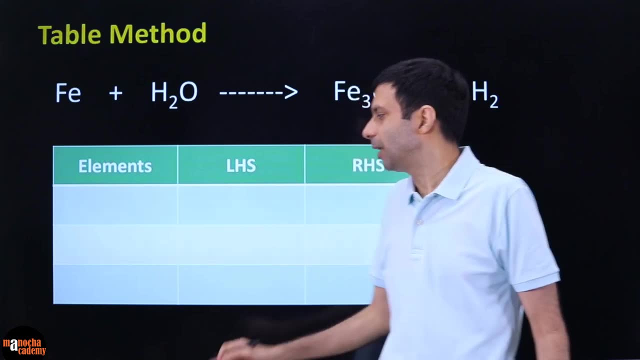 Let's practice table method with this one. So come on everybody, Write down this equation And you can check with the table. If it's balanced, then you don't have to do anything. So this table helps you account for all the numbers. 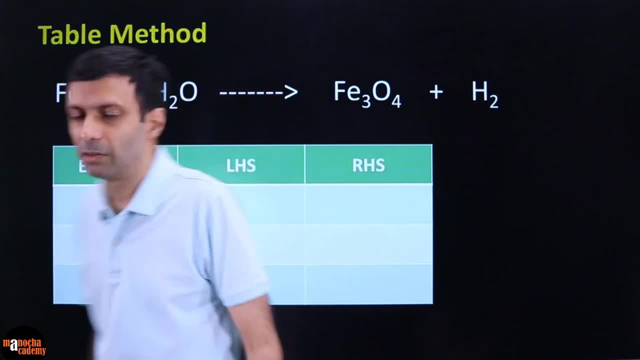 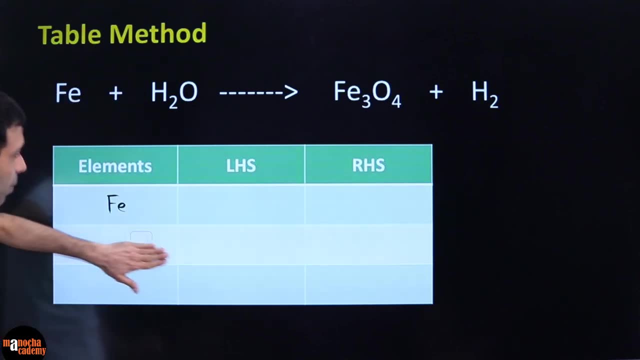 So let's try it out. So what are the elements over here? This time we have iron, And please don't put water here, Because water is a compound. You need to break it into hydrogen and oxygen. This is the table of elements. 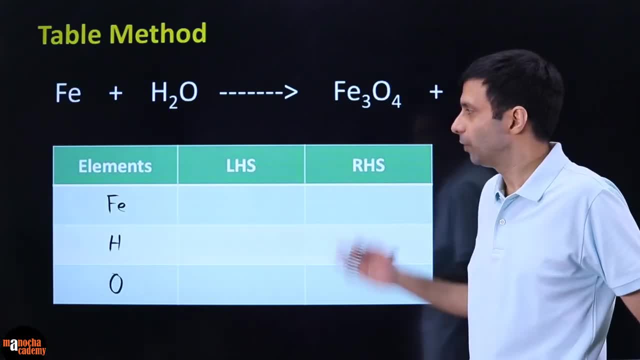 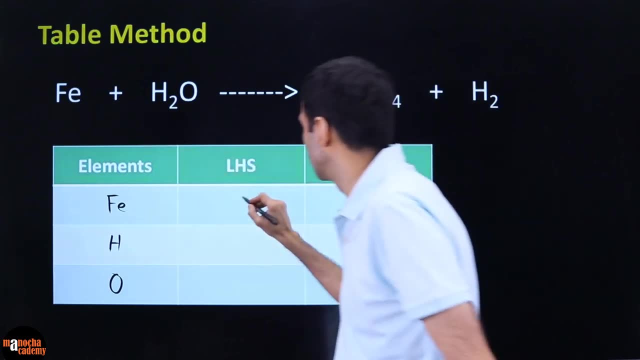 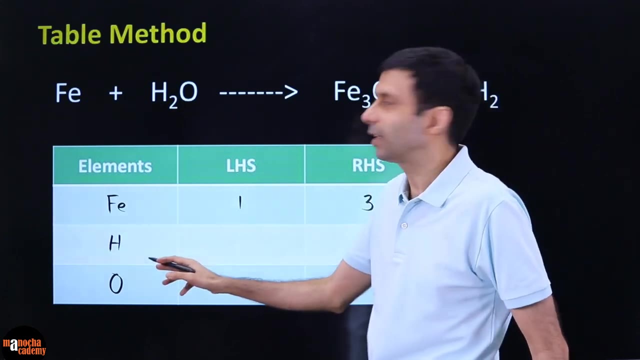 Okay. So yes, it's simple, Let's practice the table method Now for each element. for iron, Left hand side: how many atoms of iron? One atom? How many atoms of iron on the right Three? How many hydrogen atoms on the left side? 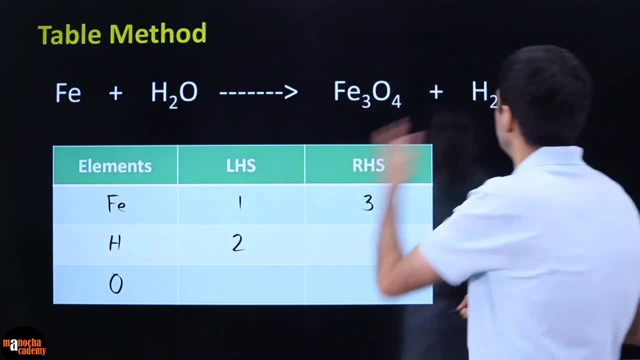 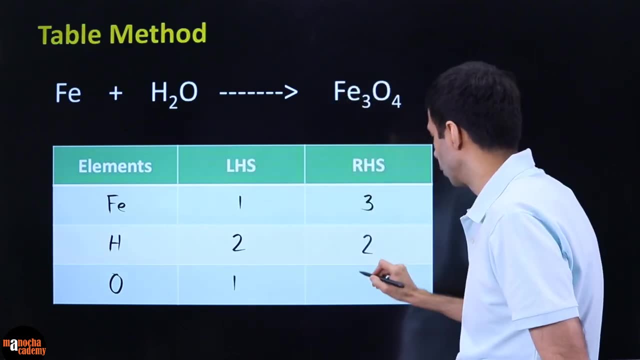 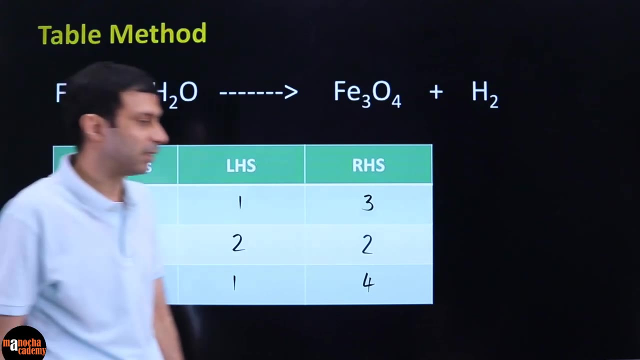 Two, We will put two here. How many hydrogen? on the right Two, We will put two Oxygen, one on the left, On the right four. So there is our table. Do you guys agree with this? Now, what did the table method say? 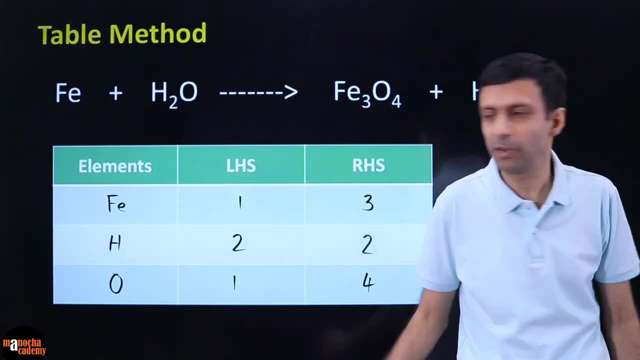 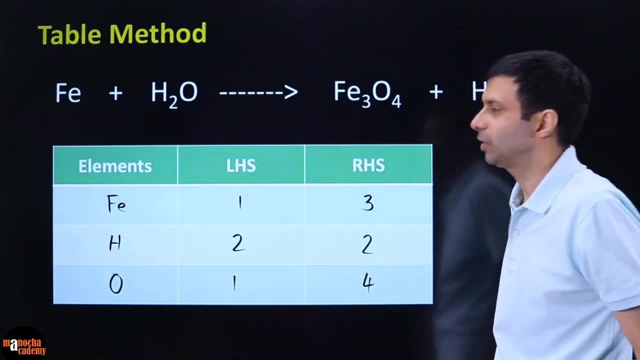 Start by balancing the easiest element, So whichever you find easy. So you can say: hydrogen is already balanced. I need to change either iron or oxygen, Whichever one you want to do. Okay. So let's say: we find iron easy, So let's go ahead and change that. 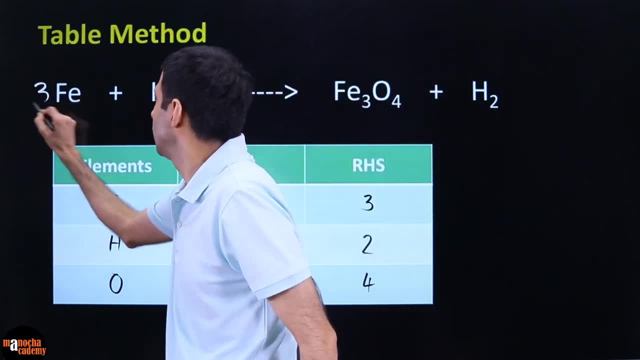 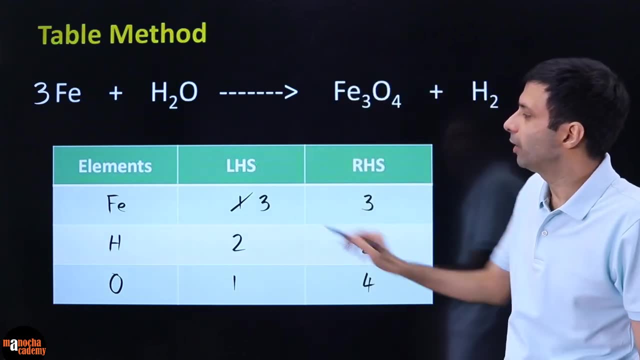 So it should be simple. We will simply multiply by three here And iron becomes balanced. Iron is done Now. oxygen is four here. So clearly on left hand side we have to add a multiplier. So let's put the multiplier here Four. 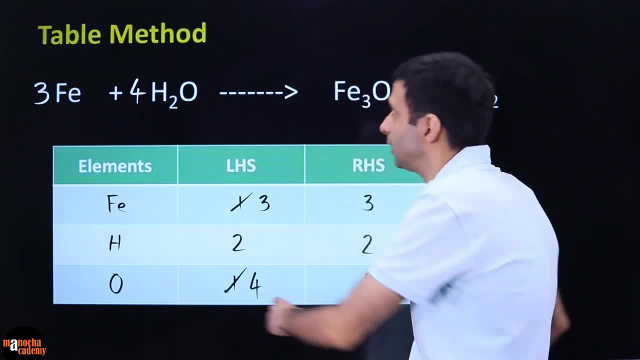 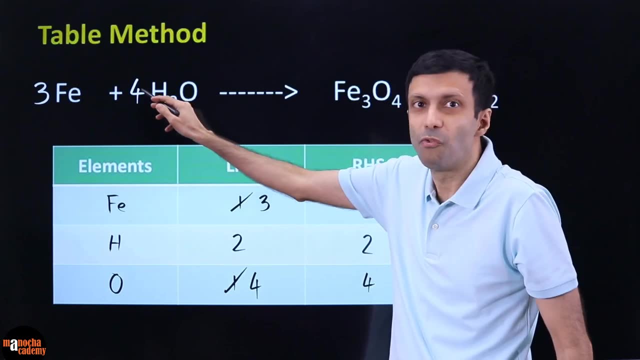 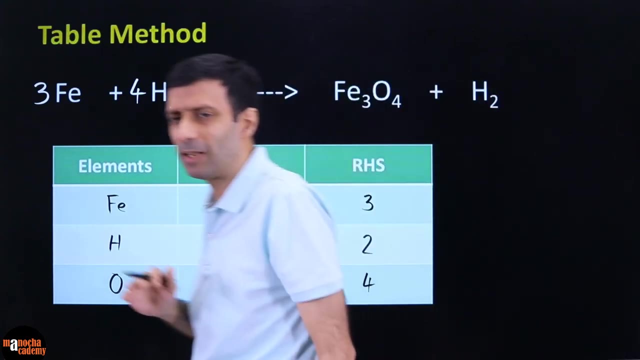 Oxygen is clearly balanced on the left now, But see, we have affected the other element. Don't stop here, Because you have put a four in front of hydrogen. How many hydrogen now? Four times two, Eight, Is that clear? So don't worry. 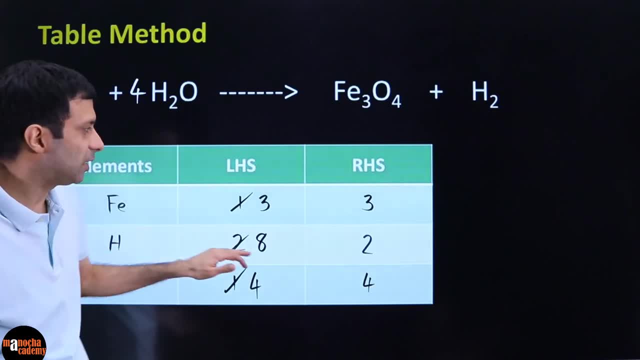 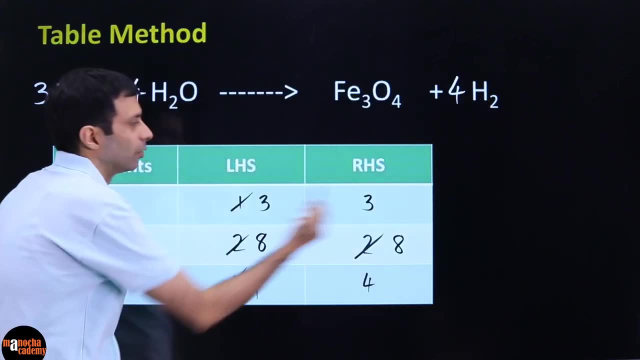 You have spoiled the balancing, But we can always adjust it on the other side. So hydrogen is eight here, Only two there. So how do we balance it? We will put a multiplier here of four. There you go: Three, three, eight, eight, four, four. 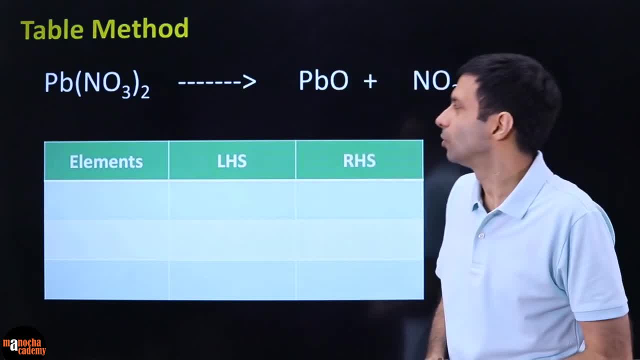 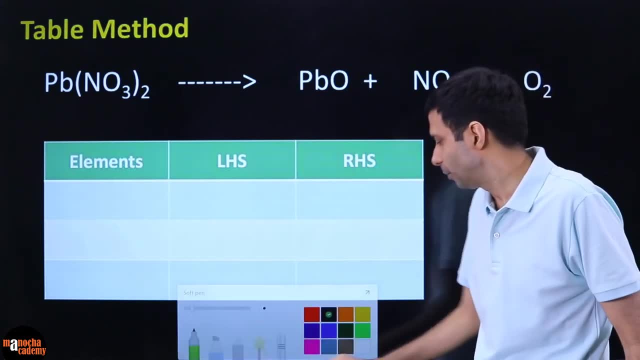 Table done And this is our final answer. We have this lead nitrate. When you heat it, it breaks into lead oxide, nitrogen dioxide oxygen. So come on, All of you make this table. What element should I put in here? 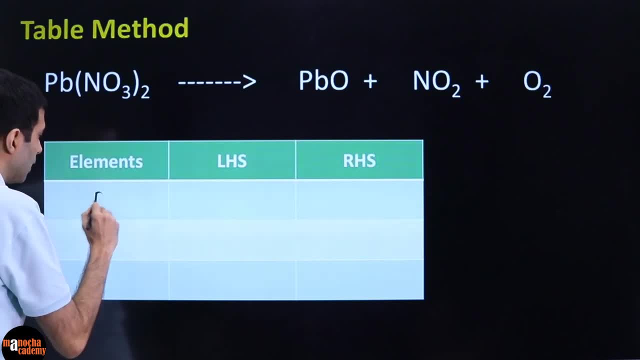 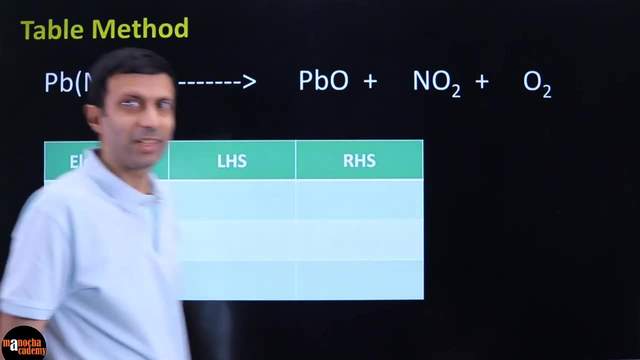 So always start from the equation. If you start from the left, there is lead, So let's put lead first. Nitrate is not an element, It's an iron. It contains nitrogen and oxygen. Remember: nitrate is a polyatomic ion containing nitrogen and oxygen. 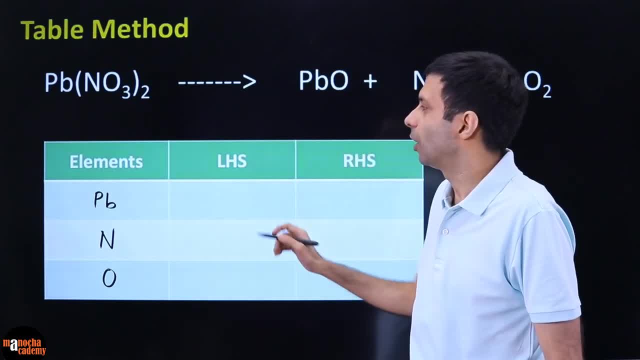 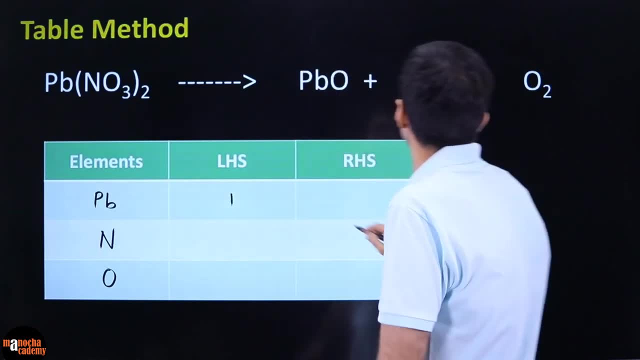 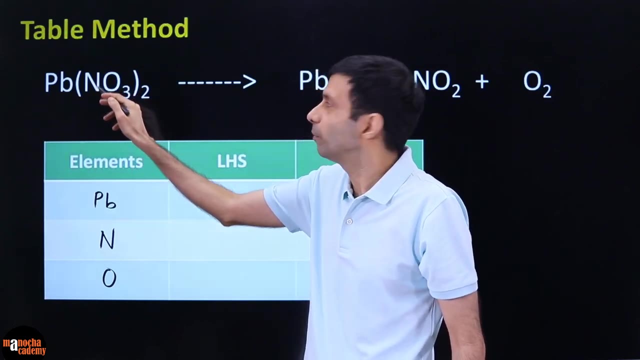 So please put that Now. number of atoms: How many lead atoms on the left This is Pb1 or Pb right. So one lead atom, How many on the right One? How many nitrogen on the left? NO3 has only one nitrogen. 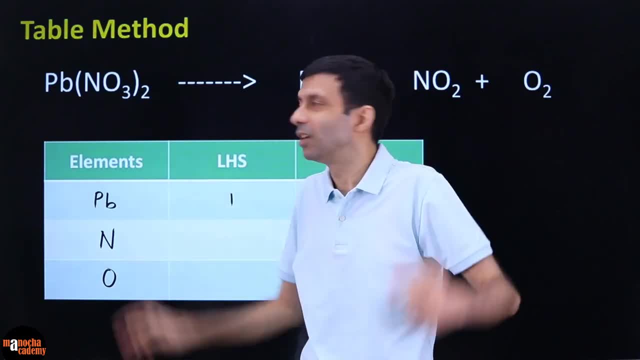 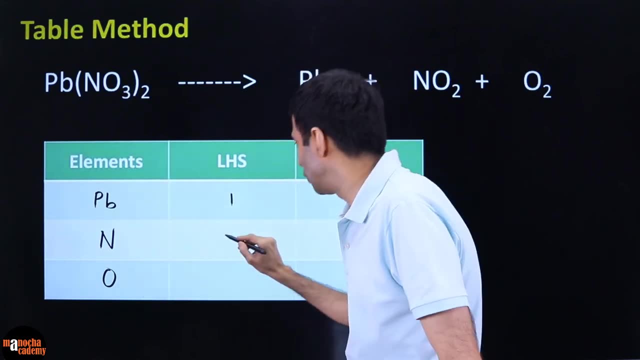 But there is a whole bracket two. That means there are two nitrates, So two times one. Be careful of the counting If the counting is wrong, gone. So two nitrogen on the left, How many on the right? Only one nitrogen on the right. 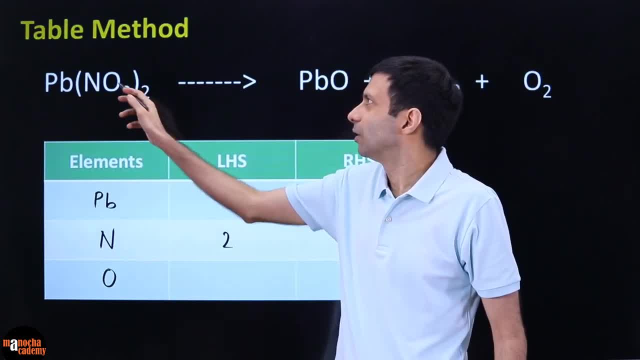 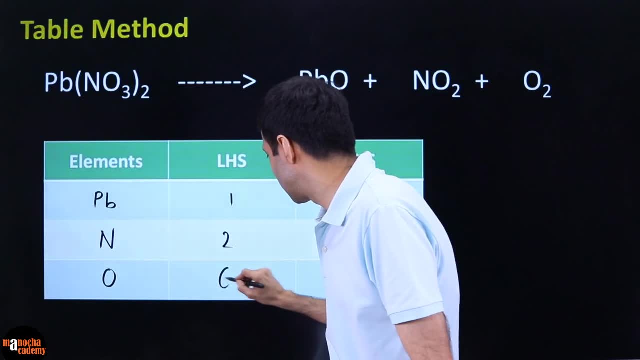 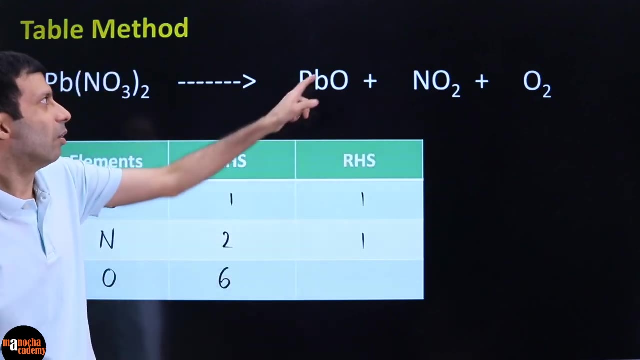 How many oxygen? Only one nitrogen on the left. Three oxygen in nitrate Multiplied by two, Because there are two nitrates, So six. Please don't do three plus two. Three times two, Six. How many oxygen on the right hand side? 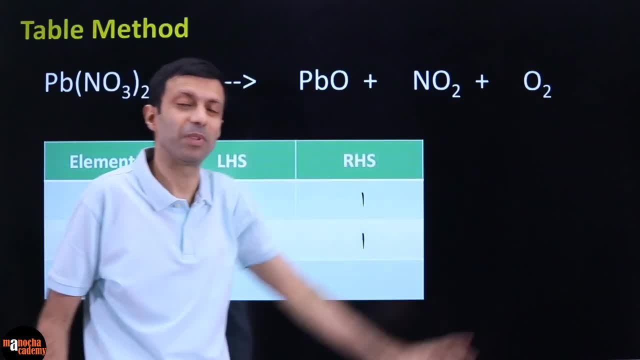 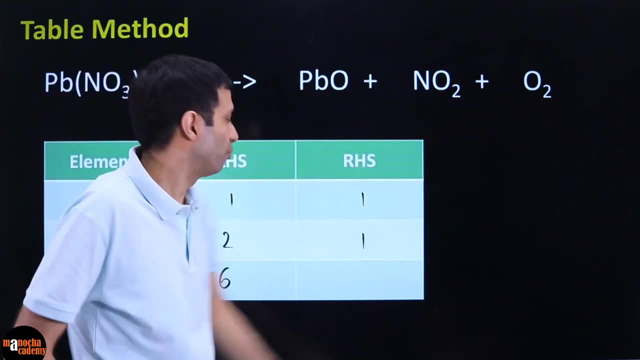 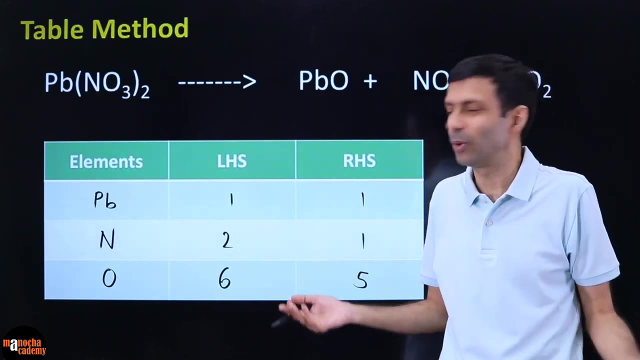 One plus two plus two, You have to add up all. If the element is present in multiple compounds, You have to add substances. You have to add it up. Two plus two, Five. So there is our table. Always check if everything is balanced in the table. 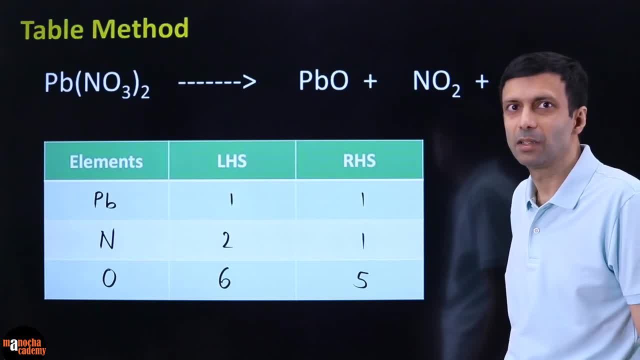 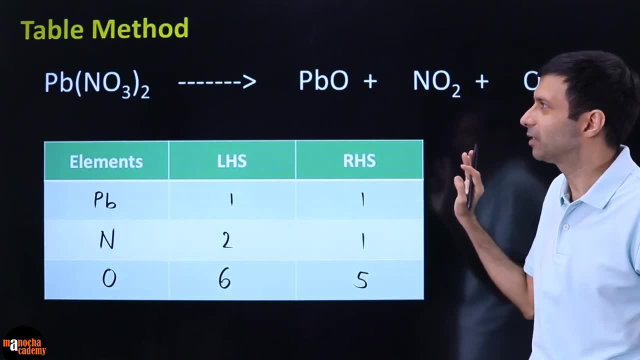 Then great news, You don't have to do anything. But clearly you can see, only lead is balanced. These two guys are not balanced. Which element is easier to balance here? Clearly, nitrogen looks easier to balance Because oxygen is all over the place. 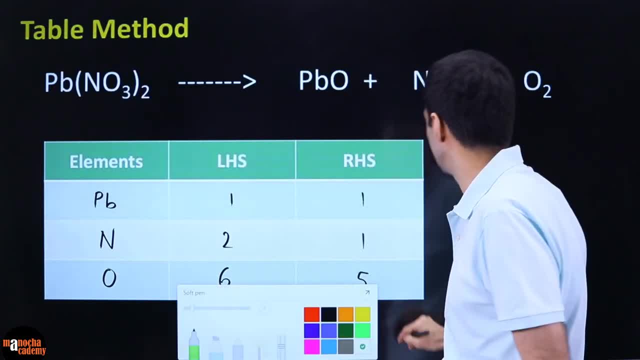 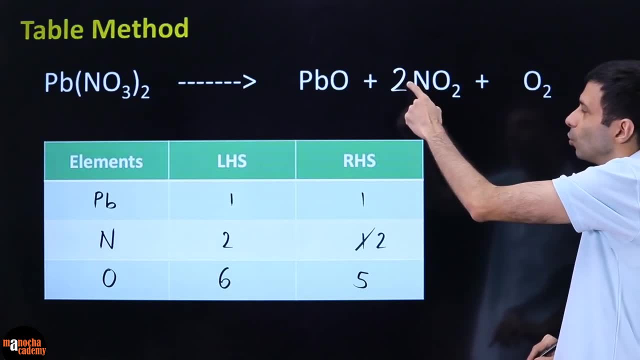 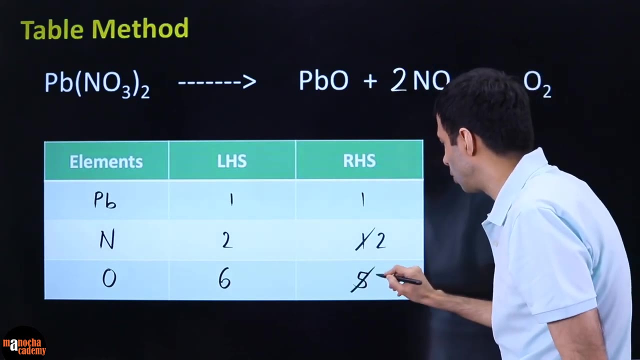 So let's finish off. nitrogen. Nitrogen, only two on the left, One on the right. Nitrogen here, But how many oxygen? See you have affected oxygen, So don't forget that. Two times two, Four, Five, Six. 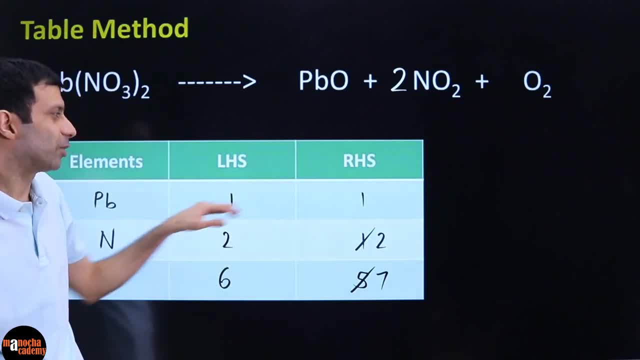 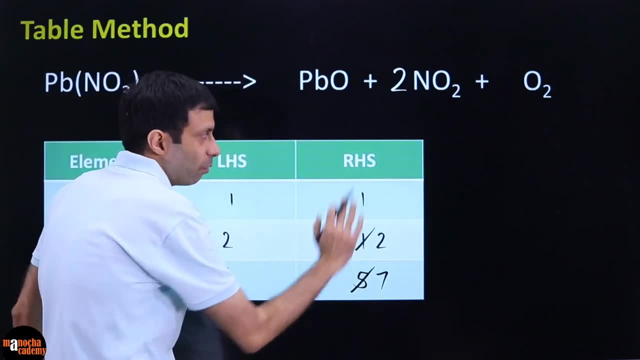 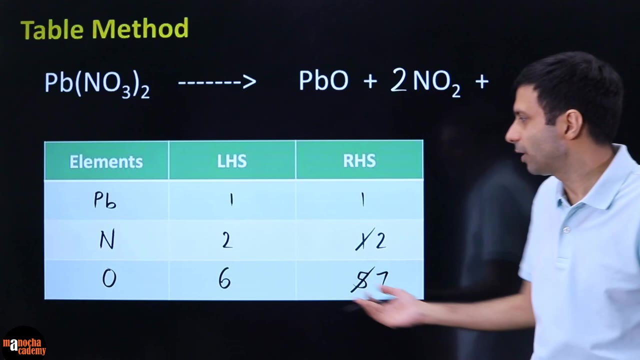 Seven. So oxygen still remains unfortunately unbalanced, Because this is one, one, Two, two, But six and seven. Don't worry, Don't get scared, Do you guys see that? So where should I increase, Since it's more on the right, less on the left? 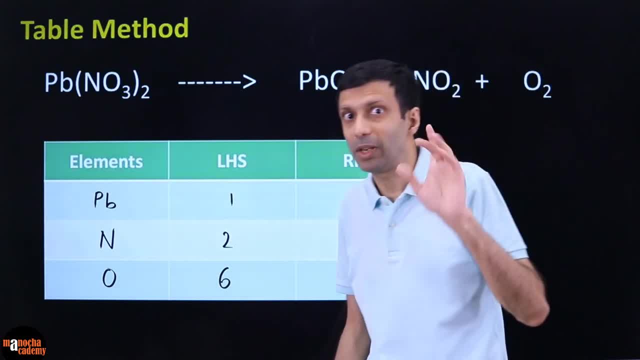 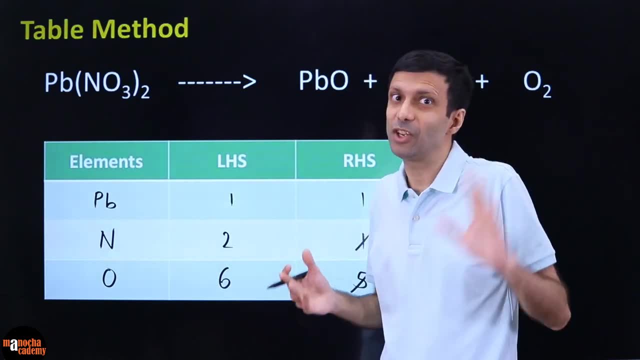 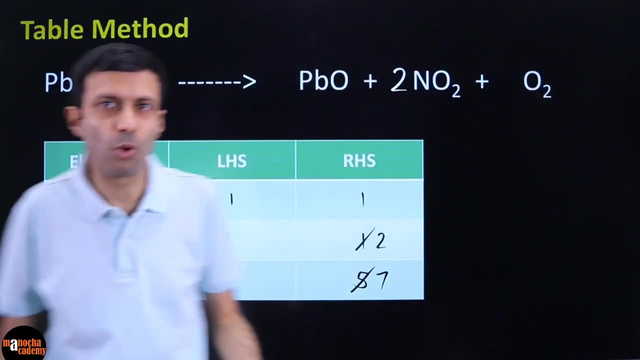 We will increase the oxygen on the left. How do I increase? Only multipliers. So what we need to do, Multiply again with the smallest number. Don't be too generous. Be generous in life, But not with equations. So six and seven: 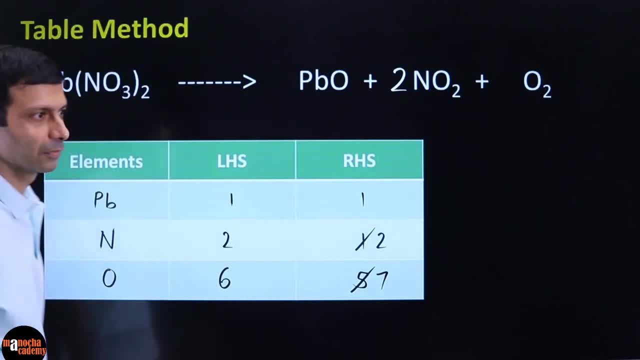 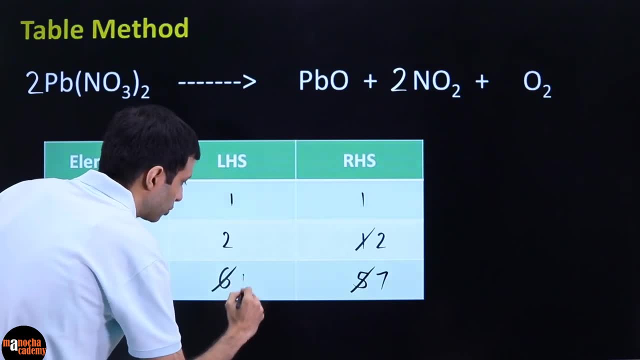 So let's multiply this entire thing. We have no option but to multiply this entire reactant by two. Do you guys agree? The table will multiply by two All the elements we have multiplied by two. So six becomes twelve, Two becomes four. 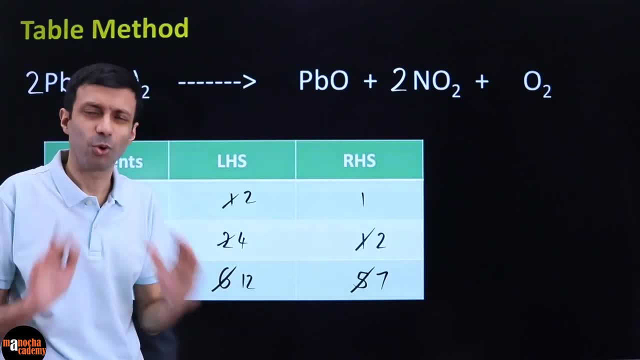 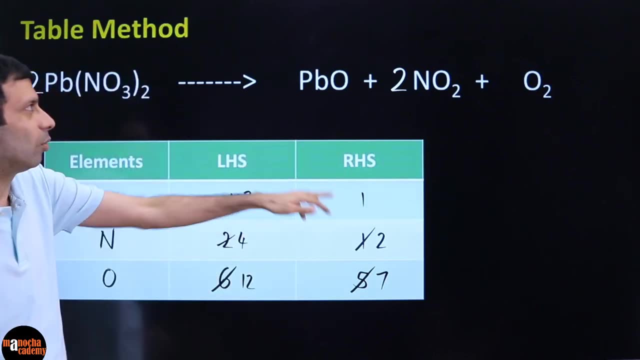 One becomes two. So looks like we have disturbed the whole table. But don't worry, We will again go and balance each element Again. we will start with the easy ones. So lead is two here, Only one there. So first let's finish off lead. 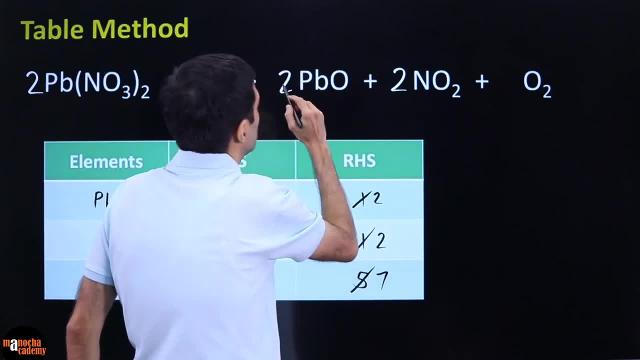 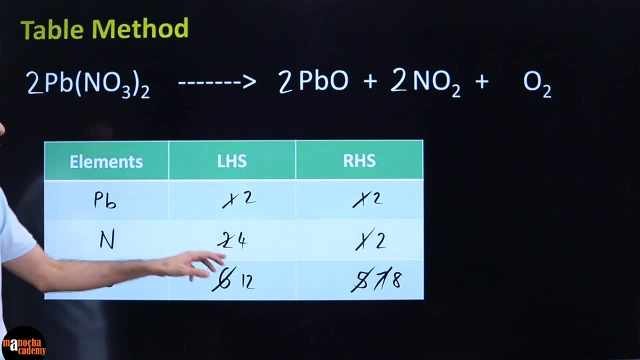 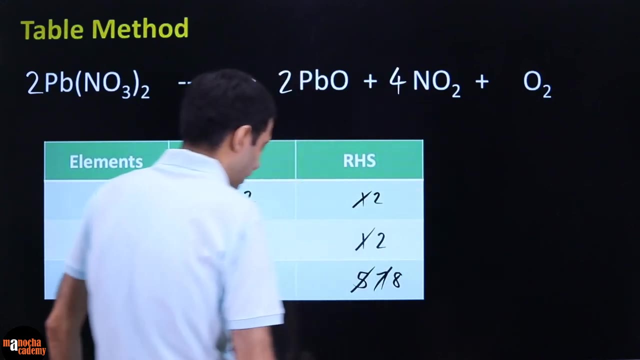 Two times lead here. That should take care of two lead And oxygen is now two Plus four, which is six, Seven, eight Nitrogen: four here, Only two there. So let's multiply this nitrogen by four now To balance nitrogen. 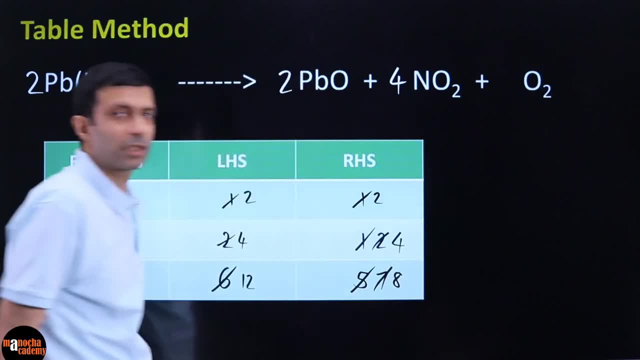 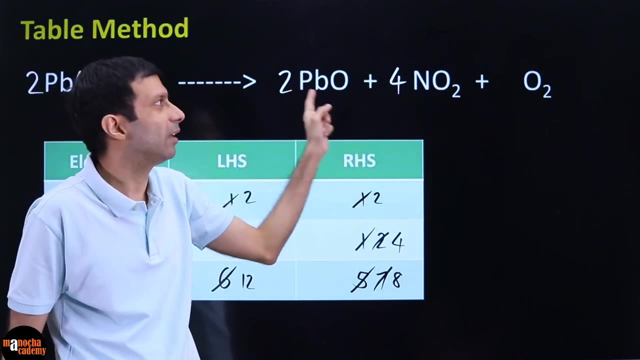 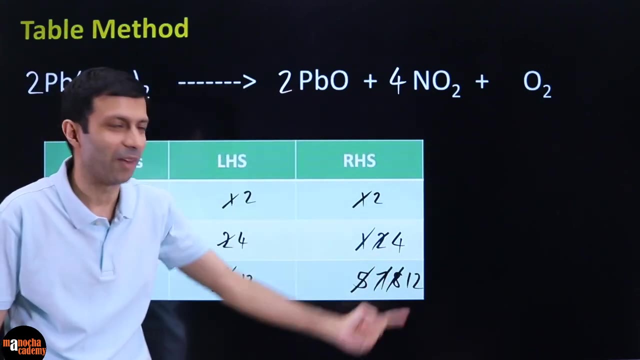 So nitrogen has got balanced. How much oxygen do we have now on the right? Two Plus four times two, eight. So eight plus two, ten Plus two, twelve, And the good news Can you see: Oxygen twelve. So even though we started with the easy, 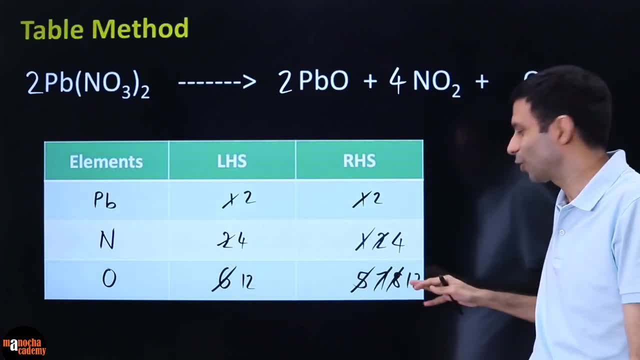 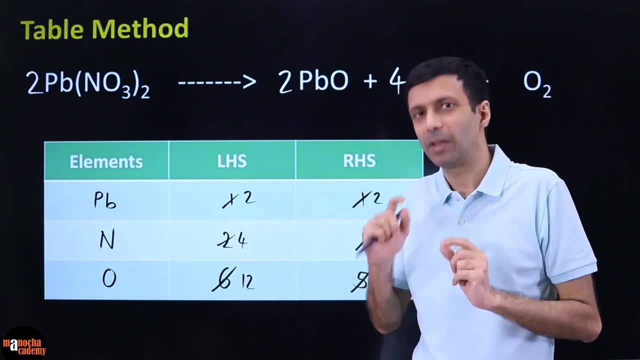 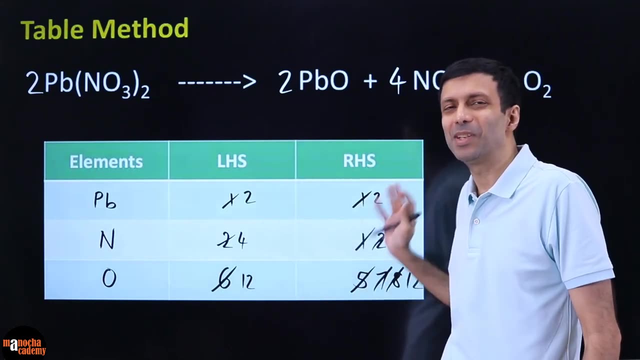 We did the easy ones first. The difficult one automatically got balanced here. So this is the nice thing about table method: Do it one element at a time. If you multiply, you might be disturbing the others. Don't worry, It's just like you know. you are keeping your statistics or numbers here. 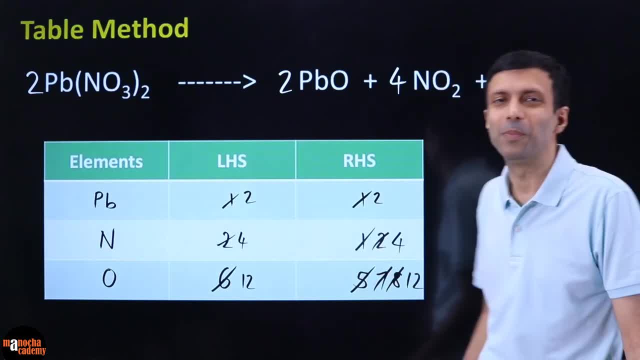 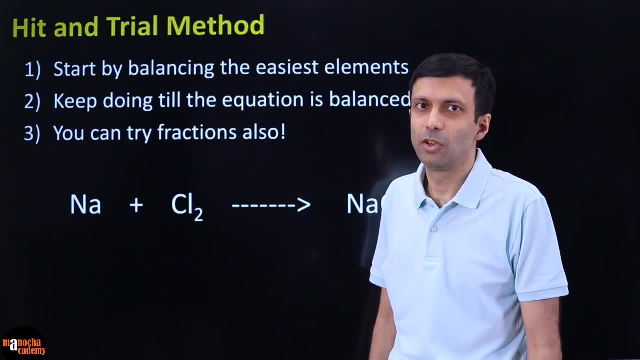 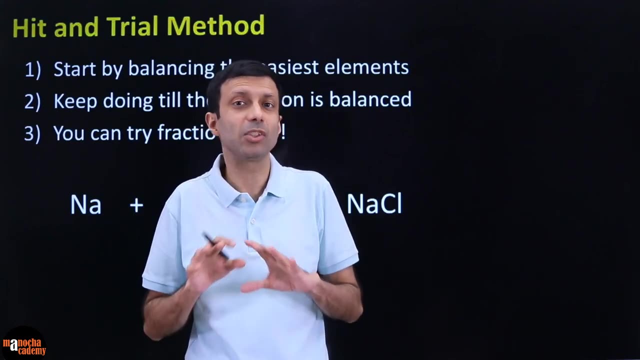 And finally check that each and every row will get balanced. So we have done the table method. Now let's look at the hit and trial method. So in hit and trial, method is more like you know, trying it out, Trying different numbers and trying to balance without drawing the table. 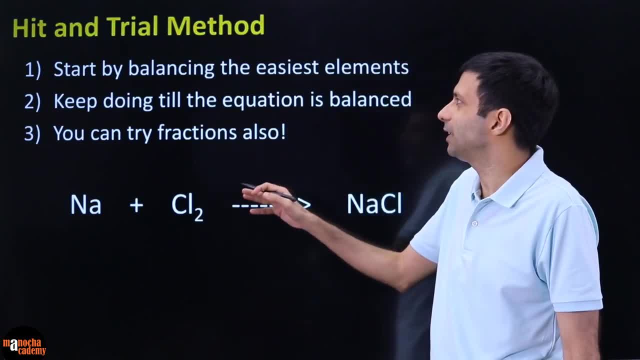 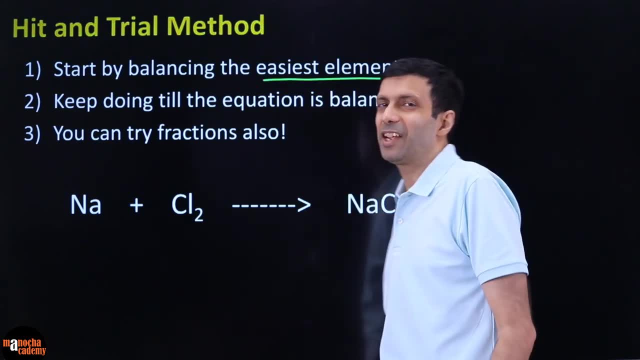 So the nice thing is it is quick and easy And you can start by once again balancing the easiest ones. Just like you know, when you have to study for an exam or do the syllabus, We always try to finish the easy chapters first. 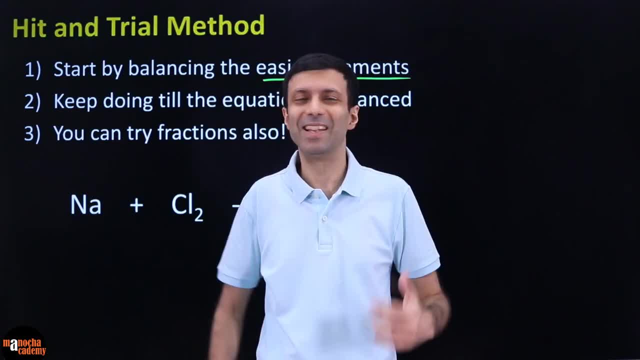 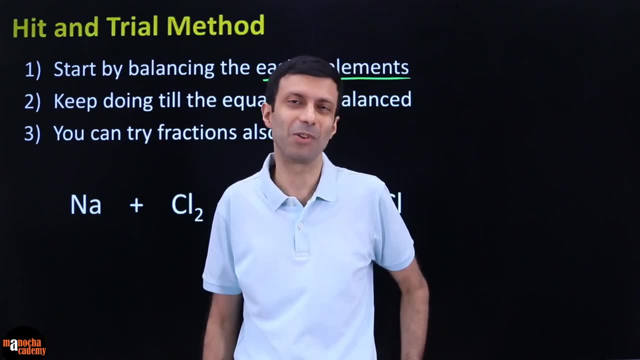 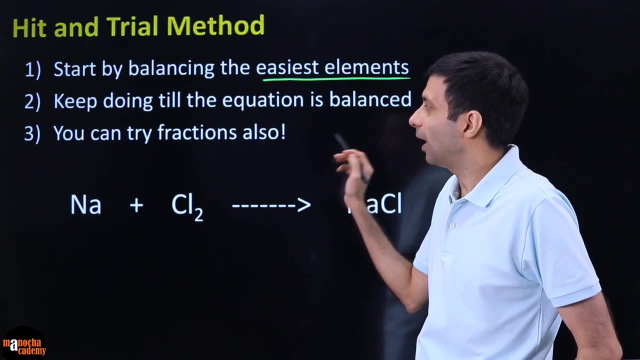 So that our confidence gets boosted. Same thing with balancing equations: Finish balancing the easy one first, Because sometimes automatically the difficult ones get balanced. So do the easiest elements first And keep doing it till the equation gets balanced. And I will teach you another nice technique where you can try fractions also. 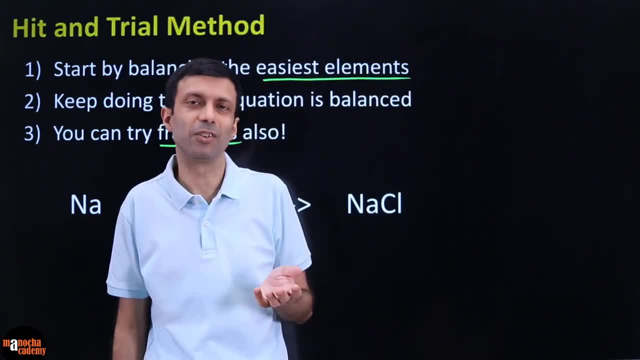 So we said we are multiplying. Usually we multiply with. you know natural numbers or normal integers, But you can even multiply, sometimes with fractions. I will show you those tricks. So let's say we want to balance this equation: Sodium plus chlorine gives sodium chloride. 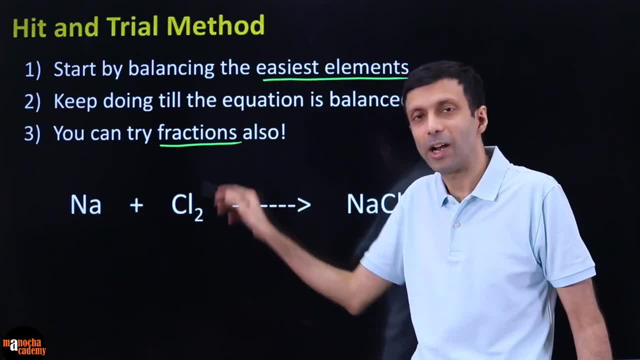 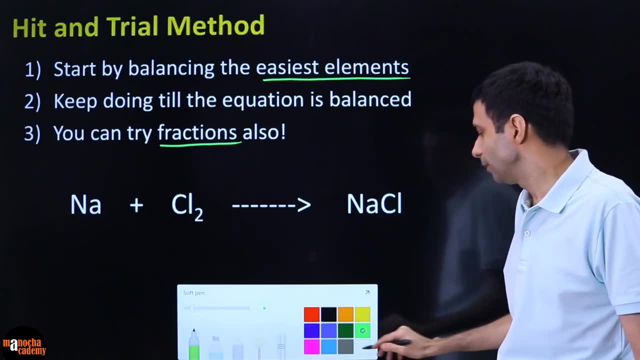 See again. Sodium is monoatomic, It is a metal Chlorine diatomic written as Cl2.. And sodium chloride compound valency 1: 1.. So NaCl. So this is our equation. If I want to balance it One, I could draw the table. 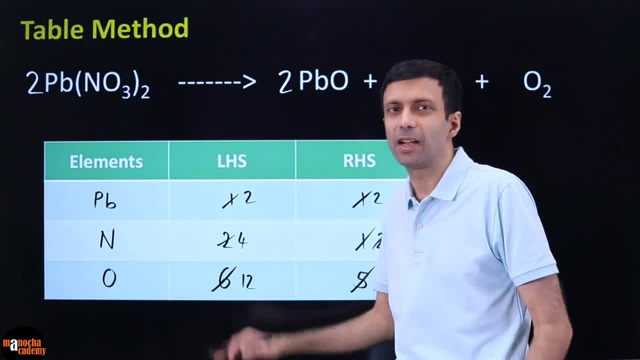 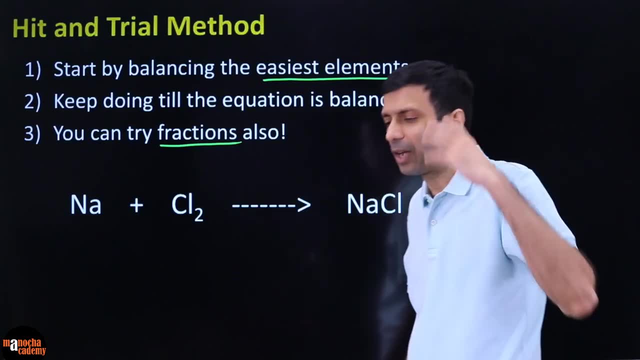 But table you saw is little lengthy. You have to write all this stuff. If they ask you to show the table, then please do it. But If you directly try to do it mentally, Hit and trial means try to do it mentally And just putting the numbers as you go. 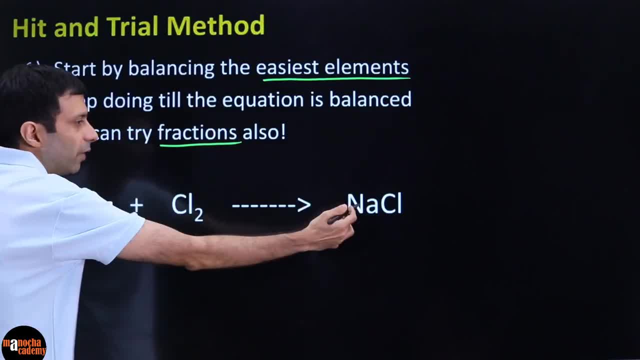 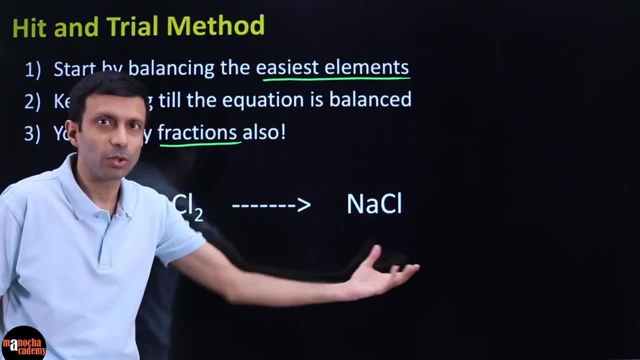 So what is happening here? You can see sodium is already balanced. One sodium here, One here. Chlorine is the guy which is problem. 2 chlorine, 1 chlorine. So chlorine is less on the right hand side. So put a multiplier of 2 here. 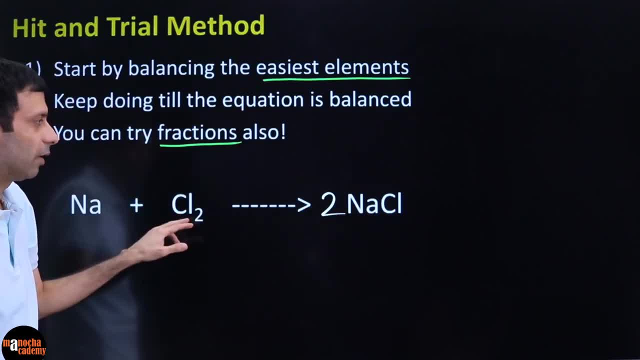 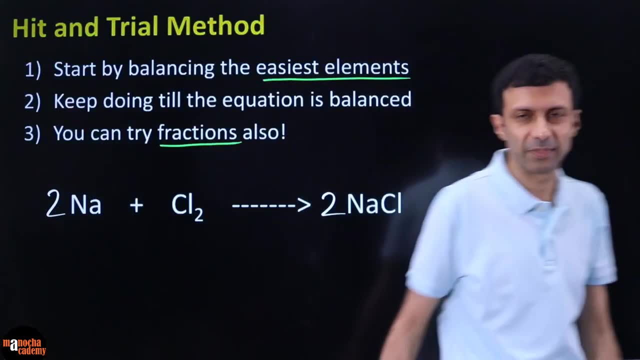 So can you see, chlorine has been balanced: 2 chlorine, 2 chlorine, But now you have made it 2 sodium. So simply put a 2 here And you will be done. That's it. So that's all the hit and trial method. 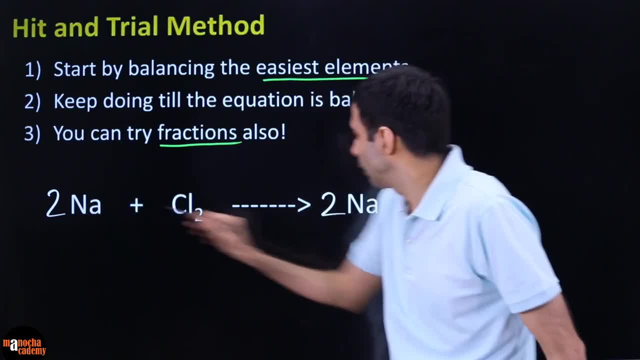 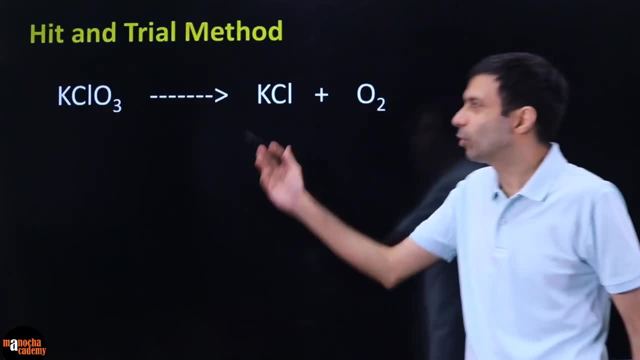 But since you don't have the nice table, Please do a double check: 2 sodium- 2 sodium, 2 chlorine, 2 times 1 chlorine, 2. Done. Do you guys want to try this one with the hit and trial method? 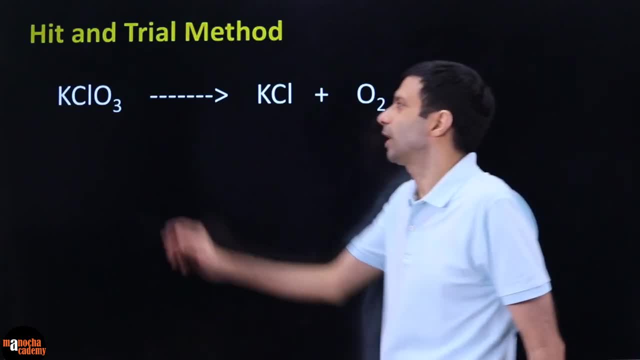 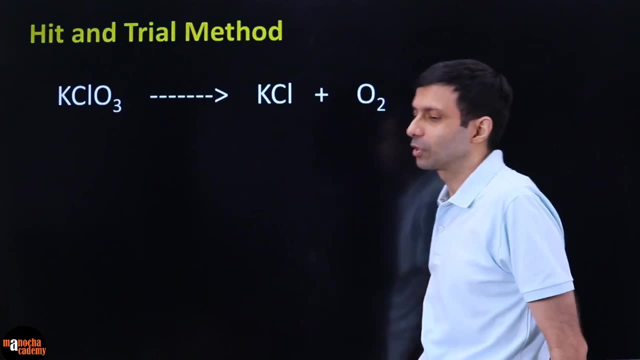 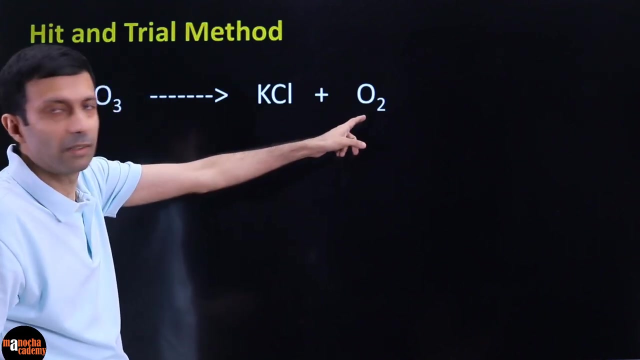 Come on, Try this So you can see: potassium Already balanced, Chlorine already balanced Oxygen is 3.. But oxygen is 2 here. So always ask yourself the question: Where is oxygen less? It's less here, It is more here. 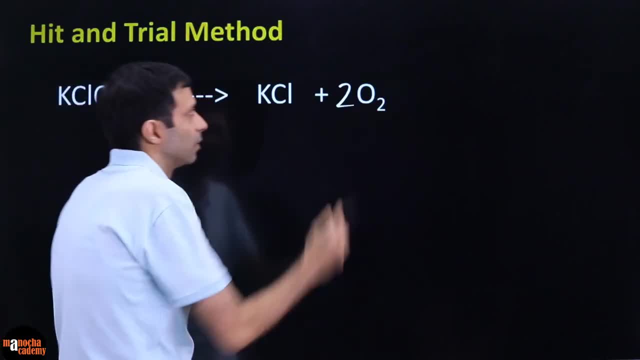 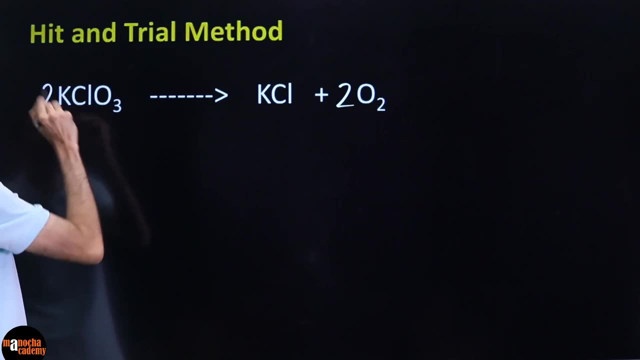 So I want to multiply. So let's say, if we multiply by 2.. So how much have we got? 4 here, But 3 here. So now it is less here. So, like the fruit and vegetable guy, We will put a 2 here. 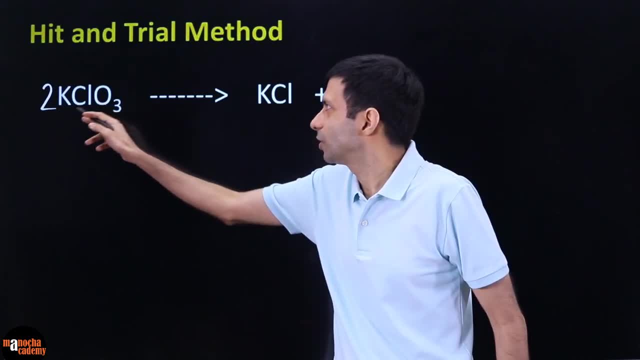 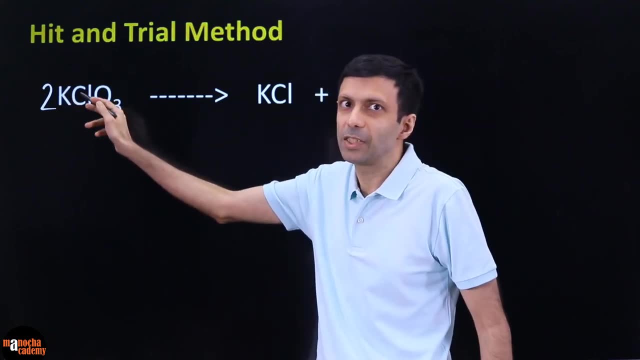 So how much does it become? It will become a 6 on that side, So oxygen becomes 6.. Here it is only 4.. But by multiplying by 2. We have disturbed potassium and chlorine. So there is 2 potassium, 2 chlorine. 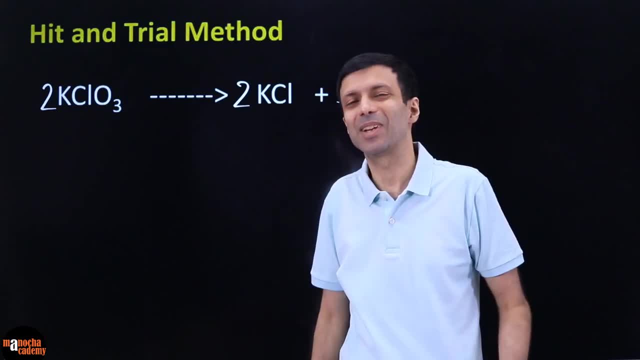 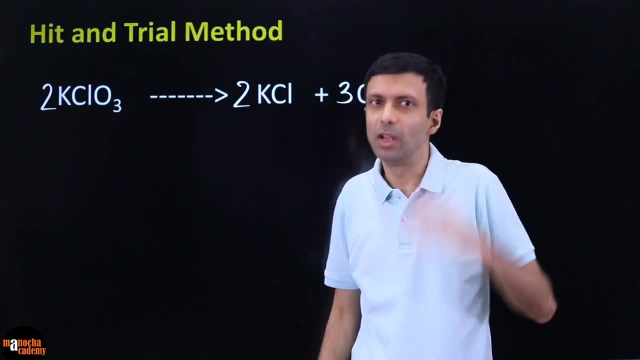 Only 1 here, So we put a 2. And there you can see it is balanced. So hit and trial is just putting the numbers. Keep on trying till you get the combination Without making the table. So you are basically doing it mentally. 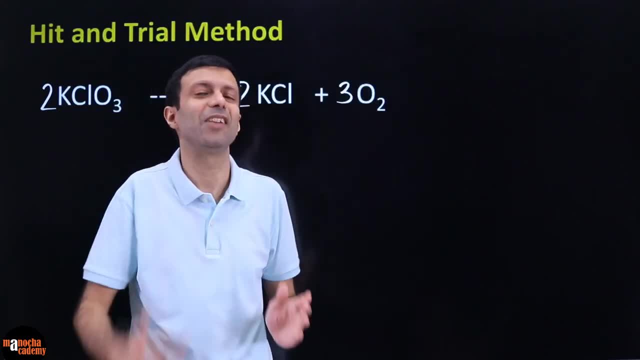 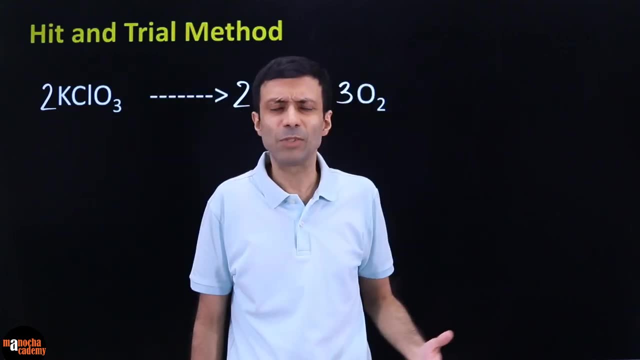 And I would recommend it Because once you are familiar with the table method, You can upgrade yourself to hit and trial, Because it is way faster. You can do it quickly. Now do you guys want to see an awesome fractions trick- How we can do this equation with fractions? 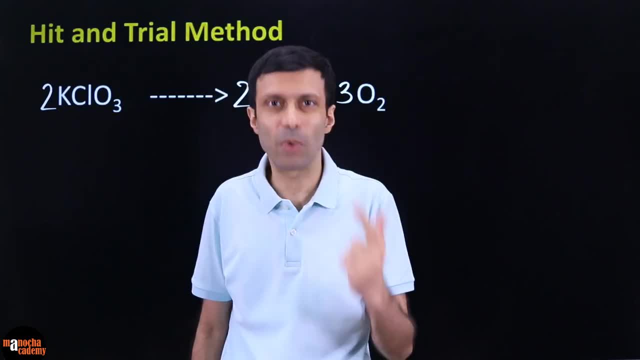 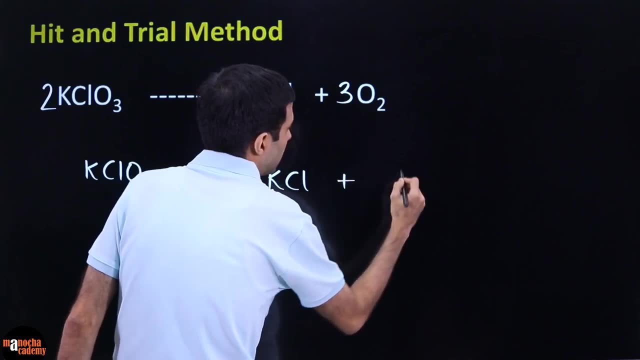 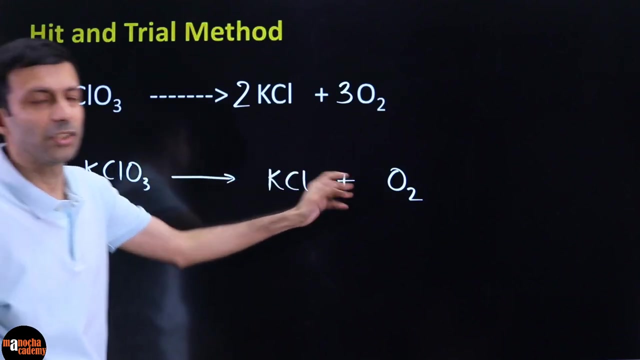 Do you want to try it out? So please write down this equation one more time. So let us write it again: KClO3 gives KCl plus oxygen. So we can see potassium was balanced, Chlorine was balanced, Only oxygen is causing the problem. 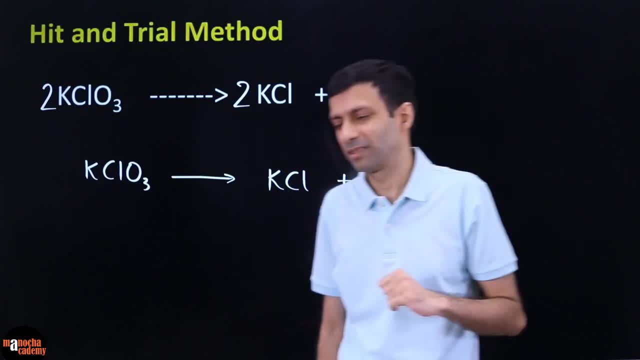 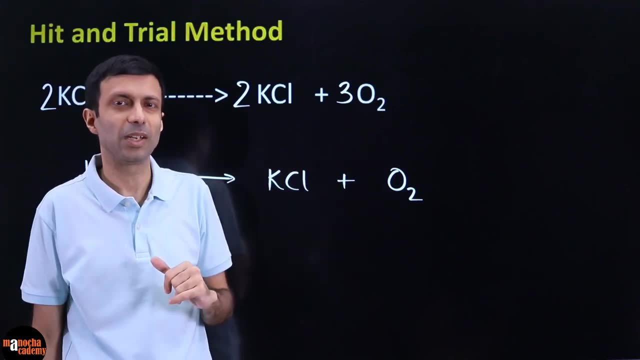 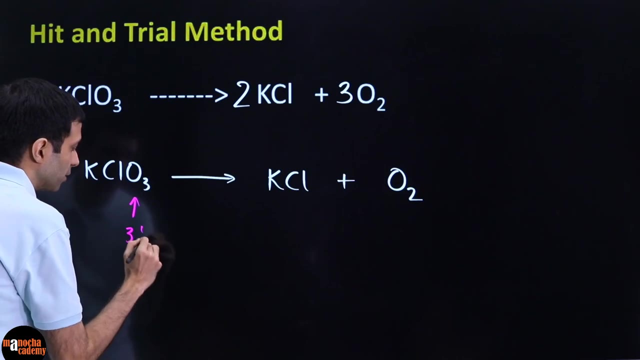 So when you have one guy left And that guy exists in different form Means alone, Then you can easily balance it using maths fractions. What do I mean by that? You can see, here We have 3 oxygens And we have 2 oxygens here. 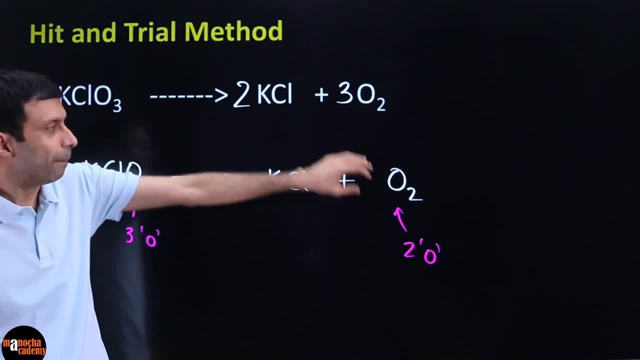 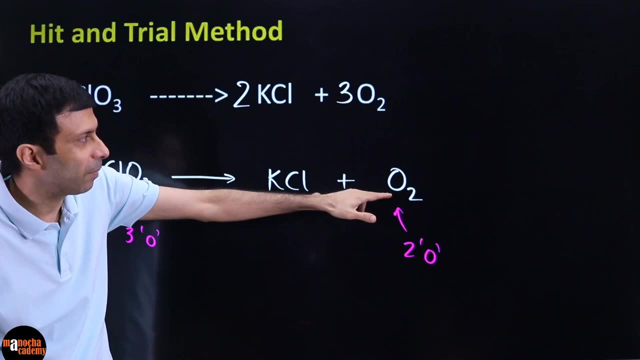 So by what number, Since it is less over here? By what number should I multiply this to get 3 oxygens? Can you tell me By what number should I multiply O2 to get 3 oxygens, If you are allowed to think in terms of fraction? 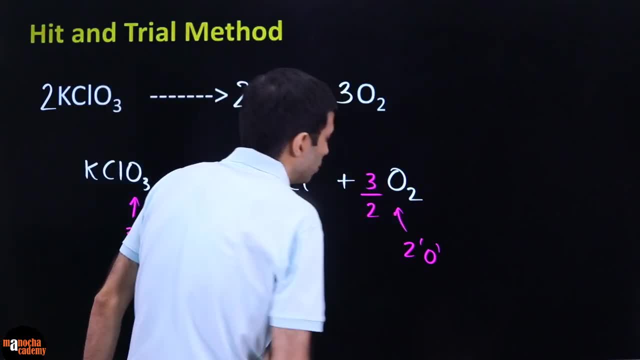 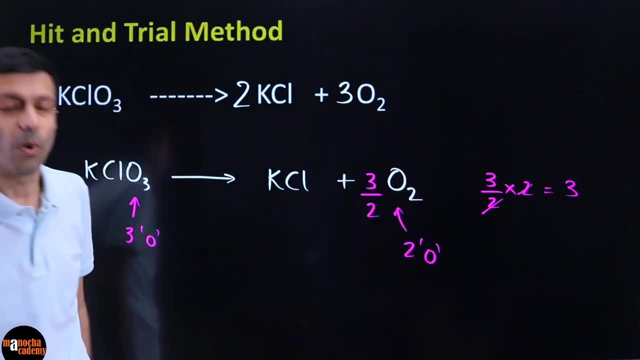 You will say: Why don't I multiply by 3 by 2?? Because, after all, 3 by 2 times 2 is 3.. 1 and a half or 3 by 2?? Yes, Here you can think about improper fractions. 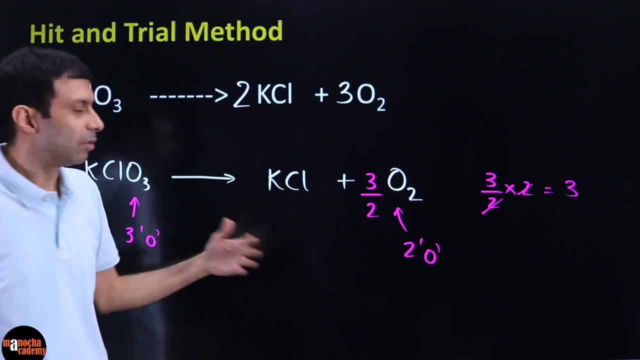 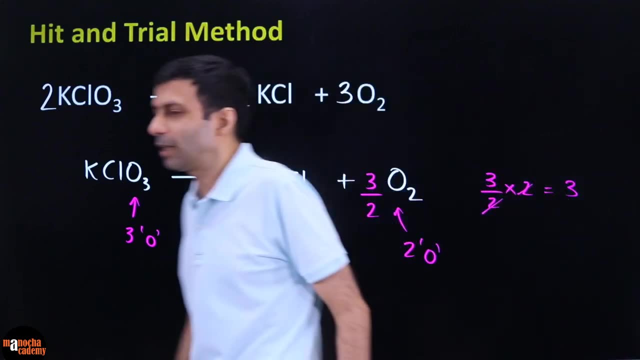 You don't have to write 1 and a half, So write 3 by 2.. So now, will you guys agree with me? Is this equation balanced? Please take a look, all of you, Because after doing this multiplication, We have 3 oxygens. 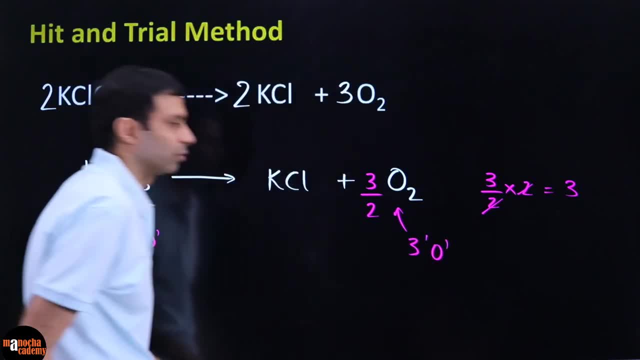 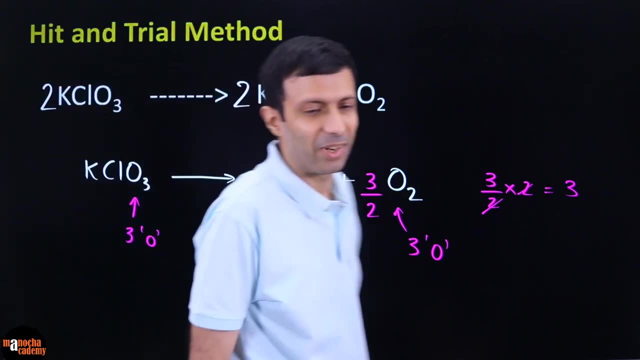 And 3 by 2 times 2, which means again 3 oxygens here. So great we are done, But are we allowed to leave fractions? No, So the chemistry teachers will get really angry if you leave the final answer as having fractions. 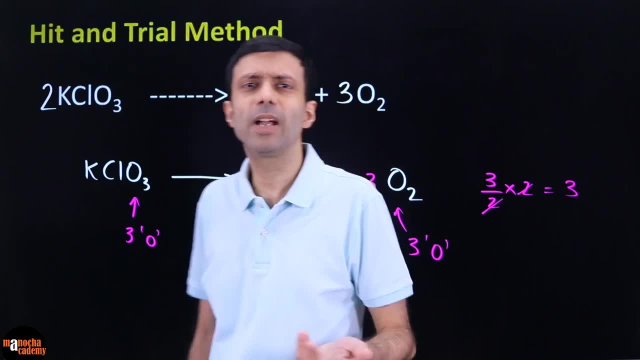 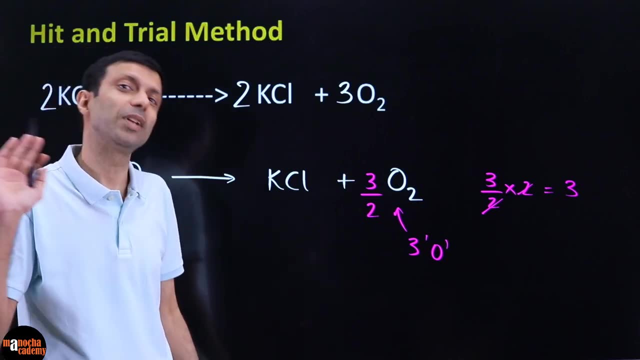 So what do you need to do? Get rid of the fraction. How do you get rid of the fraction? Because the problem is, there is a denominator. How do you get rid of the denominator? By multiplying out so that the denominator gets cancelled. 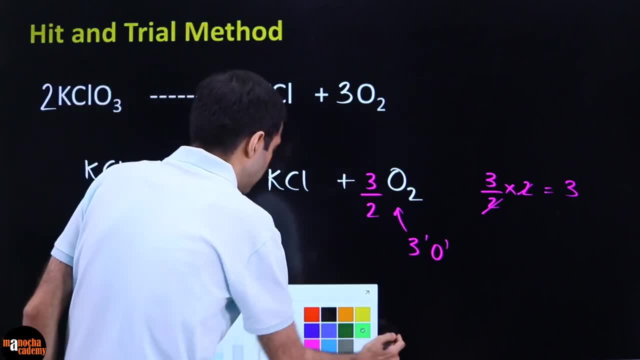 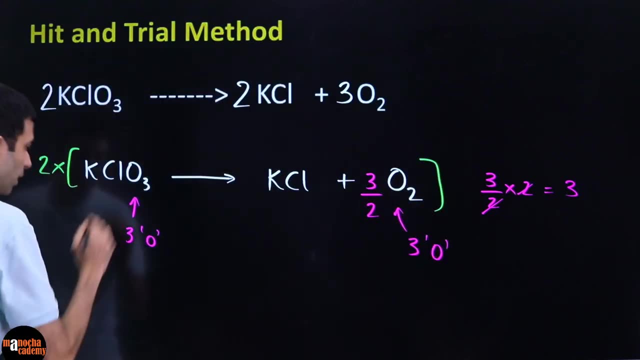 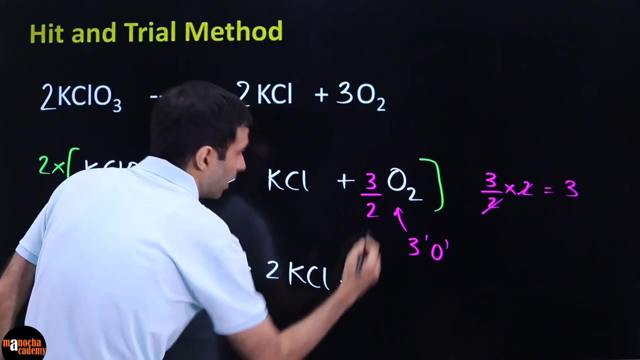 So denominator is 2.. So you multiply this entire equation by 2.. So if you multiply this entire equation by 2. You are going to get what 2KClO3 is going to give you 2KCl and 3 by 2 times 2.. 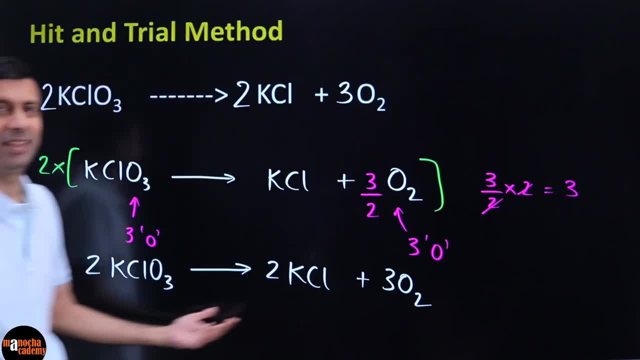 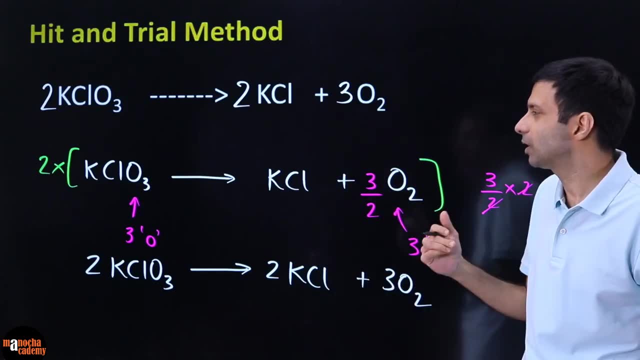 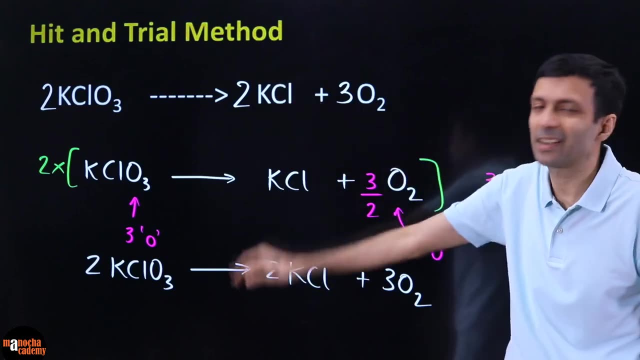 So 2 and 2 will cancel Plus 3 oxygen. There you go, We have the answer. So you can see that. whichever way you like, sometimes fractions are way faster because you can see 3 by 2 it is solved. So I just multiply by 2 and you can see we have got. 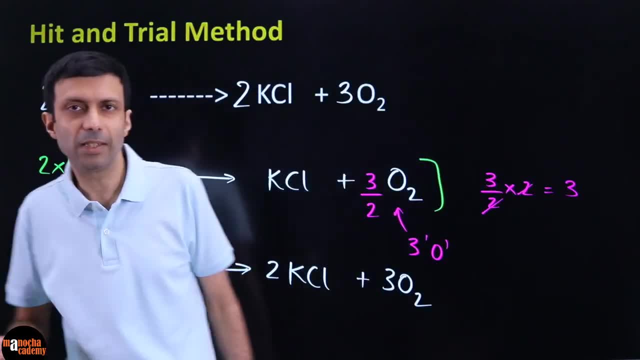 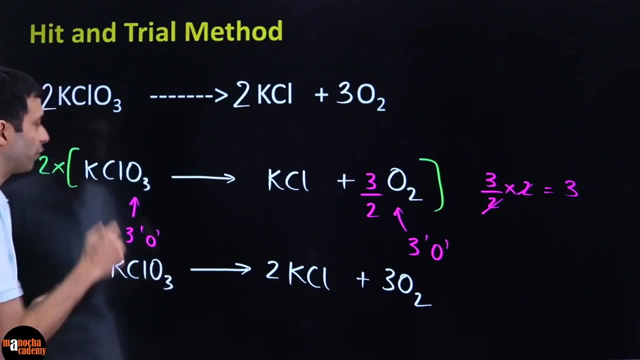 exactly the same answer Done. So this fractions method is a little more advanced method. The first method was simple, where you were being hit in trial. In this last method, why did we use fraction? Because we saw KCl is already balanced, Oxygen is 3 here. 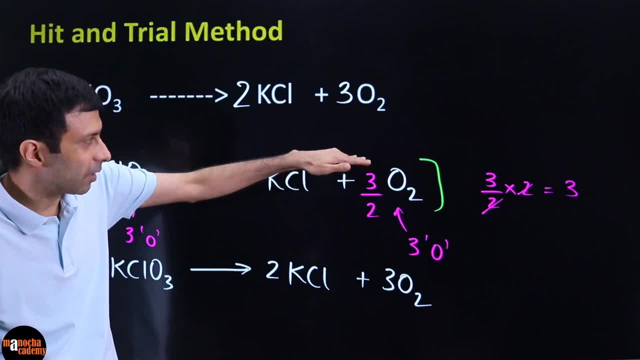 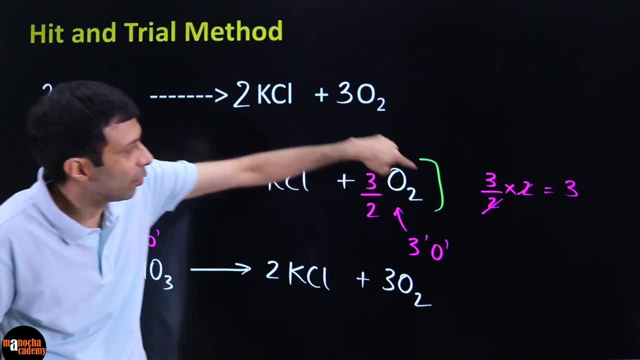 It is 2 here. So if I multiply oxygen atoms by 3, by 2. times 2. 2, 2 will cancel. So 3 oxygen over here. 3 over here. We have balanced it. But the only problem is: 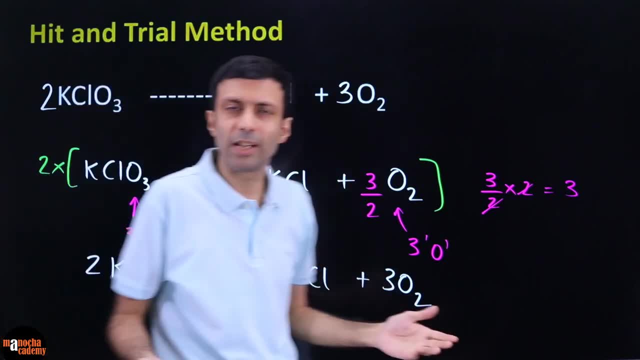 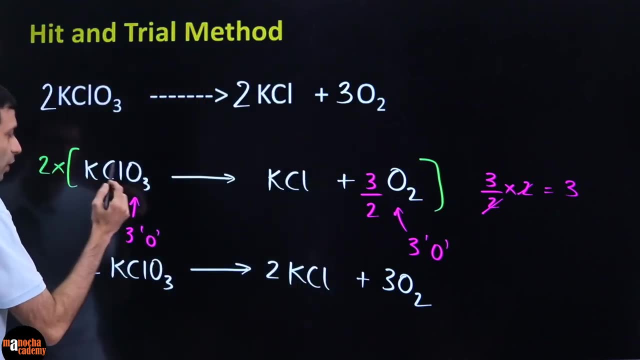 we cannot leave fractions in our final answer. So how do we get rid of the denominator of the fraction? Just multiply the whole thing by 2.. So if you multiply the entire equation by 2.. 2KClO3, 2KCl. 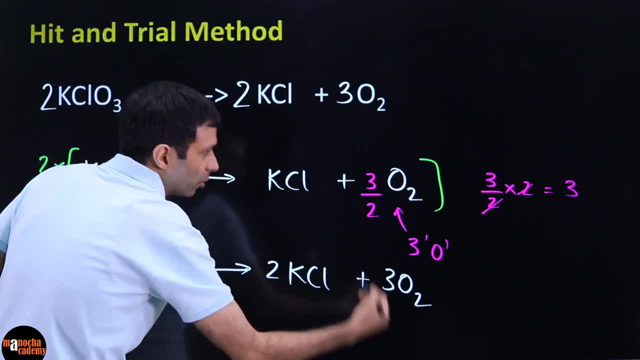 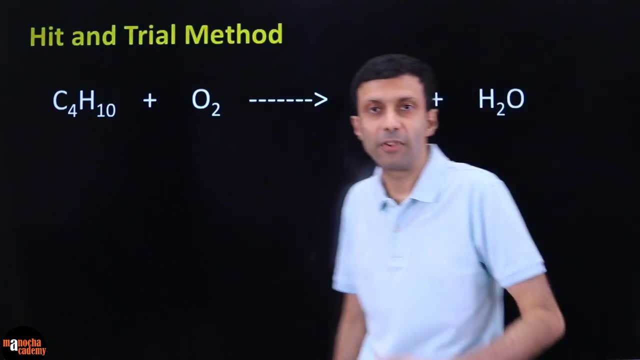 and 2 times 3 by 2.. The 2,, 2 will cancel, So 3O2.. That is the same as our last answer, Clear. So you guys go ahead and try this. You can try again. try with. 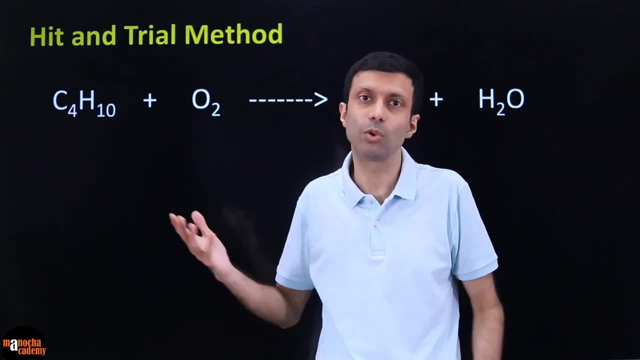 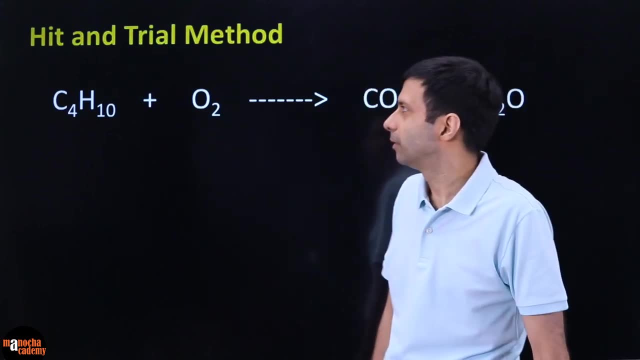 hit in trial. You can try with fractions or without fractions, I don't know Whatever works best for you. Please try this equation, all of you. So how do you do this? by hit in trial method Once again. just scan through. You can see there is. 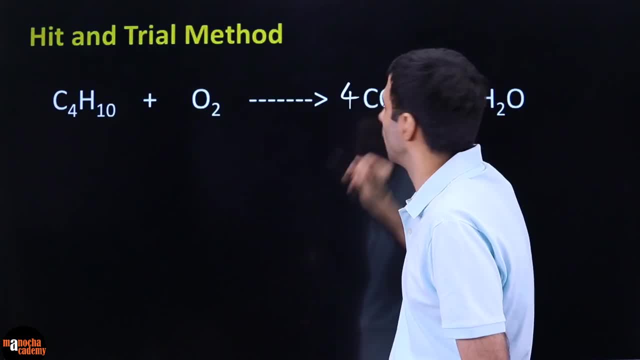 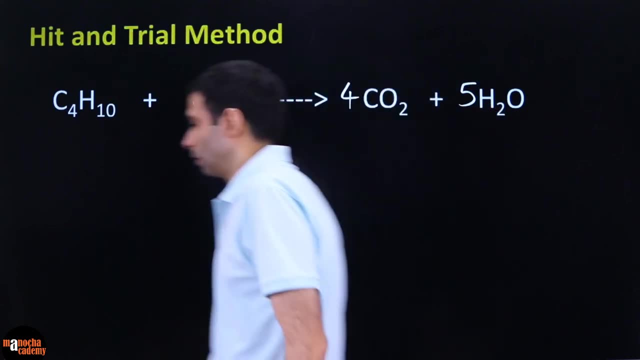 4 carbon, only 1 carbon. So let me finish the carbon 4 times. You can see. hydrogen is 10 here, Only 2 here. What if I multiplied by 5?? So can all of you see Carbon and hydrogen is done: 4 carbon. 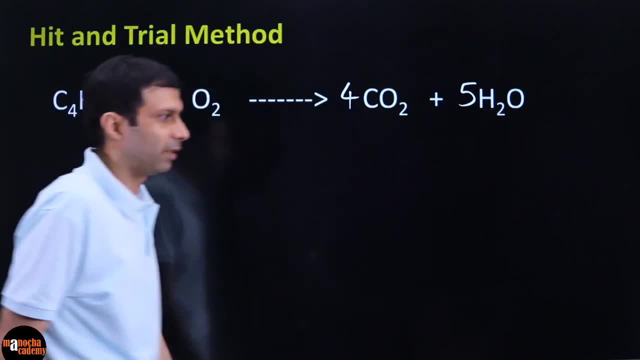 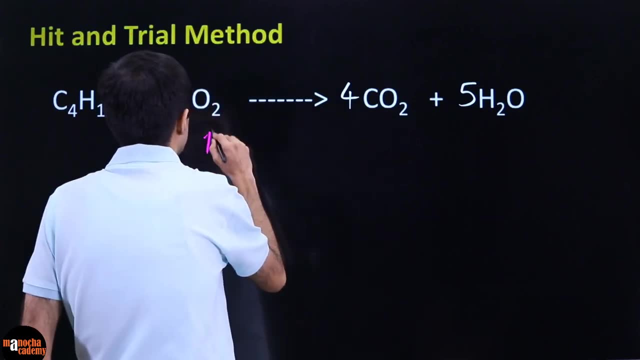 4 carbon, 10 hydrogen, 5 times 2, 10 hydrogen Done. But oxygen, how many do we have? We have 2 oxygen here, So you can see that there is 2 oxygen atoms And how many on the right side? Count carefully. 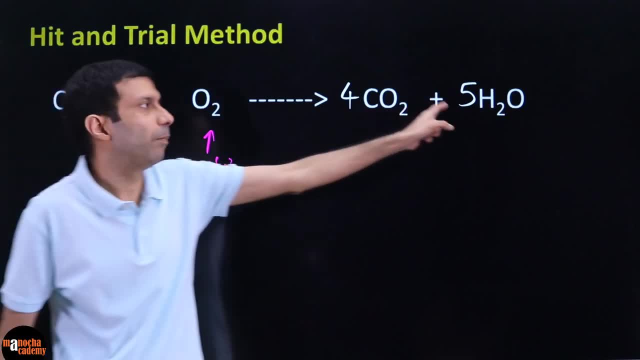 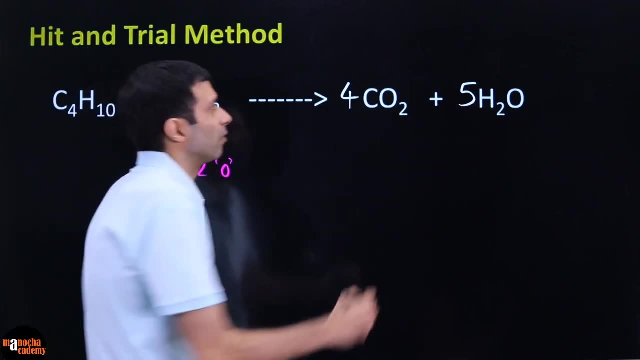 4 times 2, 8 plus 5 of the water Right, 5 times 1.. So 4 times 2,, 8 plus 5, we have 13 oxygen on the right, 8 plus 5.. Yes, 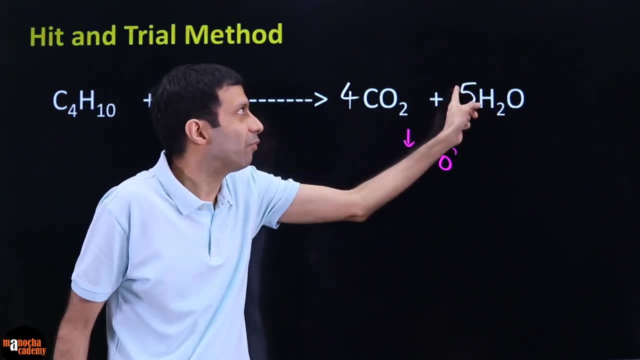 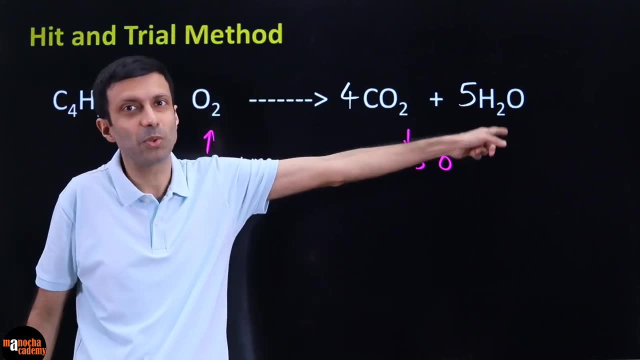 4 times 2, 8, but not 1.. 5 times 1.. Because there are 5 water Right, Each water having 1 oxygen, You understanding It's a multiplier. So 5 times 1.. 13. 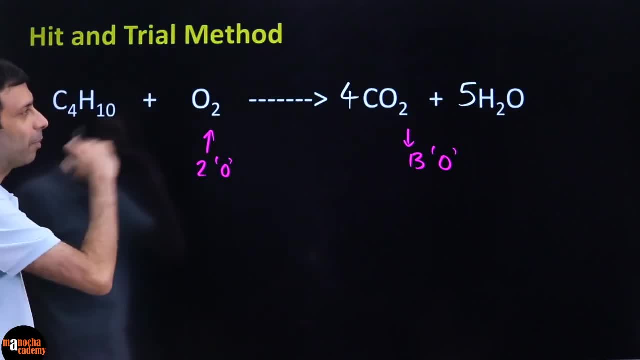 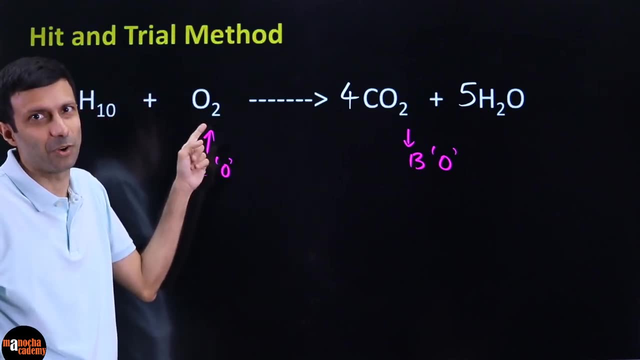 oxygen. So now, what do you do? So carbon hydrogen balance. You can see again. we have 1 element remaining, We have 1 oxygen remaining, which is luckily in the element form. So you have 2 oxygen here and 13 here. Your goal is to get 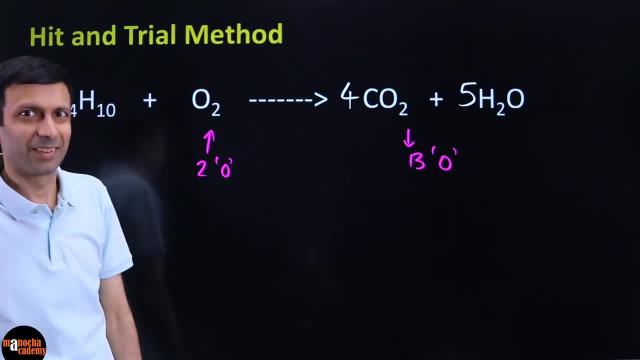 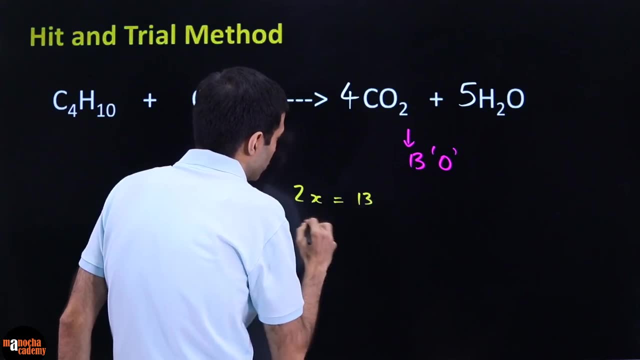 to 13.. Right, So how will you do that? It's almost like you can think of maths equation: 2 times x equals 13.. So what if I do 13 by 2.. If 13 by 2 is my multiplier? 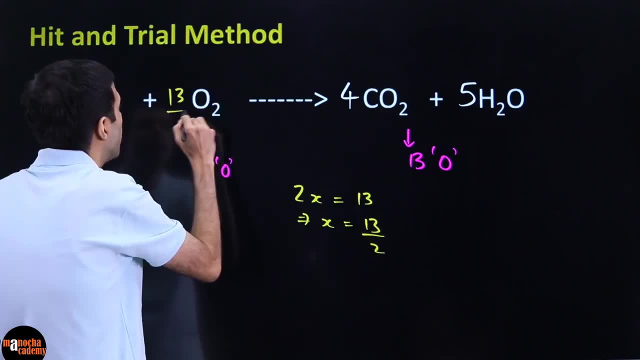 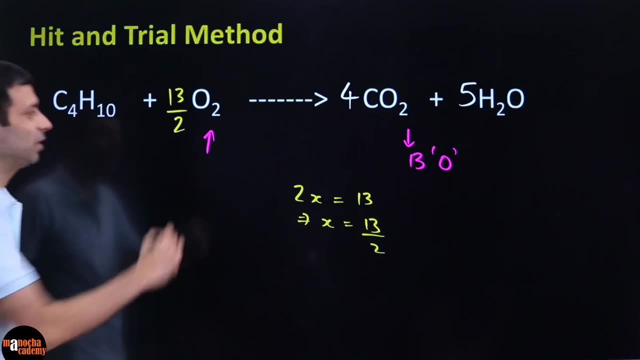 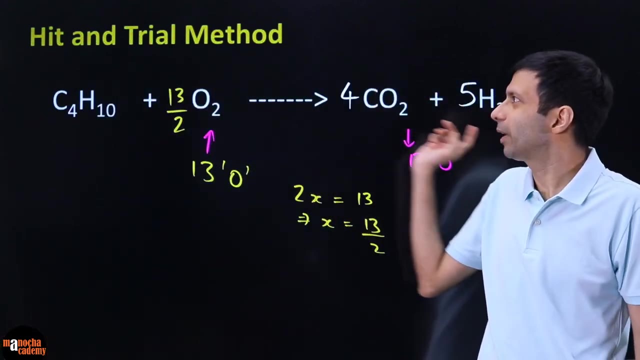 So let's say I put 13 by 2 here, Would it finish it off? 13 by 2 times 2.. 13 oxygen Done. So can you see how the fractions trick can really help us here to quickly balance the equation? And of course, the last step: 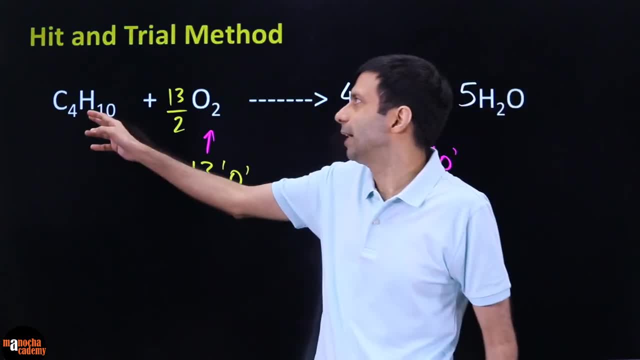 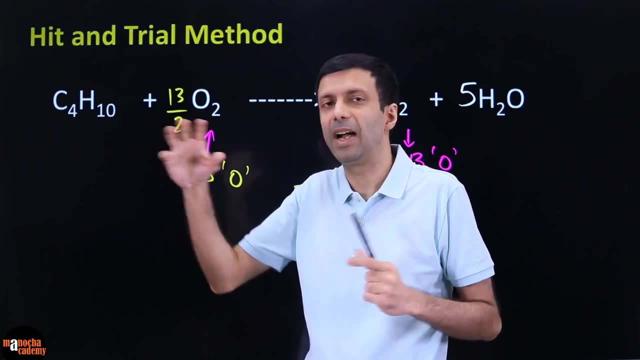 is to get rid of the fractions. So good question: Why is C4H10 not written as C2H5?? Because in this compound it is structured to have 4 carbons and 10 hydrogens. Right, If we were forming it by? 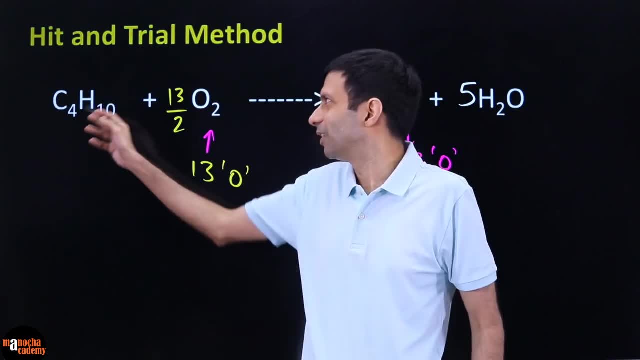 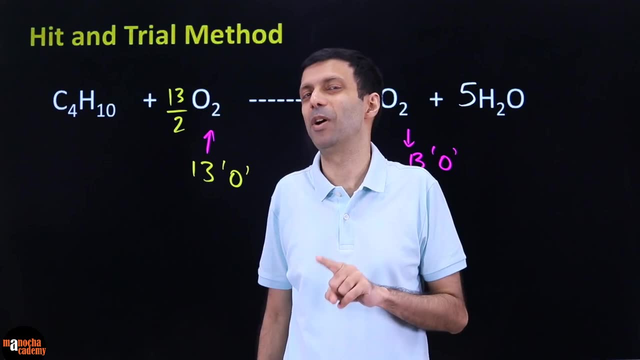 crisscross. yes, Sometimes we end up cancelling stuff. But great question here: Here we do not see any simplifying because the compound is like that. Remember, it is a crime to change compound formulas. So whatever formula is given, we have to use that. 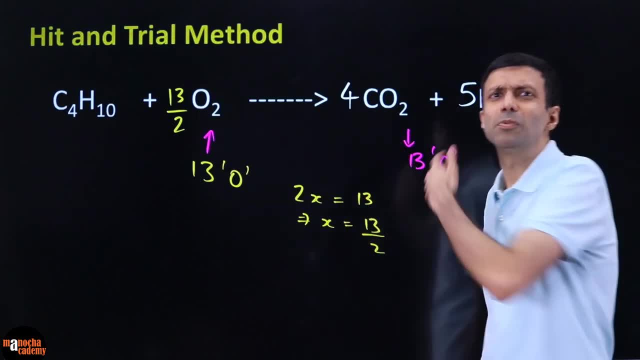 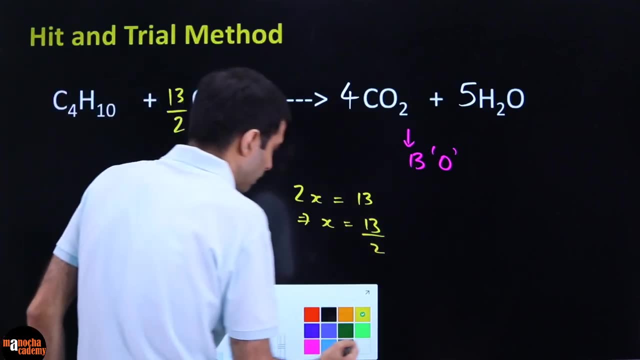 So how do you guys get rid of this 2?? Just multiply the whole equation by 2, because you have to check what are all the denominators. There is only one denominator here, So multiply this entire thing by 2.. The entire equation. 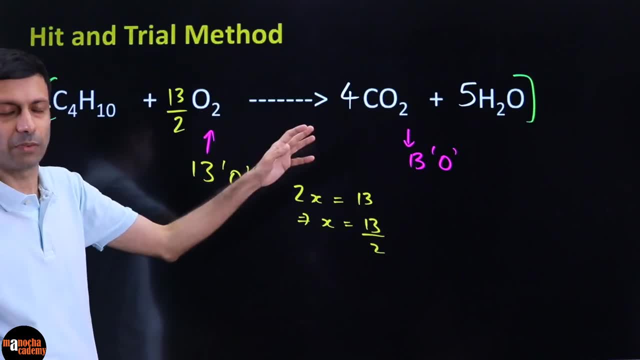 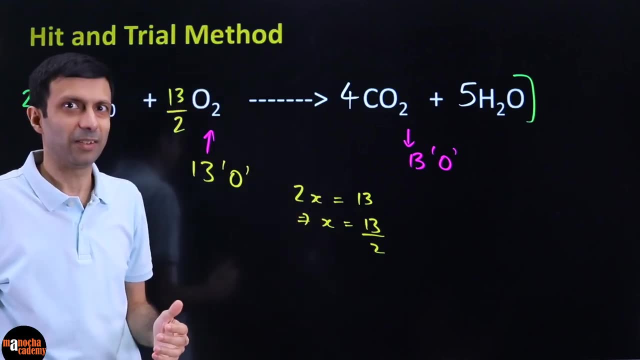 It's like in maths, right, If you multiply the entire, when you, if you have an equation, if you multiply it on both left and right hand side, the whole equation gets balanced. Right Means you are not disturbing it if you are multiplying with the same number. 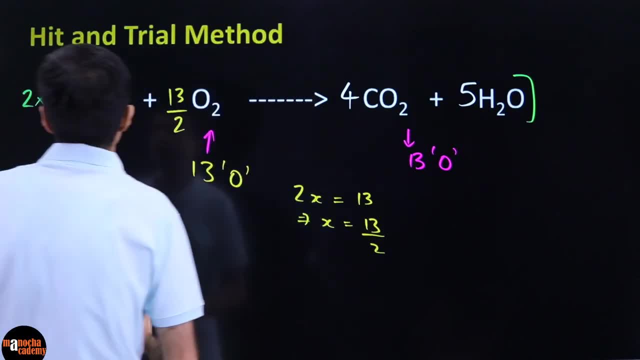 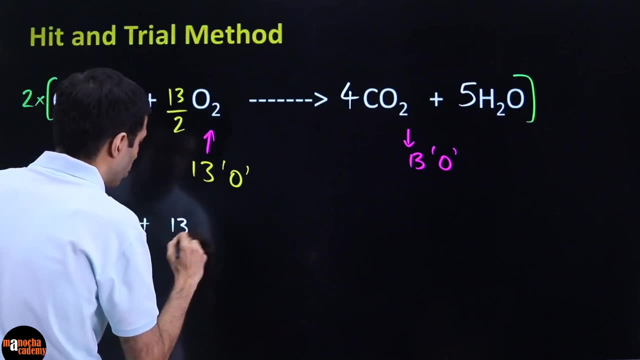 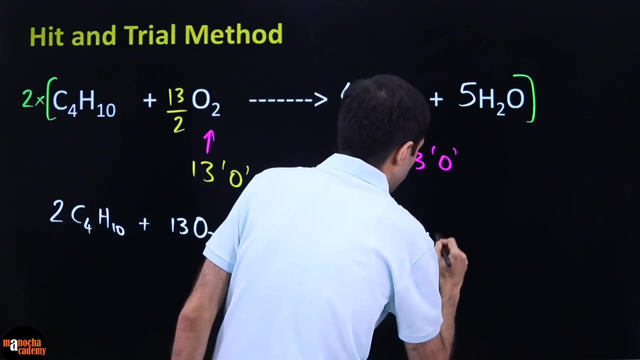 So what do we get here? So we are basically going to get 2 C4H10 13 times 2, the 2 will cancel. plus 13 O2 is going to give us 2 times 4, 8 carbon dioxide and 2 times 5. 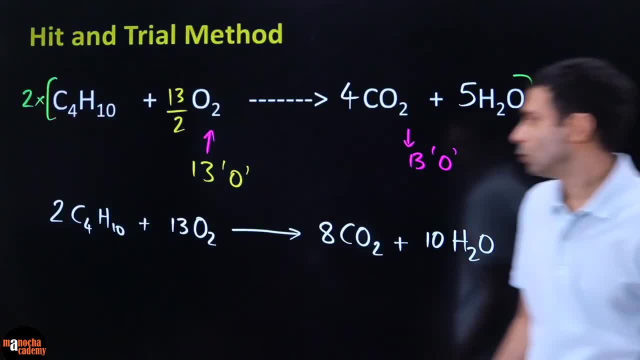 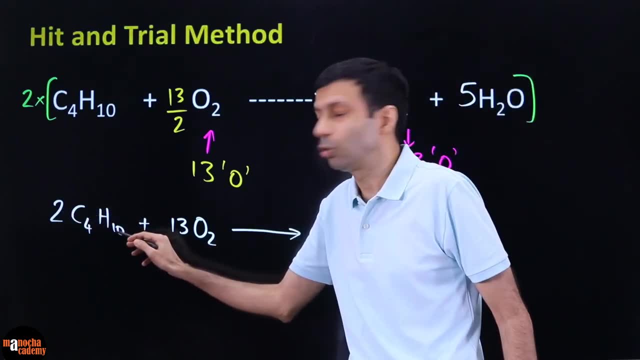 10 water. You guys can see that. So you can see there is 4 times 2, 8 carbon: 8 carbon 2 times 8, 2 times 10, 20 hydrogen: 10 times 2, 20. 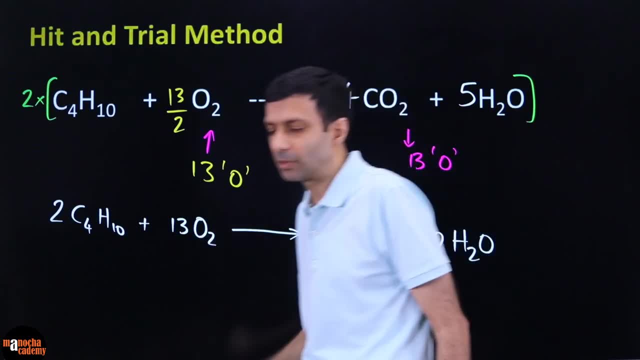 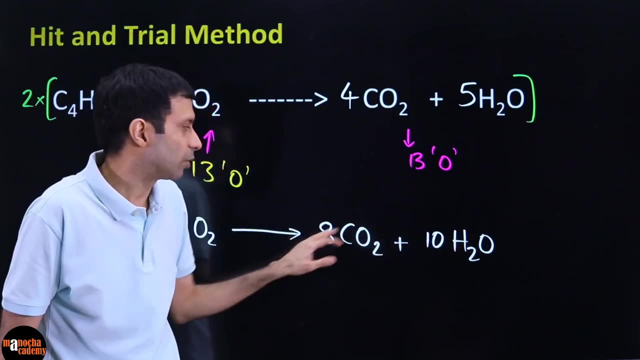 hydrogen Oxygen. how much? 13 times 2, 26. Please check over here. 8 times 2, 16 plus 10 times 1. Remember H2O1. So 16 plus 10, 26. We are balanced. 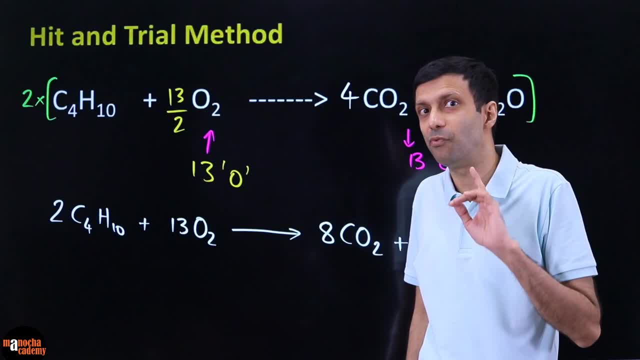 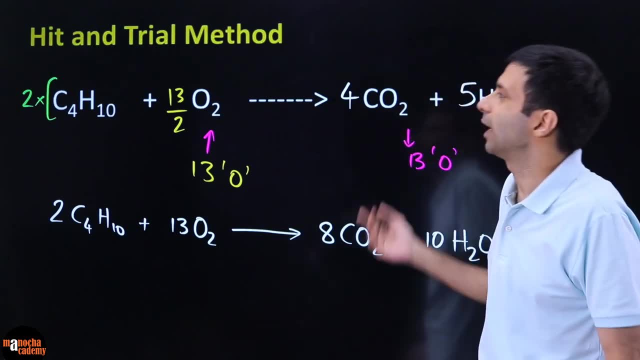 So the fractions can be really really powerful and very fast. if you have one element remaining like this, right, You could have also done it without fractions, You could have sat and you know, since you have done it till here, then you saw oxygen is less, but 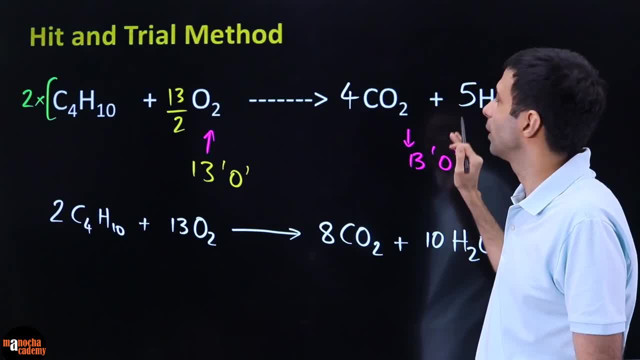 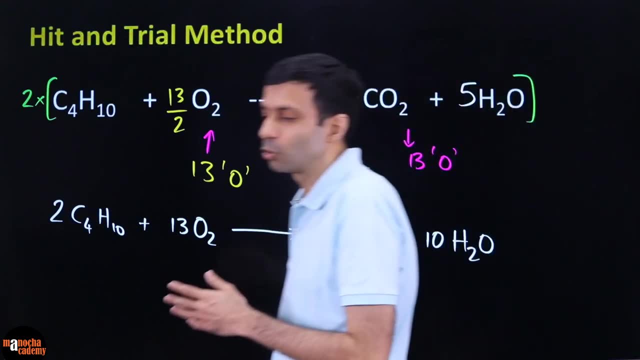 you are realizing that there is an odd even problem. There is 13 over here, So maybe you start multiplying the stuff you do 6 times you know, and try to balance it. get it close to that. That is also possible, but fractions will be. 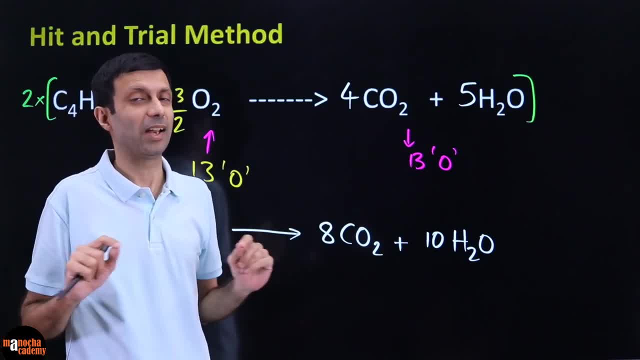 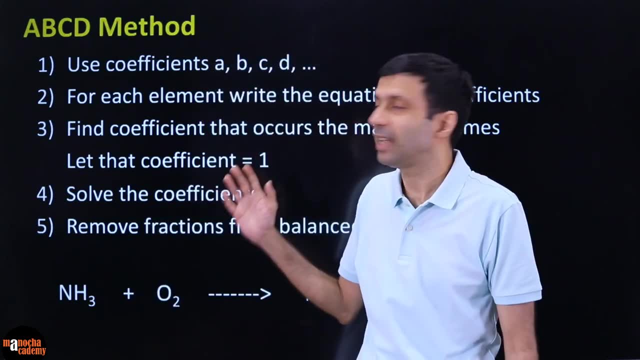 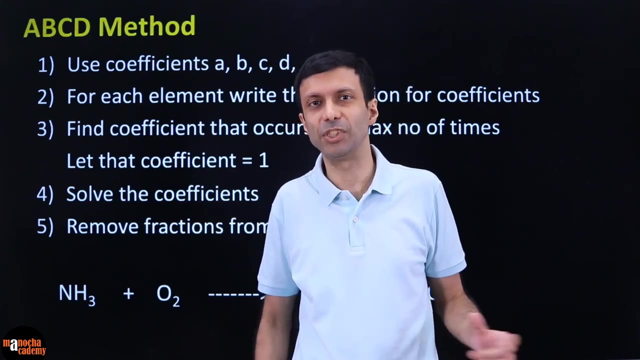 way faster. Only remember: do not leave final answer with fraction Chemistry teacher will not like that. So please practice balancing and I will be doing the ABCD method in the next class. This is a more advanced method which can help you solve more difficult balancing equations. 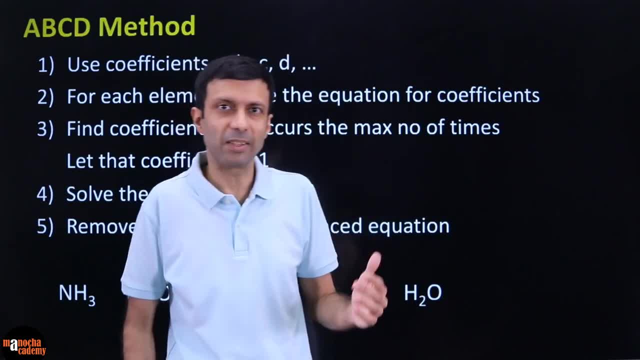 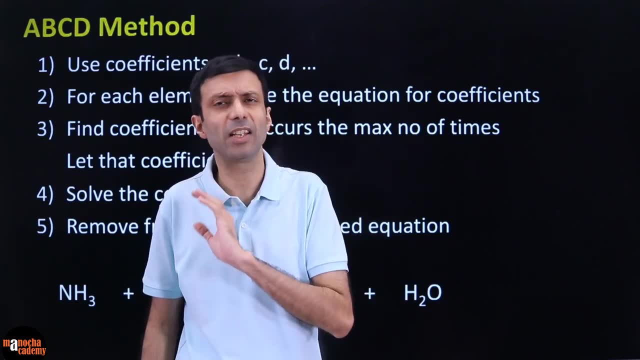 So our goal is to really balance with the easy methods like: please practice the table method first. Once you are familiar with the table method, do hidden trial method. Hidden trial is very fast. You can easily solve with that and this is the advanced one where hidden. 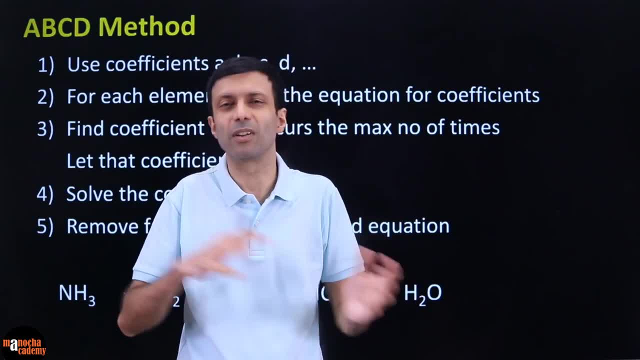 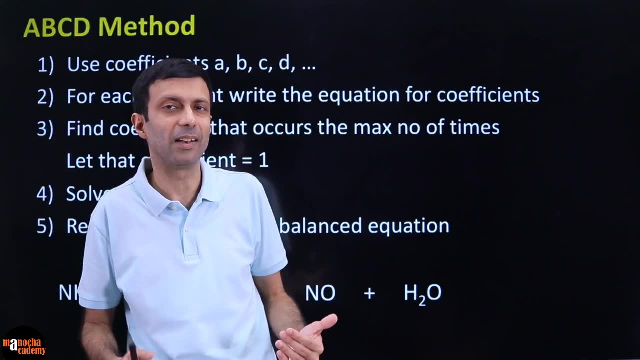 trial. sometimes you get stuck. You are sort of in a fix that you are trying a bit of hidden trial and it is not working. then this guy will rescue you out. But I will teach you this in the next class because it will take a little more time. 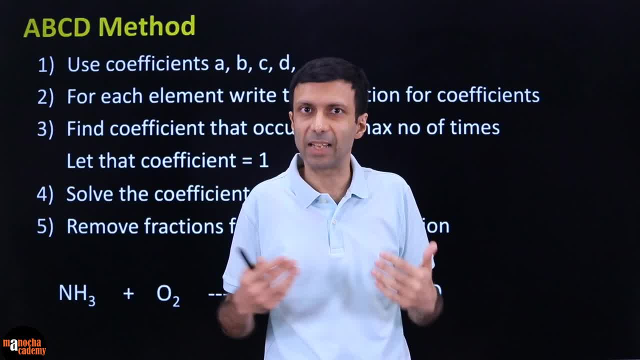 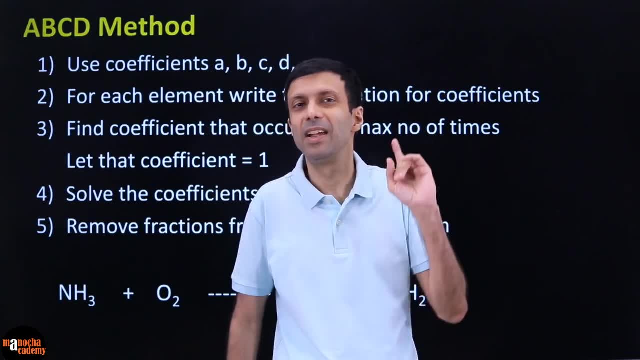 and so that I can take some doubts in this class I will open it up for doubts and we will continue this in the next class, But before that, please promise me to practice the first two methods: Table method and your hidden trial method, That is, your. 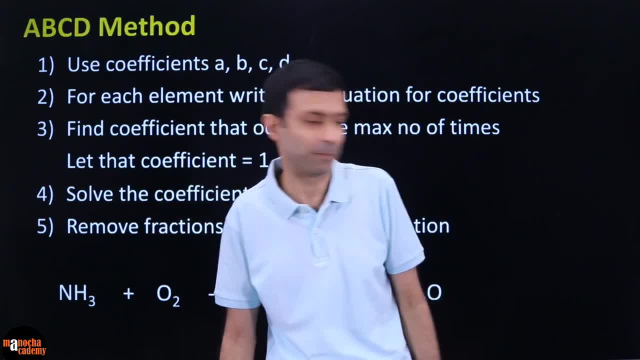 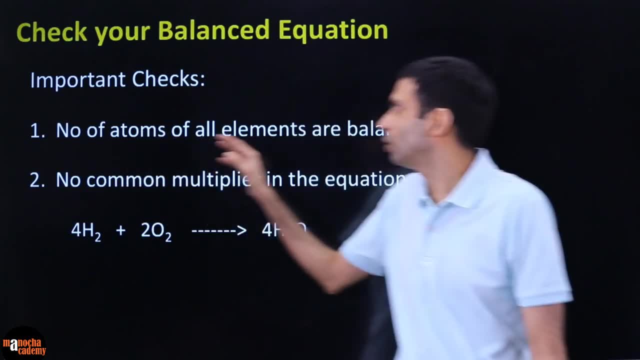 homework- This extra method I will be teaching you next time. And one important thing: when you are balancing equations, What are some important checks to do that? make sure that your number of atoms, of all the elements, are balanced Like we checked last time. Go back and check. 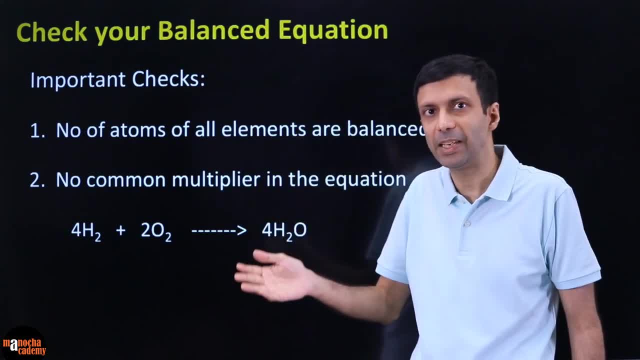 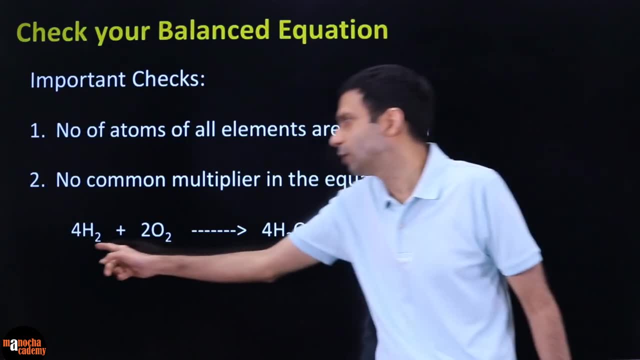 your answer because you have balanced it. You can easily check your answer by comparing each element and also make sure that there are no common multipliers in the equation. What do I mean by that? If you guys look at this equation, is it balanced? It looks. 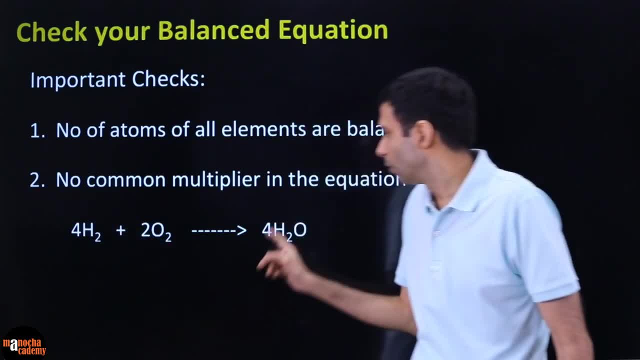 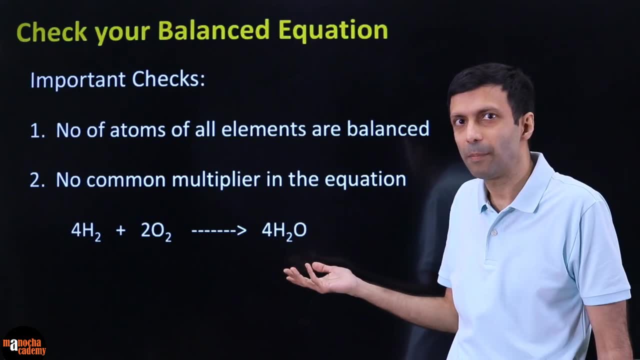 like it is balanced because you have 4 times 2, 8 hydrogen, 4 times 2, 8 hydrogen, 2 times 2, 4 oxygen, 4 oxygen. So both hydrogen and oxygen are balanced. But what is? 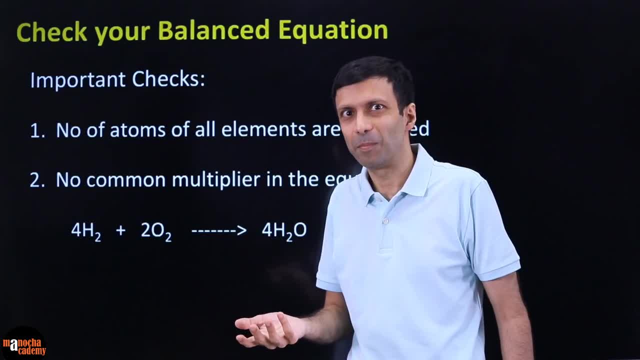 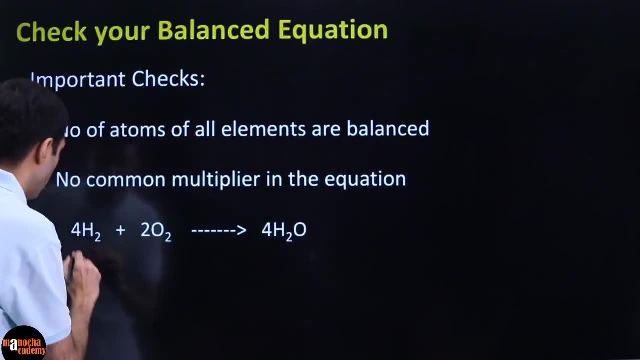 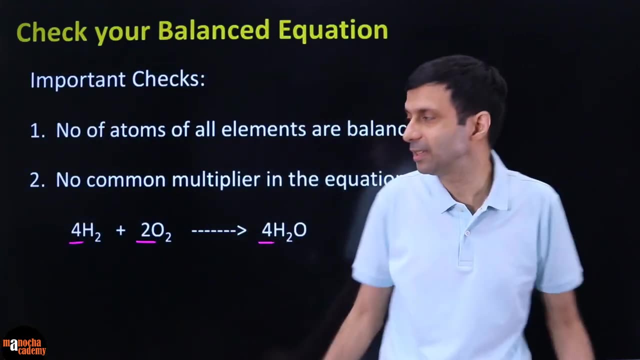 the problem. You have sort of over balanced it, Because you can see what are the coefficients here. So what are the multipliers 4, 2 and 4. Always check if they have a common factor. So after balancing, please check if there is a common factor. There is a common. 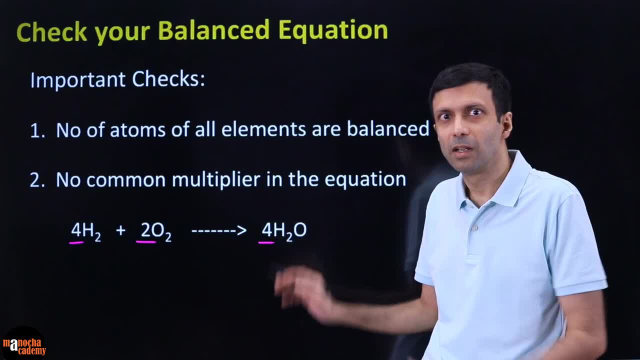 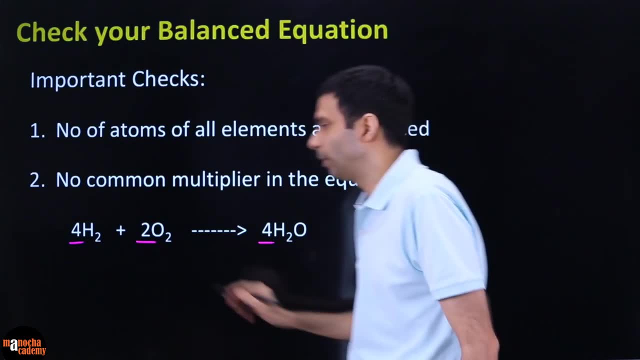 factor here: 4,, 2 and 4.. What is the common factor? If you simply divide by 2, we can see the highest common factor here is clearly 2.. So if we simply divide by 2, we will get 2H2. 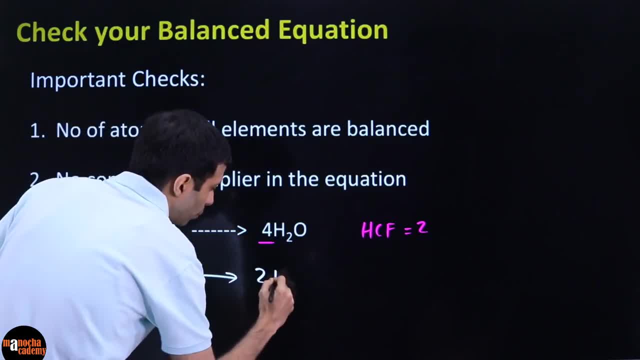 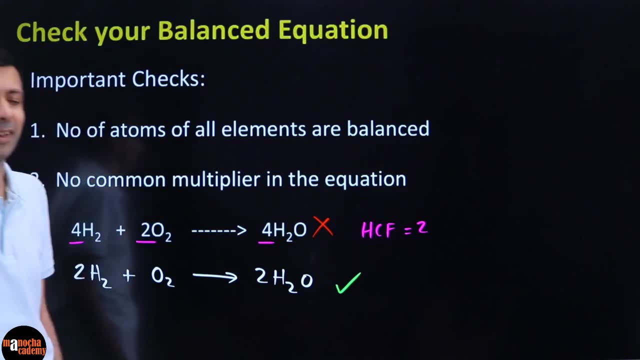 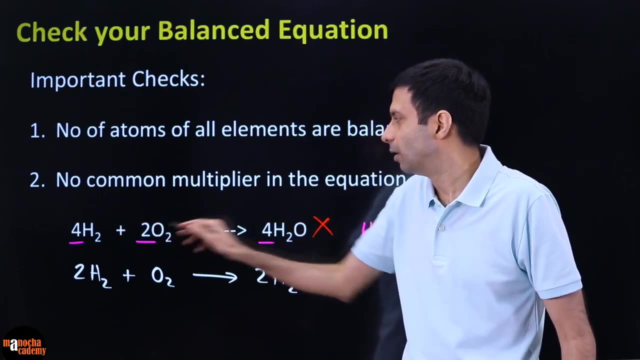 plus O2 gives 2H2.. So this will be marked correct. This will be marked wrong because you have unnecessarily generously you have multiplied which is not at all needed. So please make sure your multipliers do not have any common factor And you can easily. 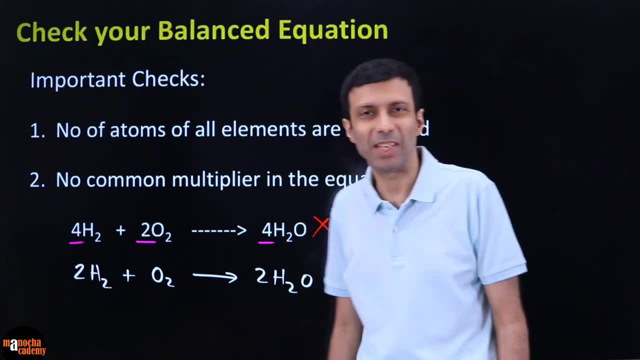 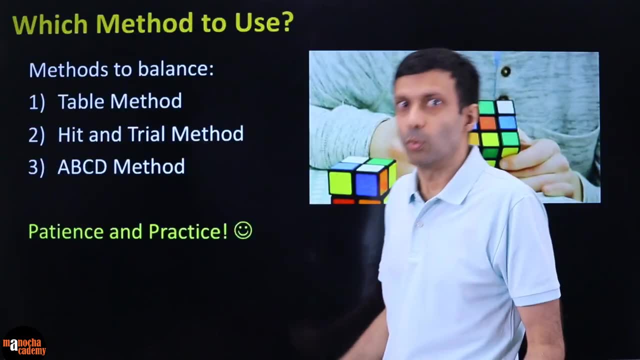 check your balancing by comparing the number of atoms of each element. So these are some very important tips to follow to make sure your balancing is perfectly right. So which method to use? Right now, you practice the basic table method. Once you are familiar with that, please try. 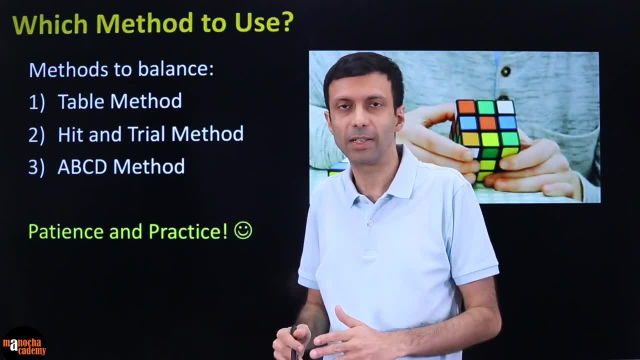 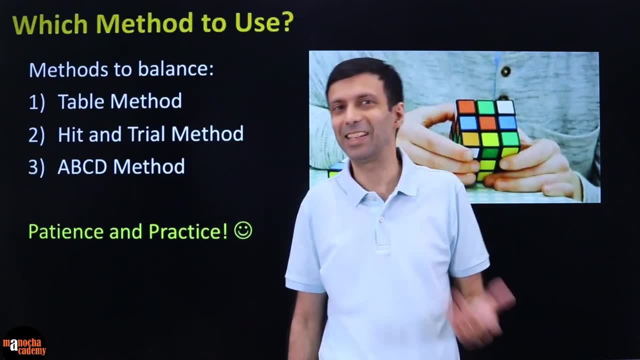 and use hit and trial. It is way faster. unless the teacher asks you to draw the table, You do not have to draw the table each time. Hit and trial is very good. ABCD is for the complicated equations and I will teach you that next time. 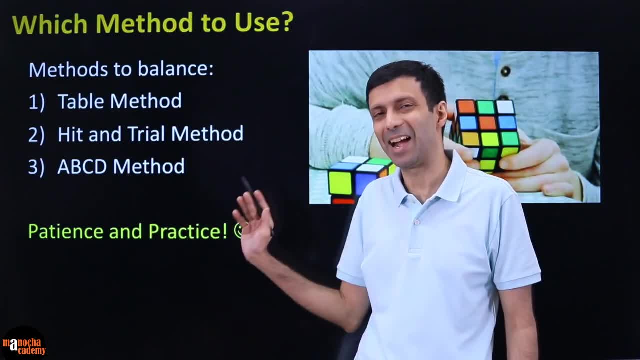 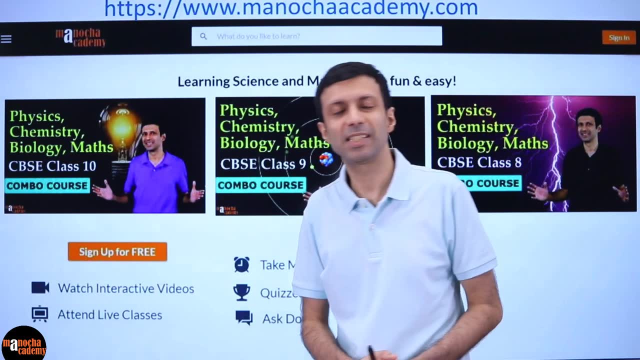 And again I am reminding you to have patience and practice. Trust me, you will get better with balancing. And do check out the other courses on our website. We have Physics, Chemistry, Biology and Maths for CBSE class 8,, 9 and 10.. 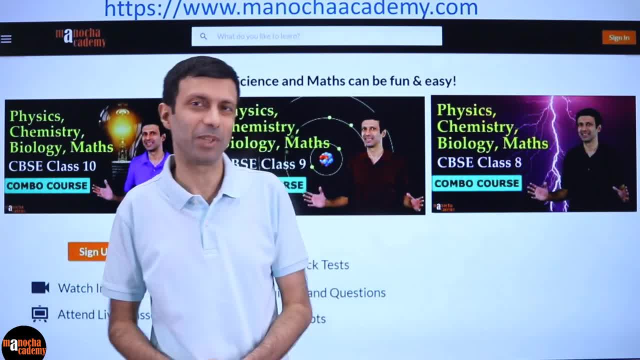 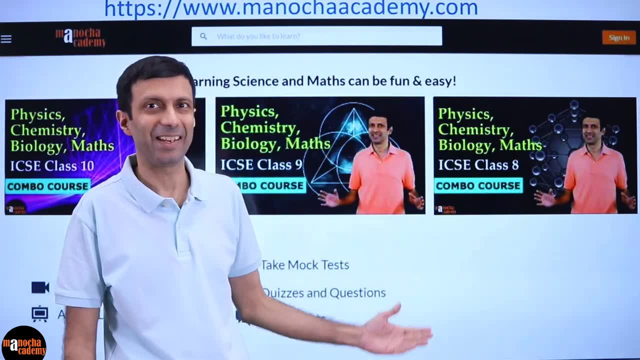 So, guys, if you haven't taken the other courses, do take them and please do share it with your friends. For the ICC students, again, we have Physics, Chemistry, Biology and Maths courses for classes 8,, 9 and 10.. And if you want to learn computer coding, we have